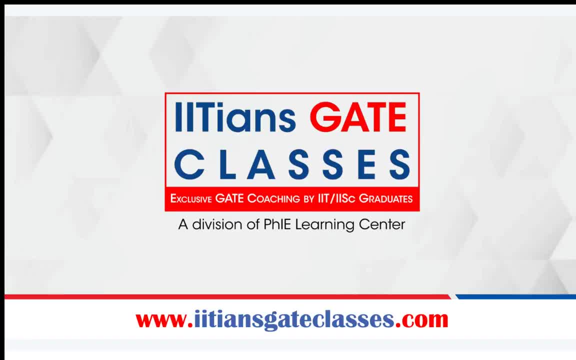 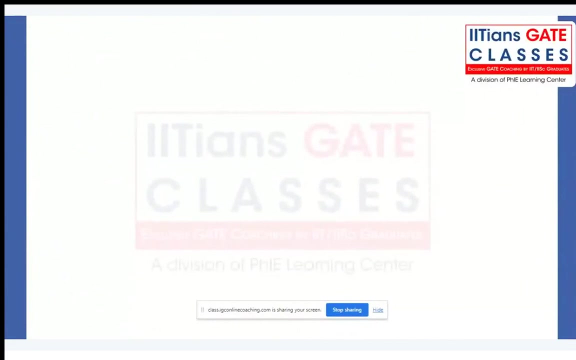 Thank you. Okay, so good evening to all of you. So we have started our discussion on Duke Dynamics and we will continue our discussion on that same. So in the last class we have discussed about the streamline, not on the stream. 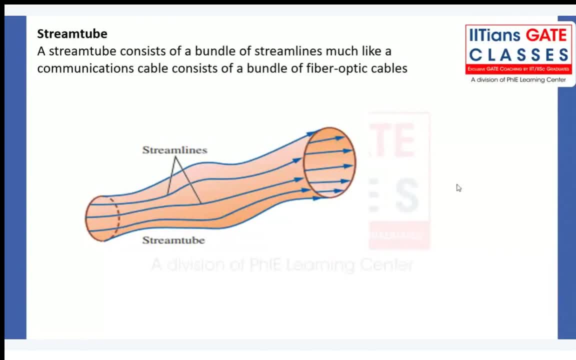 tube, The stream tube. basically, when you combine many streamlines together, they will make a tube like structure and that is nothing but the stream tube, A bundle, just like a cable wire. you know, when you open the cable wire, a very 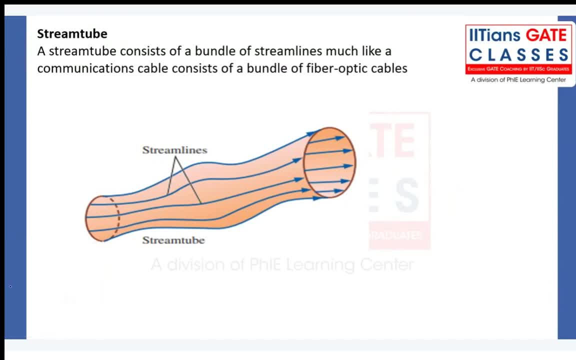 thin cable wire. when you open it, you will find in that what you will find. You will find in that so many, it consists of so many thin, thin wires. you know So, just like a one streamline, what we have when you combine. 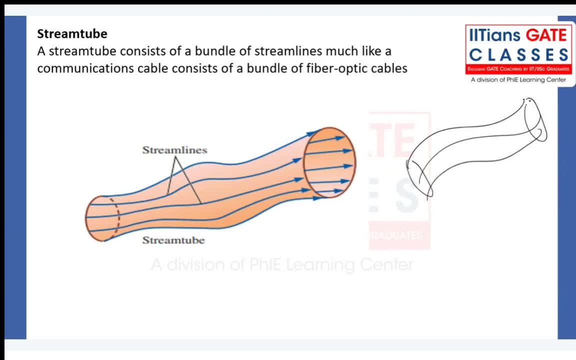 multiple streamlines you can form a tube and that tube is called the stream tube right, Just much like a communication cable wire. It happens right. In reality we do have a stream tube kind of a structure right Whenever the flow is happening in a let's. 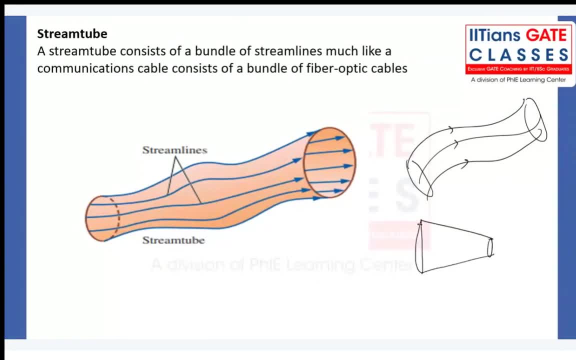 say a nozzle. So it will be like this, only It consists of multiple what we call, you know, streamlines. In a 3D figure you try to visualize, not in a 2D figure, In a 3D figure it will be there, complete. 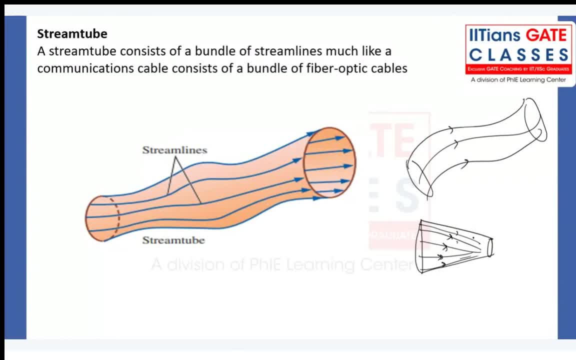 Picture of streamlines. you know, And when you just make the tube by combining all this streamline you will find one stream tube structure Not that much important. but to have the clarity we have to note down So you can see, you can see, you can see. 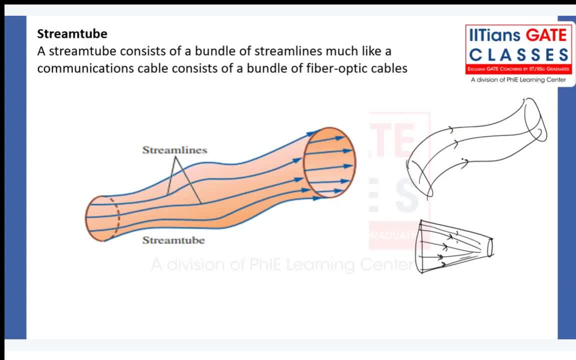 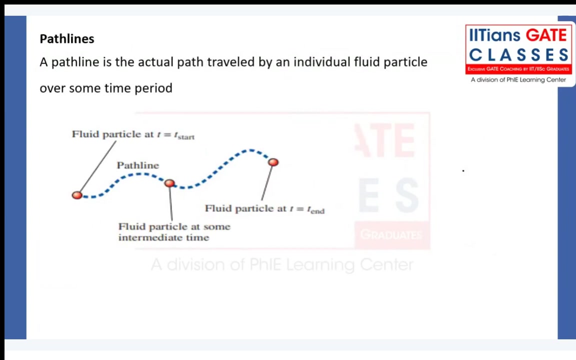 if a stream line, is you not on the next hotline, you, you. so pathline is nothing but the actual path which is being traveled by individual fluid particle over some time period. so 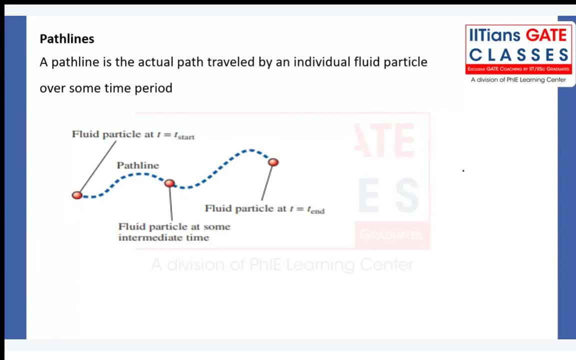 pathline is an actual path which is being traveled by individual fluid particle over some time period. we call that to be a pathline, just like a. you know, fluid particles is there which is being traveling, so right. so, whatever the history of the particle is there that can be measured. 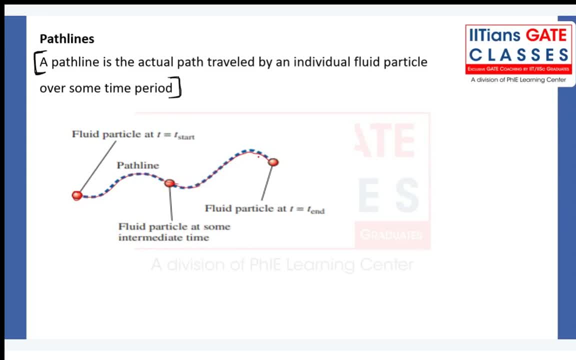 that can be. we can see through this pathline. so what we can write, it is based on the Lagrangian approach. it is based on Lagrangian approach. so I am going to show you how to write a pathline. that is the first thing. second thing: 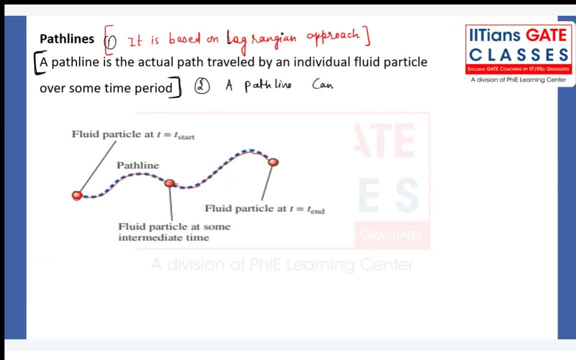 a pathline can intersect itself. whatever the pathline is there that they can. single particle is there, you know it can basically cross itself right. pathline is for single fluid particle, for single fluid particle. all of you have noted them. all of you have noted them. so the history starts from here. 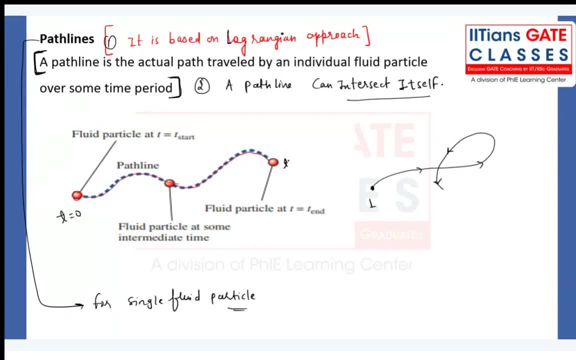 so the history starts from here. so the history starts from here, from time t equal to zero to time t equal to capital T. once it is done, let me know. so, apart from this streamline and path line, we do have one more line, that is a streak line. 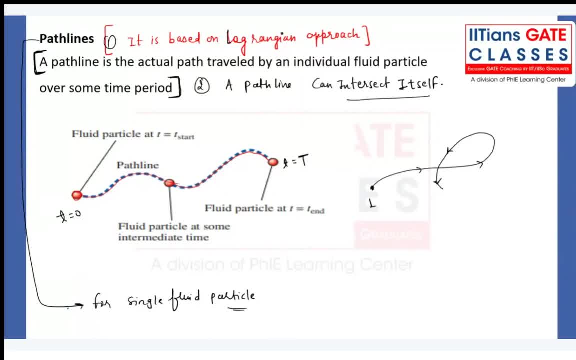 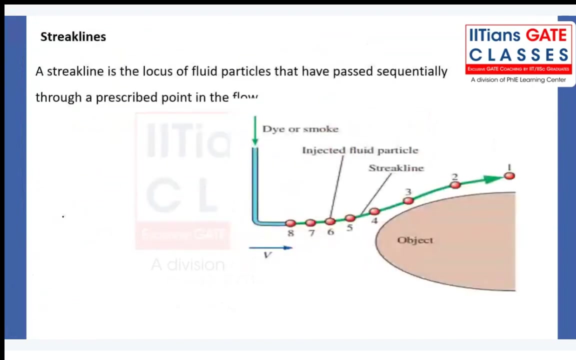 and that is a very important Done. please, no doubt, and please join the class on time guys, especially in my class. I need to tell a lot of things, so definitely I need some more than two hours always Done now. note on this streak line: 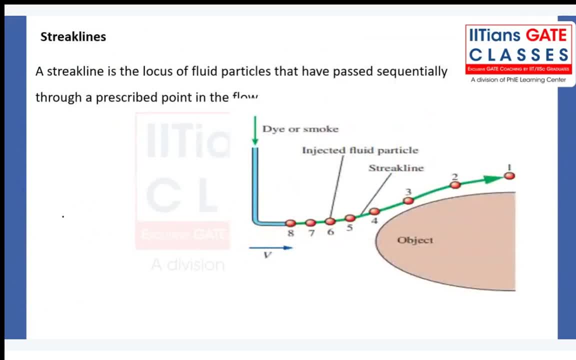 A streak line is a locus of fluid particles. a streak line is a locus of fluid particles. a streak line is a locus of fluid particles that have passed sequentially through a prescribed point in the flow field. Now do not make this diagram. I will explain you this diagram after some time. 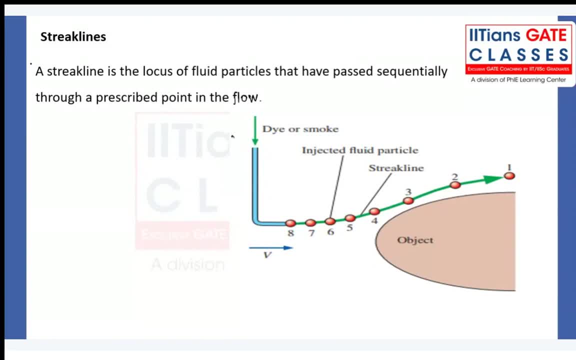 Let me explain through one another example. So you first note down from here to here only only the definition of streak line. It is a locus of fluid particles at an instant which have crossed through the same point. Now, so let me explain that, then I will get back to the definition as well as what you 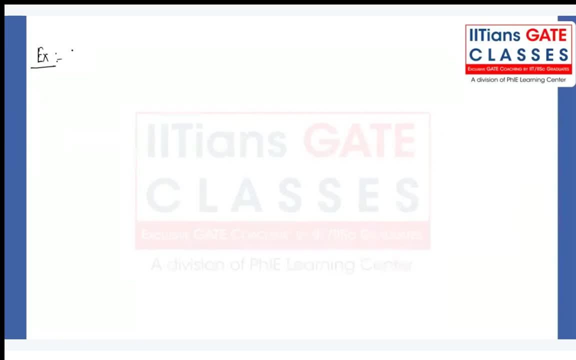 call. So let me just say, the nozzle is there or may be, some dye injector is there which injecting some kind of bubbles or fluid particles you can consider. let us say that the bubble sequence is one, two, three, four. one, two, three, four, So four particle. I have considered right, hypothetically you have to imagine, as there are infinite number. 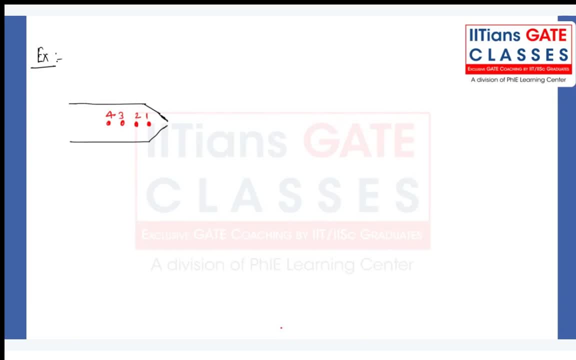 of particles are there. For the sake of simplicity, I am considering only four particles. Now, in this four particles, what I have to do? the very first thing that we have to think about. the part line, Let us say the part line of the particle number one is something like this part line of first: 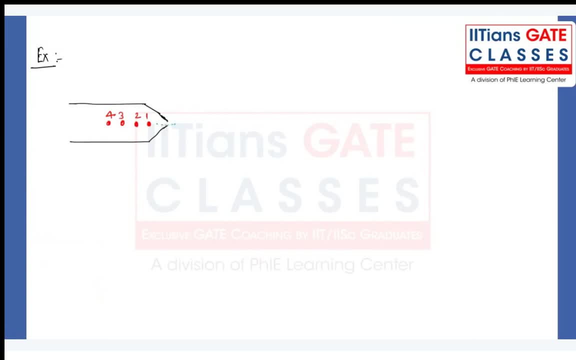 particle which is being injected, it is injecting, injecting and it is traveling. let us say it is traveling like this. This is a part line of first particle. After injecting from the point P, let us say the particle one is traveling along this line. that is a part line one. 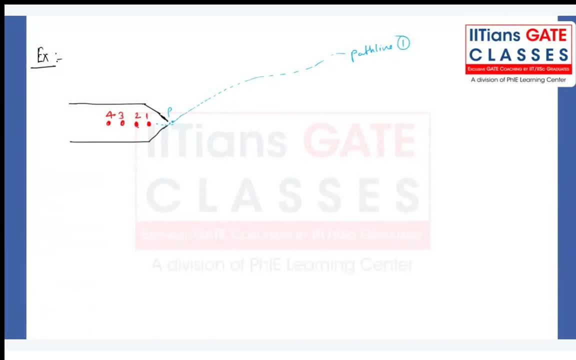 After some point of time, point particle number two will also be injected through the point P and let us say it has traveled a distance like this: this is a part line of second particle, Part Line of third particle, Part line of third particle. let us say something like this: 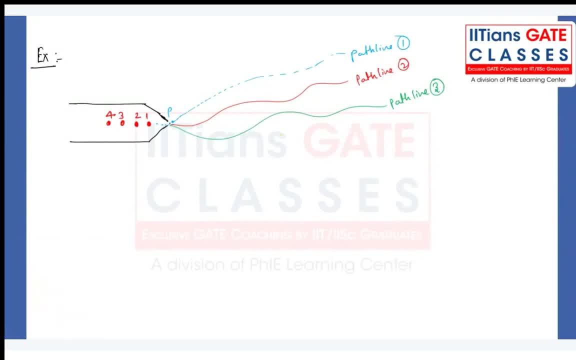 Part line of the third particle, let us say something like this: and the part line for the fourth particle is like this: because we never know right, it is a unsteady flow. I am talking about unsteady flow and in unsteady flow, you know, it is not necessary that every 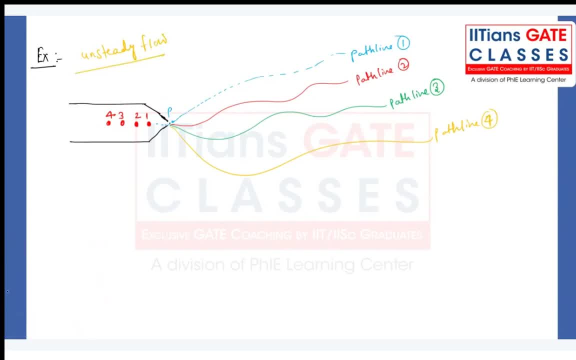 fluid particle will follow the Hello hello. I am audible. all of you can hear me. is that any breaking is there in the voice? can you please check? I will say So. the part line of the fourth particle. we will be having something like this, you know. 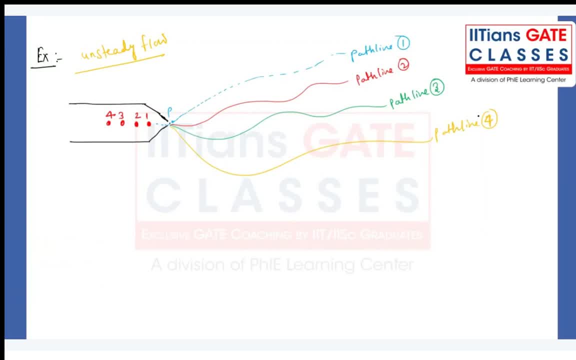 as it is unsteady flow, so we cannot guarantee that every we cannot guarantee that every particle will follow the same path. they can follow some other path. you know, every fluid particle can travel with some different velocity right now, and velocity is having both magnitude as well as directions. 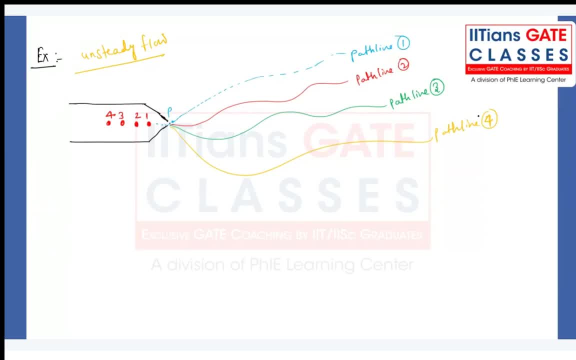 Now you understand What is the meaning of part line. let us say at time t equal to capital T. second, I want to locate my particle number one. two, three, four. where is my particle one? let us say time t equal to t, starting from zero. second, my particle one is here, somewhere here. particle. 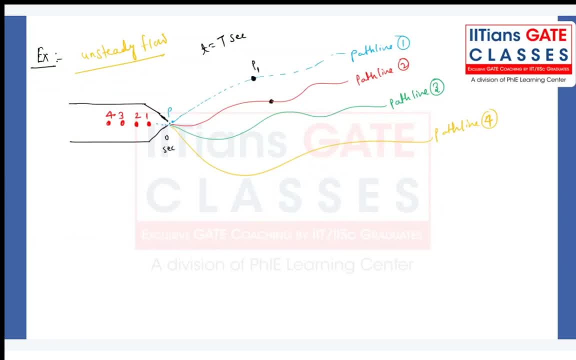 one. let us say, my particle number two is here at time, t equal to t, only capital T, and my particle three is here and my particle four is here, Part Line. So I have drawn, I have just pinpointed the look, basically location of a particle at time. 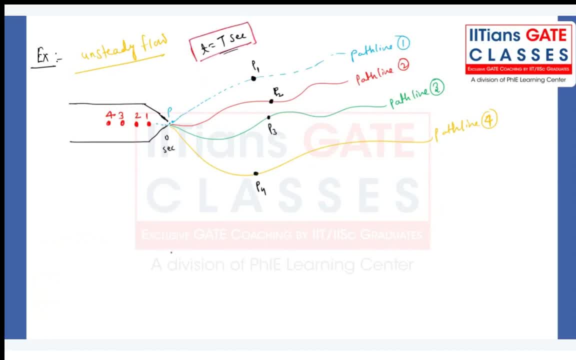 all the particle at time, t equal to capital T. second. what I will do, I will join all this locus of points through one line, something like this, and I will connect this line from the starting point. So this is my streak line: at small, t equal to capital T. second. 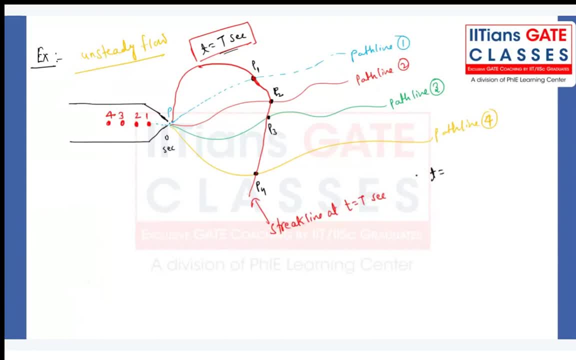 Let's say I want to calculate, I want to see my streak line at time t equal to 2 t second. So let's say the particle number one is here, particle two is here, particle three is here, particle four is here. 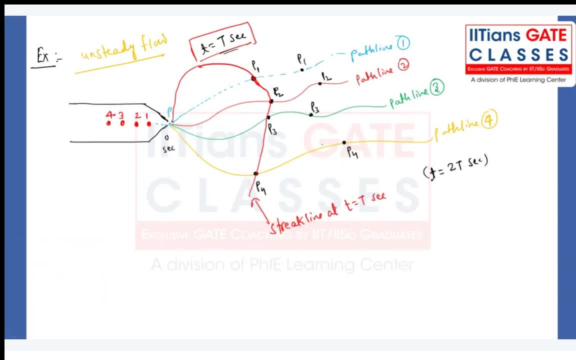 So what I will do? I will join this locus of all the particles through one line, But I will not left it by while joining all the points, simply like that. I will connect this, basically point to the starting point, because everything is injected to a starting point. 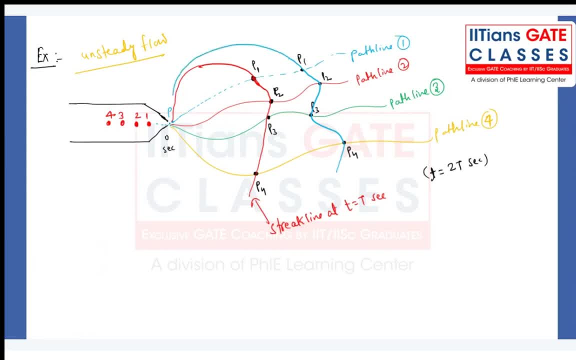 So I will just connect this to the starting point like this: So this is my streak line, at small t equal to capital T. second, Make a note of it. So I hope that the streak line is clear. So what is the meaning of the streak line? 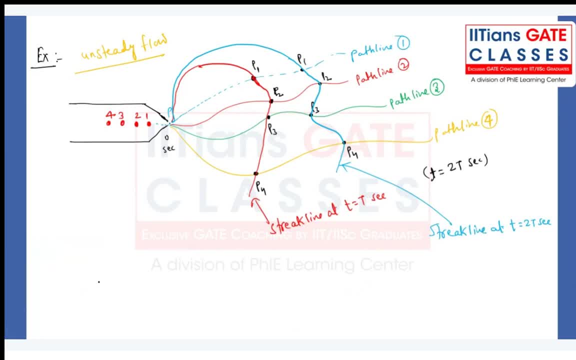 The streak line is basically telling you that, in a very short term, I would say that it is related to the identification of. it is related to identification of t equal to capital T. Identification of location, of location of different fluid particles. different fluid particles. 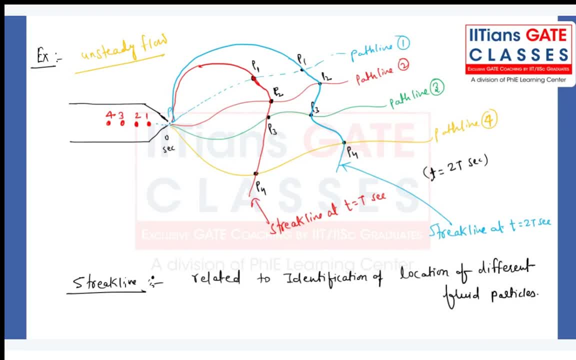 You can identify okay, just by seeing the streak line. particle one is here, particle two is here, particle sorry. particle three is here, particle two is here, particle one is here, Right. So it is also one kind of what we can say. 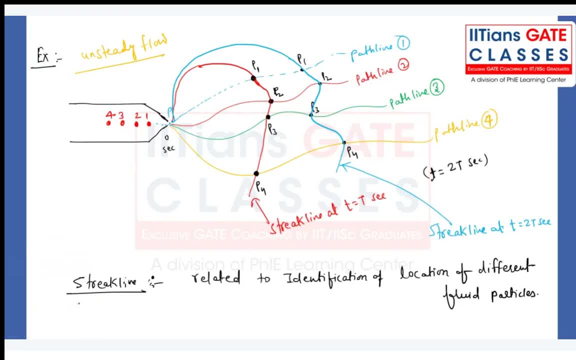 Ah, Eulerian approach. Getting my point, Yes or no, Can you say like that, It is for the multiple fluid particles, right? This line is also for multiple fluid particles, Not for the single particles, right? This is a very, very important. 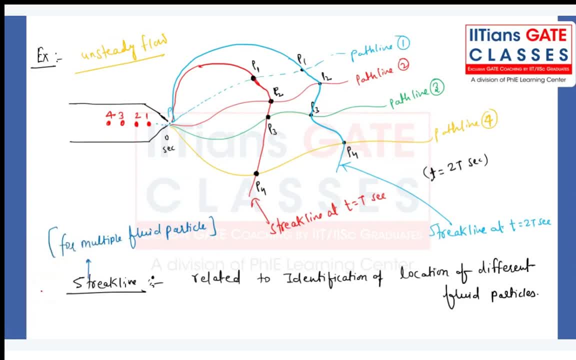 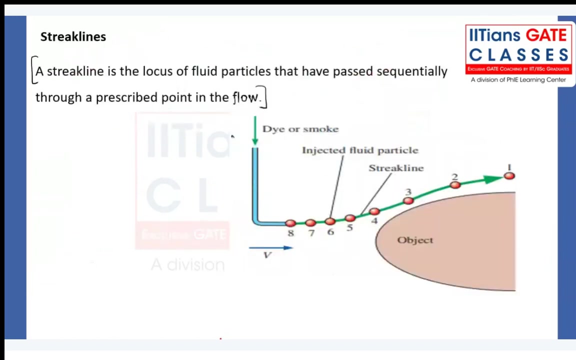 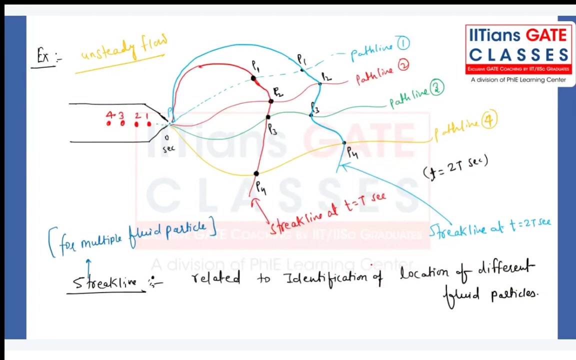 Make a note of it. Once it is done, let me know. It is quite. it is a very important thing, right? Yes, Now all of you have noted down. can I move back to the previous slide to explain that? you can move back to the previous slide to explain that. 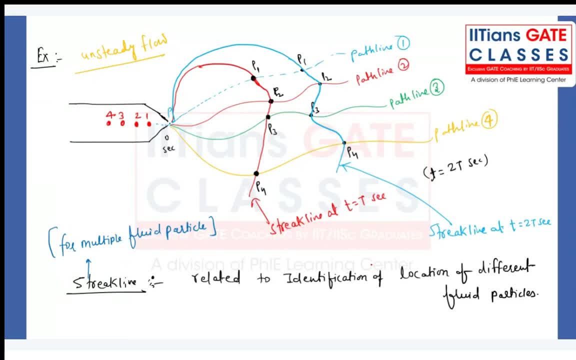 Yes, correct, At a particular instant it is more like a Eulerian based approach because it is for the multiple fluid particles, right, not for the single particles. Now you try understanding this particular figure, how they have drawn this figure. 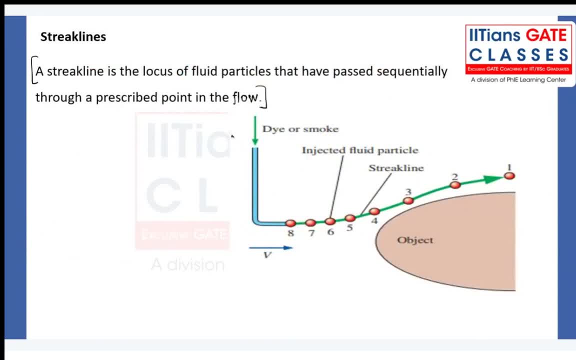 An object is there. On that object, the dye is being injected from here, And it is being injected from like this. So what you have to understand here, the particle one, the particle one may follow this path. Particle two may follow something like this path. 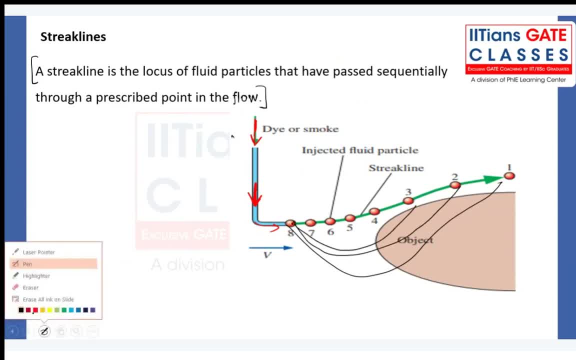 And particle three may follow this path. Individual path lines. I am drawing individual path lines. Particle four: they may follow this particular path. fifth and sixth and seventh right. But it's a coincidence situation that every fluid particle- let's say I want to draw time- 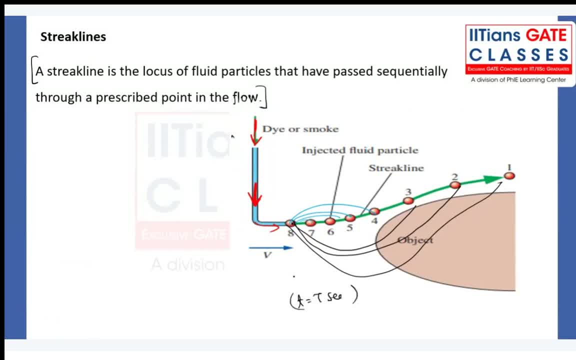 t equal to capital T. second, I want to locate my streak line. So particle one is here, Particle two is here. Particle three is here. Particle four is here. Particle five is here. Particle six is here. Particle seven. Particle eight is here. 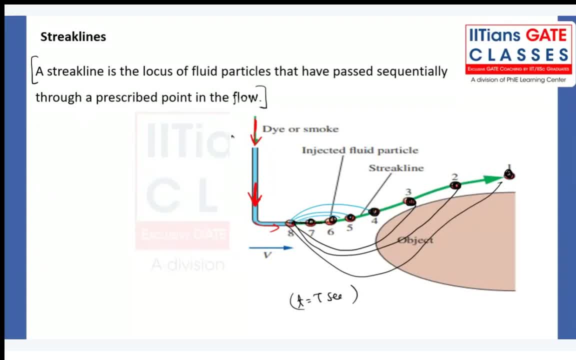 So when you just join the local of location or locus of all the particles through one line from the starting point you will get one line. That line is called streak line At time t equal to capital, T second right. So make a note of it. 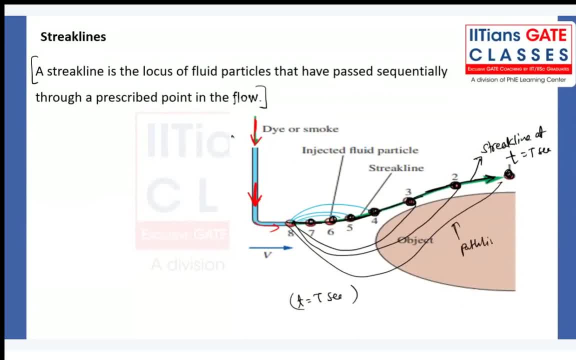 This is the path line for first particle, path line for second particle, path line for third particle, path line for fourth particle, something like this. You make it, You come back up to this here. example: on the first part. Do we notice any problem? 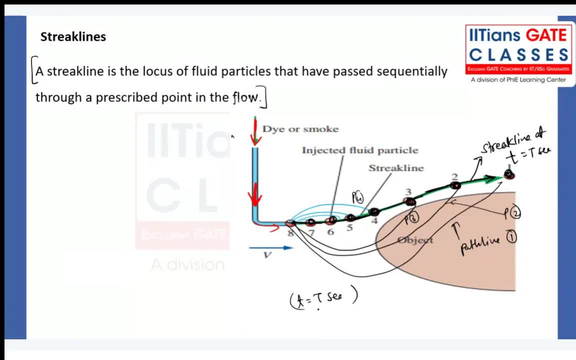 No problem, We can go on. Now see whatever the phenomena is happening. that is a time-based phenomena. you are correct up to some extent. See, the path line is telling you the individual time history of a single particle. You are basically making the video of a particle. 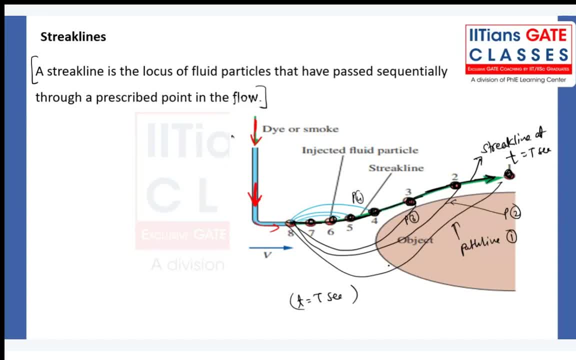 That is the true sense of path line. But what you are doing actually at a particular instant, let's say at any- you have this stopwatch, you are stopping and you will see where all the particles are there And you will take the picture of that. 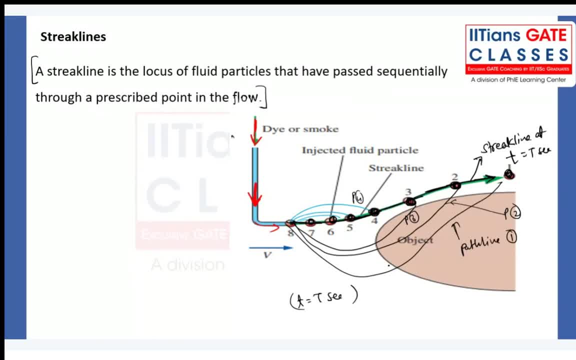 That is snapshot of that instant or moment. you will call that line to be streak line. But streak line when you see that containing number of fluid particles, when you start studying the behavior of a streak line, what you will find- whether you will study like 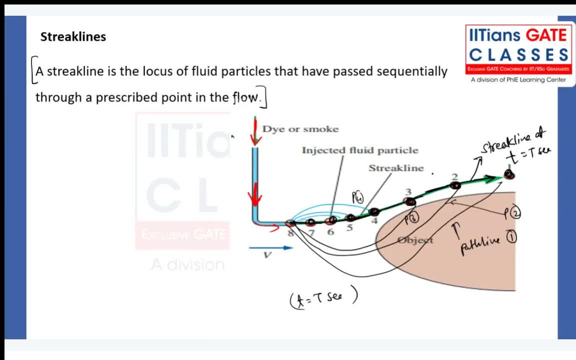 a Eulerian-based approach or Lagrangian-based approach, because Lagrangian clearly mentioned that I won't bother about all the fluid particles. I will bother only about single fluid particles, Let me guess A regular one. You weren't aware of that. 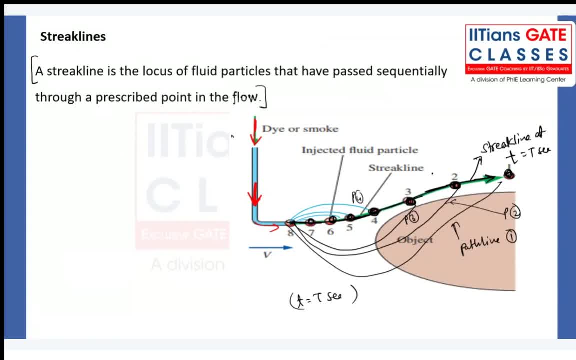 Yeah, maybe. Yes, yes, I see That is smart. That is really great. Thank you. Thank you very much, Dr B difféna. Thanks, Thank you, Thank you. Thank you very much. Have a wonderful day if you have any questions. 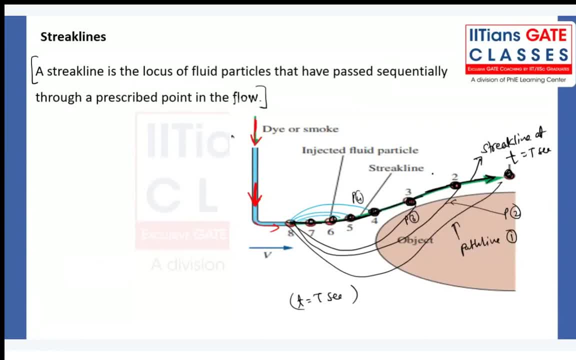 Bye-bye, Bye-bye, Bye-bye. If every fluid particle will follow the same path line, then what you can have? then you can have a streak line that will become a path line and that will be Lagrangian based approach you can study. that is only for the what you call study flow. 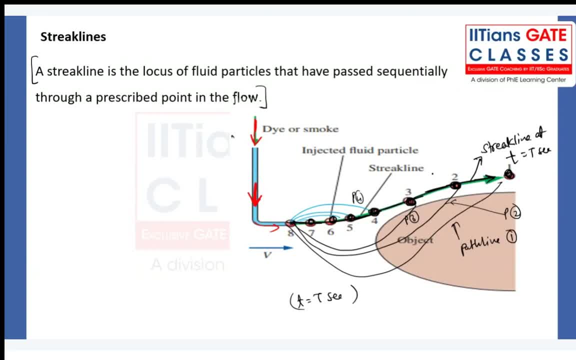 Now, once it is done, let me know. I will explain what is the meaning of study. flow path line is a time history of individual particle. if you want to have analysis of, let us say, the fluid layer, fluid particle is there, you know. let us say, you have the eddy, suppose you have. 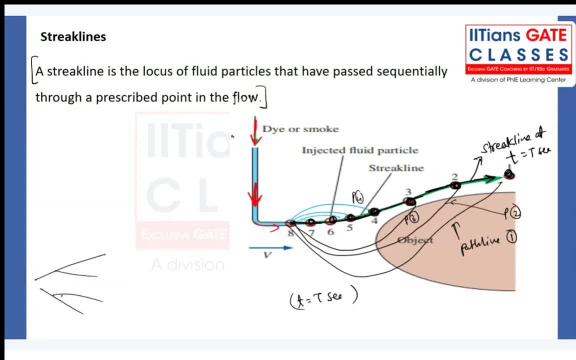 the diverging flow, we have the flow suppression which is being initiated from any of the diffuser wall. so what will happen? this flow suppression? the particle is there. you know this. in this region. we want to analyze what is the kinetic energy of that particle. what is the energy? 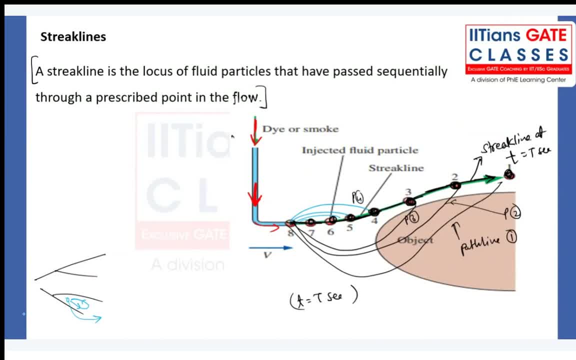 total energy of that particle, right, because that is like a dead body. right, we want to analyze, we want to do the postmortem of that dead body. what we have to do, we have to see complete picture of that body, That body from inside, right. so for that we will, we will be, we will be required, what is. 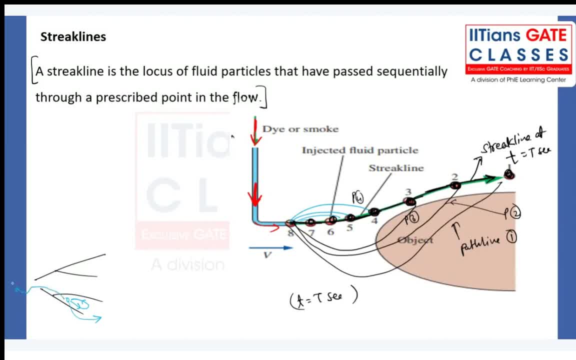 the time history of that fluid particle, from starting from where to where it has traveled. what was his time history? and all right. so in that sense we will be very much interested to know about that. but that is a very microfluidics level of thinking about the path line for path. 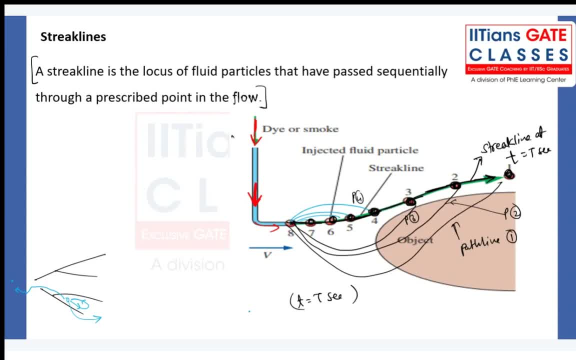 line of single fluid particle that is of totally useless as far as the fluid mechanism is concerned. Right, because here that single particle, forget that in single particle, billions of particle is there. right, you will not be able to identify which is the dead body, which is not the thing. 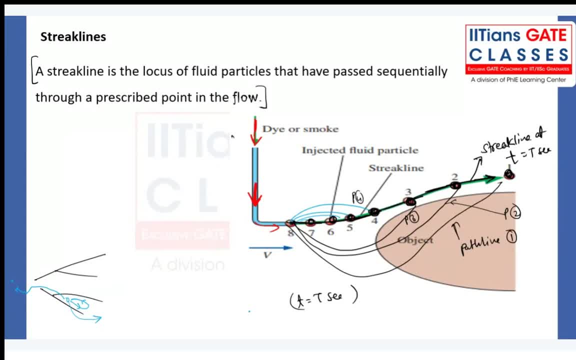 right, just like our happen in the Covid time In our particular area, lot many body's of that right, so you will not be able to identify which is the body if there are multiple bodies are there. so here what we have: billions of particles are there where difficult to identify. still we are studying, just like our path line. 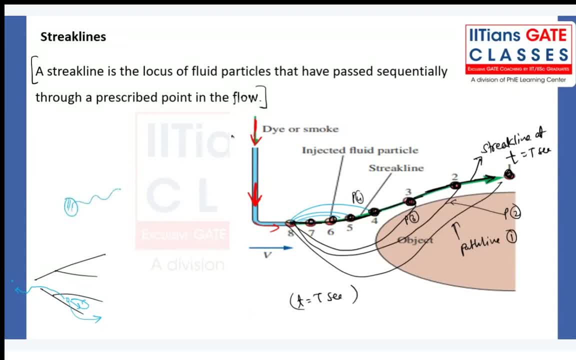 means, just like I said earlier, steel ball which is being traveling right and we can identify and we can see. okay, these are the path line, these are the motion which is being traveled by individual particles. did you remember now? so, when you uh, if you have any further confusions, uh, yeah, correct the smoke which. 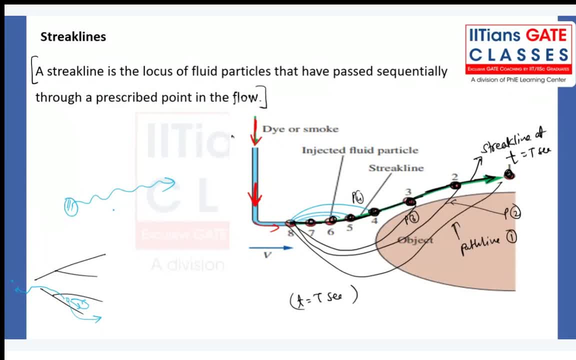 is there, uh, which is from the cigarettes that is, of the street clients. so when you study mit you know. if you need that i will send in the whatsapp group. uh, when mit pdf is there based on? they have done this study on speak line. they have mentioned that it is strictly an eulerian concept. 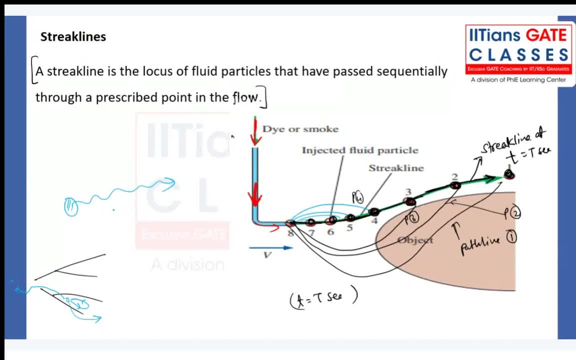 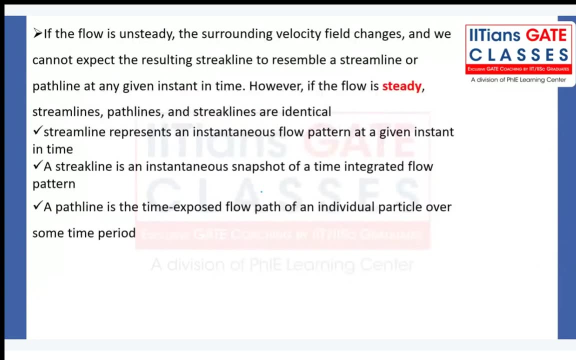 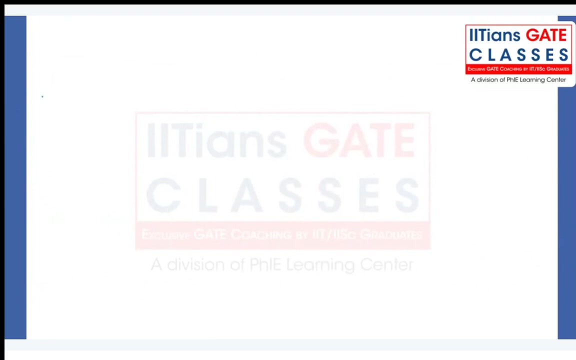 getting my point now. can i move to the next one now? so no doubt, uh, further about this um concept of: yeah, So for a steady flow. you know till now what we have observed. few points regarding the steady flow, Let's say we have 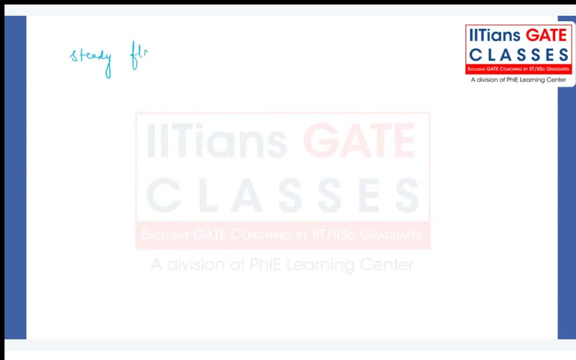 the steady flow and we have the unsteady flow. We have unsteady flow In a steady flow. let's say we have the streamline, something like this, And what we have suppose. for example, at the moment I am drawing, these are the 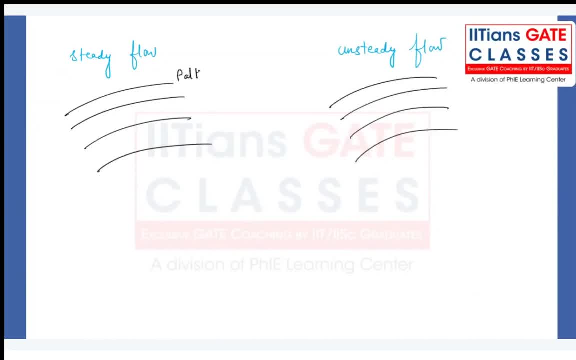 pattern of the streamline. What is this? Patterns of patterns of streamline. Patterns of streamline Supposed the fluid particle. let's say 1,, 2,, 3, 4.. For a given instead of time, if I draw the tangent. 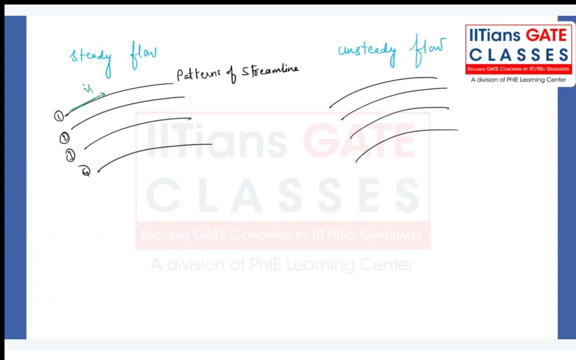 over here I will be getting one velocity vector, v1.. If I draw here, I will be getting v2.. If I draw here, I will be getting. I will be getting what? v3.. Now, at time, t equal to t1, let's say the particle. 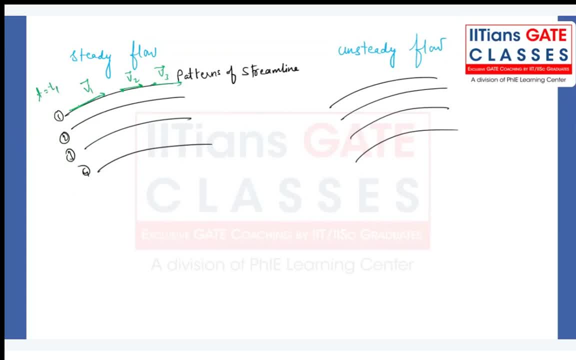 velocity is what. Particle velocity is in the same direction At time. t equal to t2, the particle velocity is what? Once again the same, Because it is a steady flow. so dou u by dou t will be 0. The velocity will not change with. 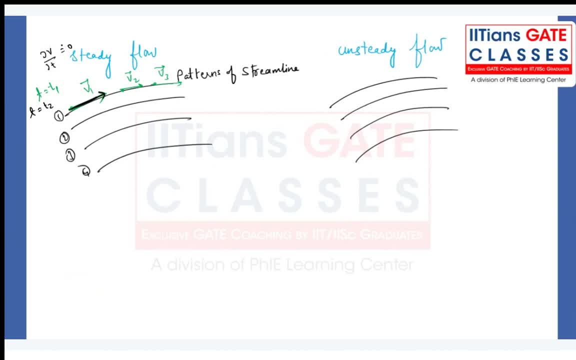 respect to time, When the velocity will not change with respect to time. now, tell me whether any pattern of streamline will change. v1 fixed in both. 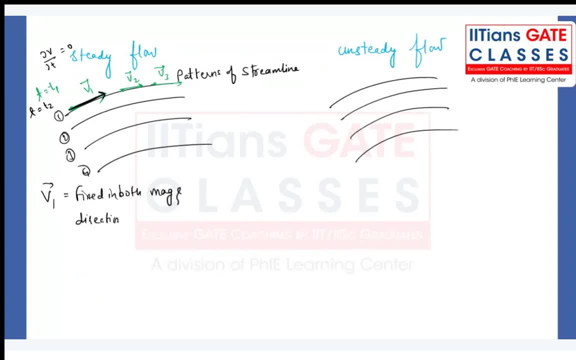 So what we can have, The pattern of the streamline will not change. So what we can have, The pattern of the streamline will not change. 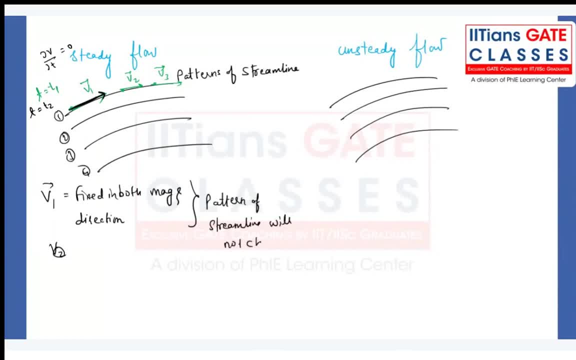 Pattern of the streamline will not change. The moment we have the v1 velocity, for example, let's say here at time t equal to t1. But at time t equal to t2, the particle is changing its direction, as it is an unsteady flow. 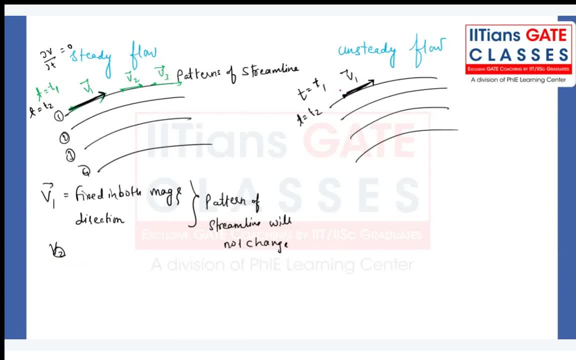 either i change the magnitude or i will change the directions. i can have the different streamline, something like this it has. now it is being traveling like this. so if i draw the tangent i will be getting v1 dash, something like this, because the pattern of the streamline has been 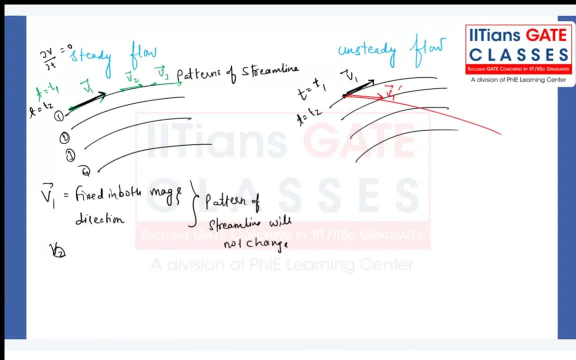 changed because of unsteady flow. so if i draw the tangent- you know, because velocity is like this- if i draw the tangent i will be getting a streamline pattern, something like this: right now, this is the streamline we are getting at time: t equal to small, t2, sec, t2 second right. so what is happening over? 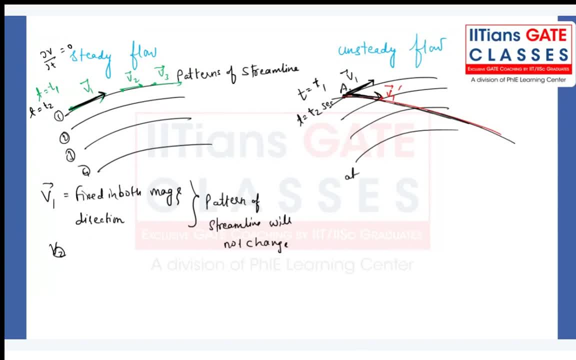 here at a point. a velocity a, that is velocity of the particle at a, is v1 at time t equal to t t1 second. but velocity of the particle a is v2 or v1 dash at time t equal to t2 second. right, so so. 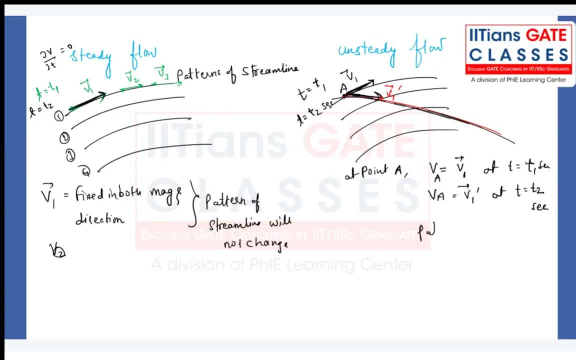 so the pattern of the streamline will be changed. pattern of the streamline will change, so make a note of it. now. what is the consequences of that? what are the consequences of that? now you have to imagine a particle. now you have to imagine a particle which is being traveling on a first streamline, right when the particle is being traveling on this. 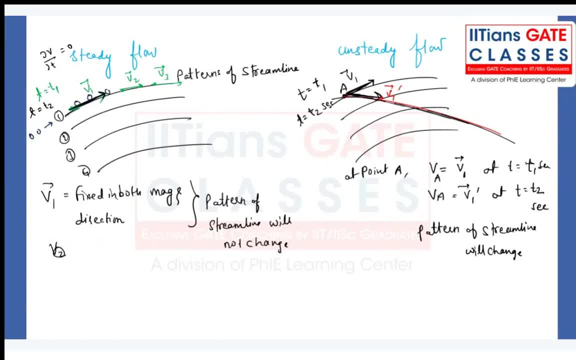 streamline on this streamline. now tell me. they will not change their directions or they will not change their magnitude, right? so what will happen? they will remain on the same instrument because we know that the particle might defend the particle. all the particle. particle number one. particle number two. particle number three. particle number four. particle number five. particle number. 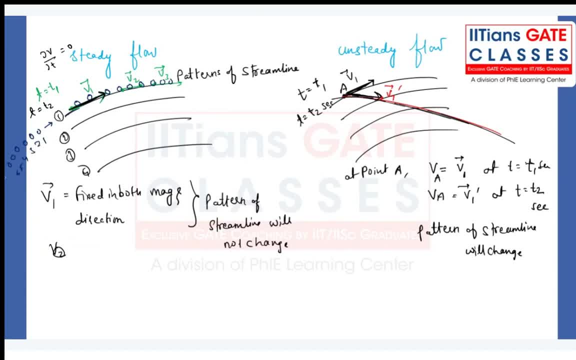 six. they will not change their directions. the pattern of the streamline will not change. so it is something like: they cannot move like this, they cannot move like this. still, they cannot move like this, they cannot move like this. so they will remain on the same streamline. so what we can say for a 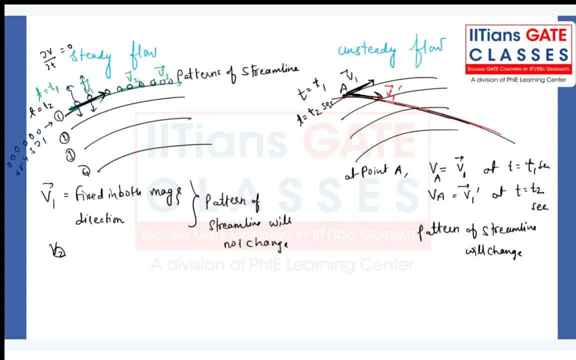 steady flow: path line, stream line, and even you draw the local of locus of all the fluid particles from the starting point, you will be getting same line which is being joining from the starting point. that is a streak line. so for a steady flow, what we can write: 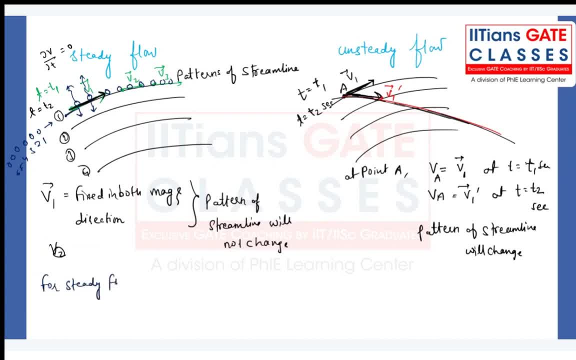 for a steady flow. for a steady flow, path line will be equal to the stream line, will be equal to streak line. right now, on the steady flow by defense, what can have suppose a part number of particles are there which is being traveling on this first streamline right? 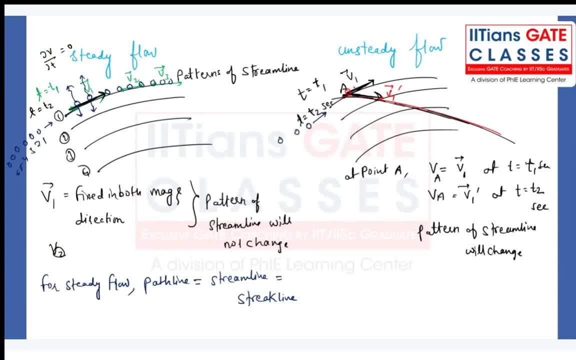 So what can happen? Some particles are traveling like this, you know, and the moment unsteady flow is there. So some particle may travel like this, some particle may travel like this, right, So what we can have? We cannot have the same stream line and we cannot have the same path line for our individual. 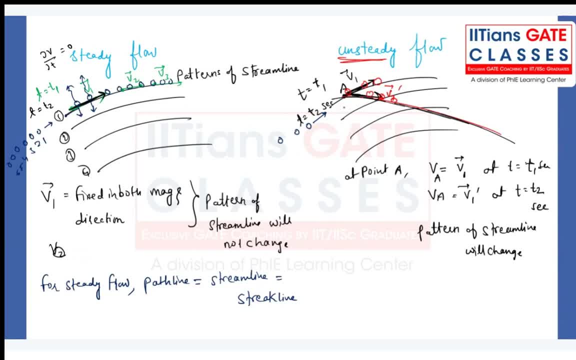 particle. Even when you join the line from the starting point, we may have the pattern of a streak line, something like this. So all together we can say path line of a particle and stream line and streak line. all are different. So, just like what we have discussed earlier, individual particle may travel individual. 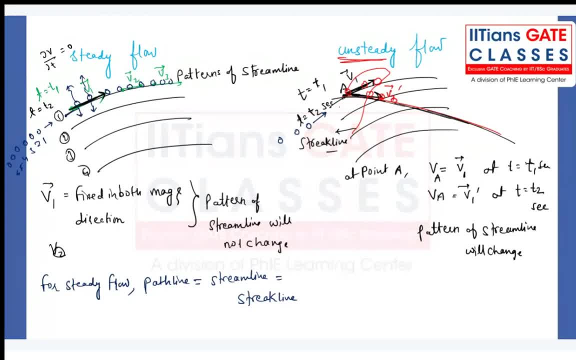 path line. Why? Why it will travel. Suppose a particle 1 is there. he is traveling like this. The particle 2 is there. particle 2 will travel like this. Particle 3 is there. particle 3 will travel like this. 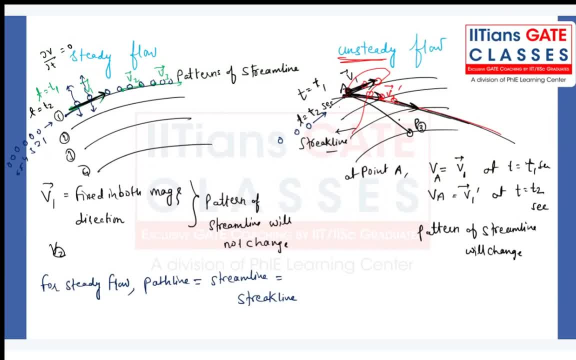 Particle 3 will travel like this, So they will not have a fixed pattern of a stream line. Getting my point, They may travel with a different, different, different, different what Path line And what we can have. Different stream lines will be there and different streak lines will be there. 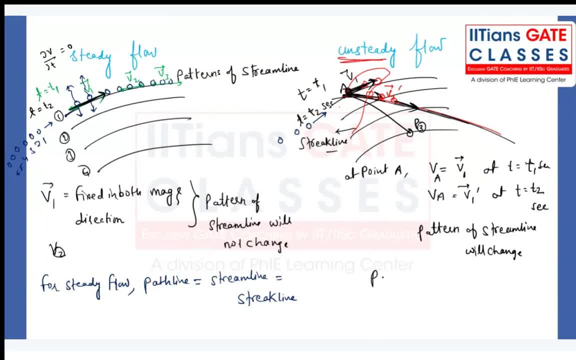 So for unsteady flow we cannot say the path line that is equal to stream line, that is equal to streak line, Getting my point. So for unsteady flow, all the three lines will have to be same. So for unsteady flow, all the three lines will have to be same. 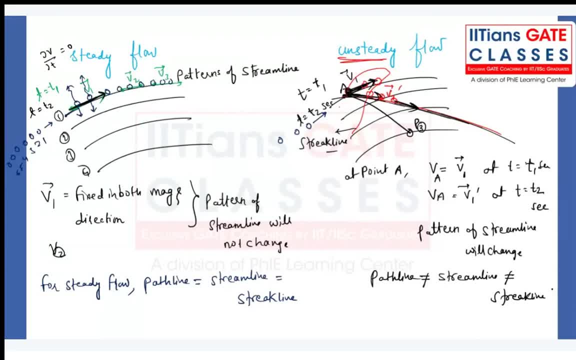 So for unsteady flow, all the three lines will have to be same. All the particles would follow the same path. in steady flow, it does not matter, it will be straight. No, no, no, no. stream line will always be a curvature line, you know it will have a. 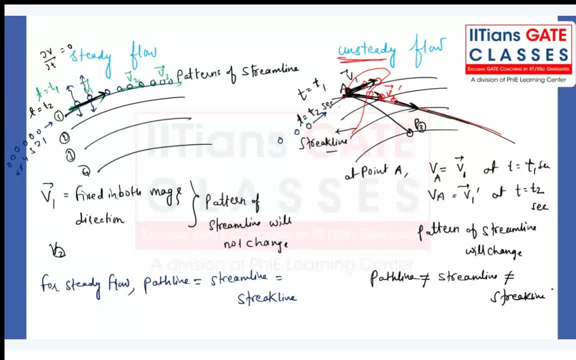 curvature, or maybe it can have a straight line when it is flowing through a constant diameter pipe. Getting my point: Suppose particle is travelling on a fixed straight line, what about the stream line? The stream line will also be like this same. both will be same tangent of velocity as. 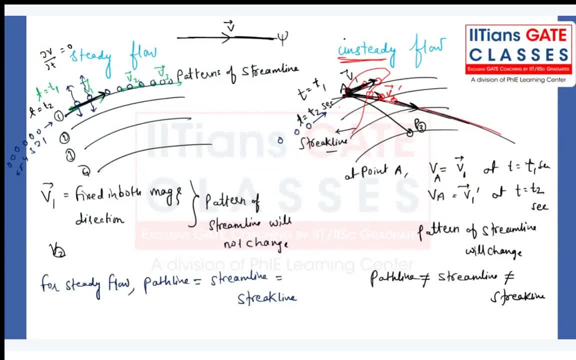 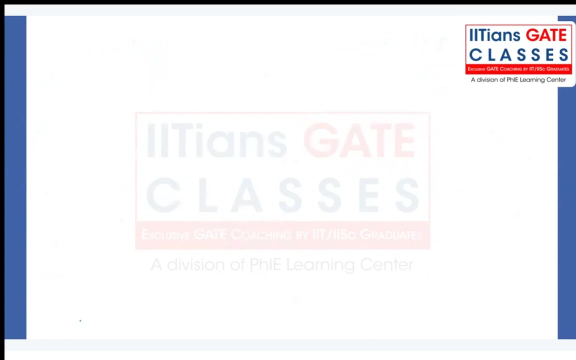 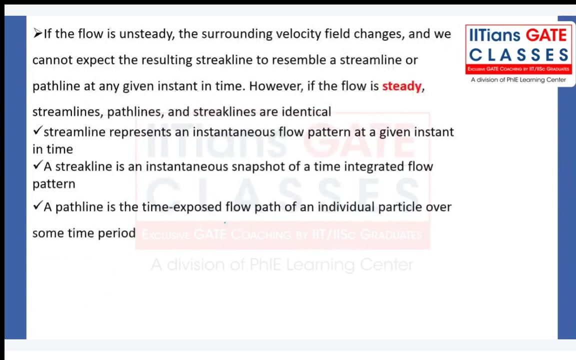 well as stream line will be same. there will not be any curvature. why there is a curvature? Because particle velocity or direction is being changing in a circular flow motion, and all Now. so note down the few points regarding the path line, stream line and a straight line. 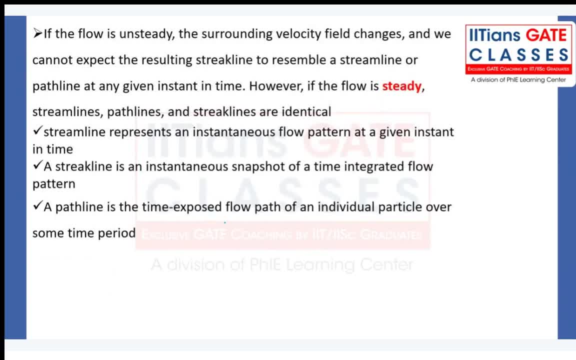 If the flow is unsteady, the surrounding fluid velocity field will change. if the flow is unsteady, as we have seen, the surrounding fluid velocity field will change. So if the flow is unsteady, the surrounding fluid velocity field will change. 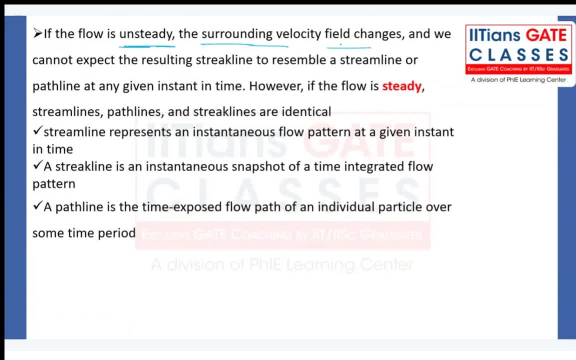 Why it will change. Either magnitude or direction it will change and we cannot expect the resulting straight line to resemble or to look like a stream line or a path line at any given instant of time. However, if the flow is unsteady, all the three lines, whatever the lines we have studied, 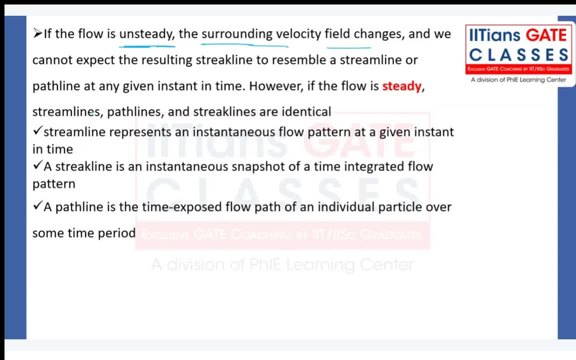 stream line, path line and a straight line will be same. In short, stream line represents an instantaneous flow pattern At any given instant of time. A straight line is an instantaneous snapshot of a particular time-integrated flow pattern And a path line is a time-exposed flow path of an individual particle over some time period. 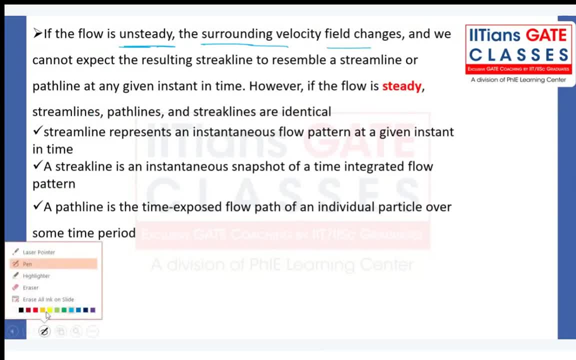 And a stream line is a time-exposed flow path of a particular time period. In short, a straight line represents an instantaneous flow path over a particular time period. Let me ask you another question. Tell me, guys, One question has been asked. 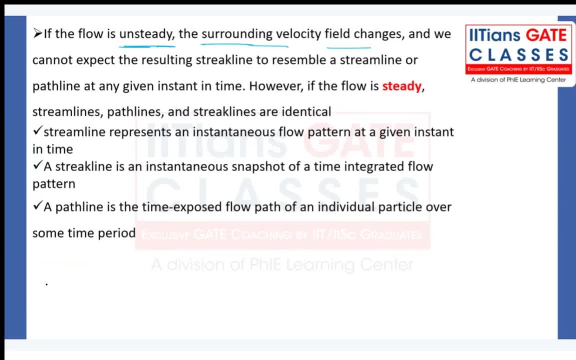 Then what about the pattern of the streamline, For example, airplane is there. whatever the airplane is there, it is being traveling and the ball is being thrown out. It will travel like this. So what about the streamline Air drag will be there. 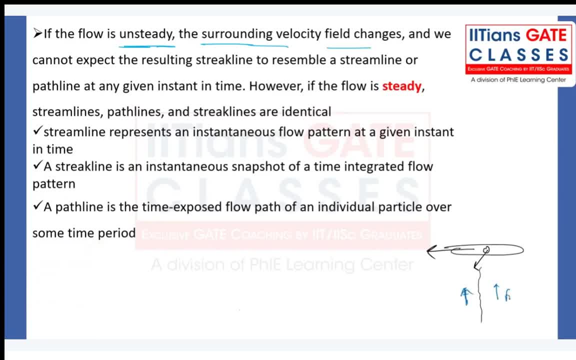 Air drag will be there, But that air drag, whatever the drag, is there. what is the drag force by the air? What about the drag force by the air? That will be small, That will not be that much high Because according to Stokes' law, you will be having some air drag. 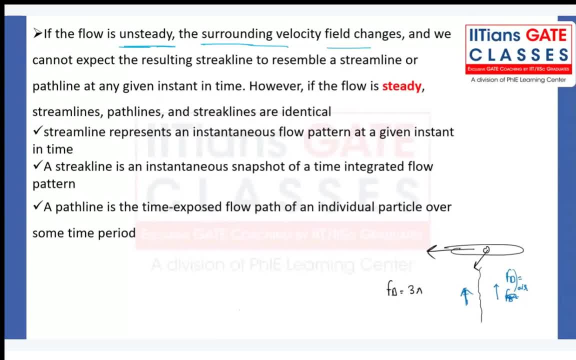 What is that? 3 pi mu? Something like this. If we just assume this is the ball of diameter d, So they will offer some kind of drag force, right, And some weight of the body will also be acting. No, just a ball is being thrown from an aeroplane window. 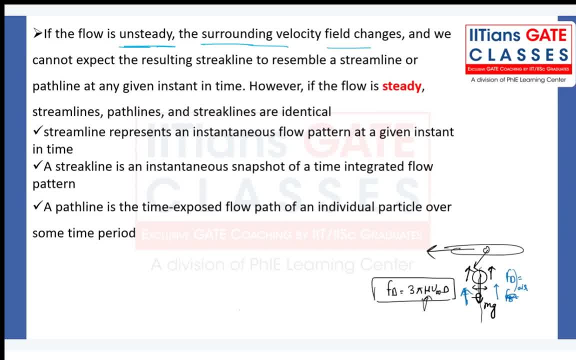 As the viscosity of the air is very small, I know So the drag force which is being there, which is being imposed by the air, will also be very, very small, Right, So there is no option. It is just being asked in one of the interviews. 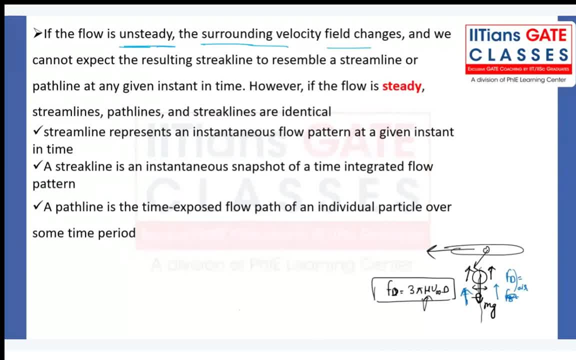 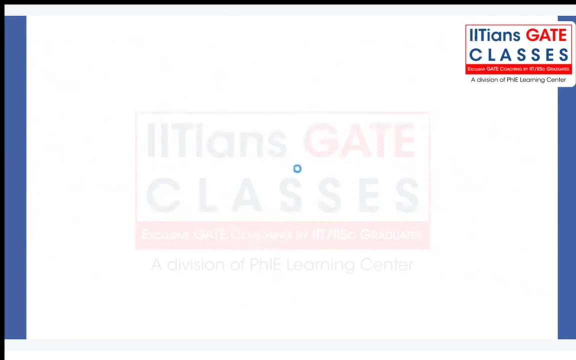 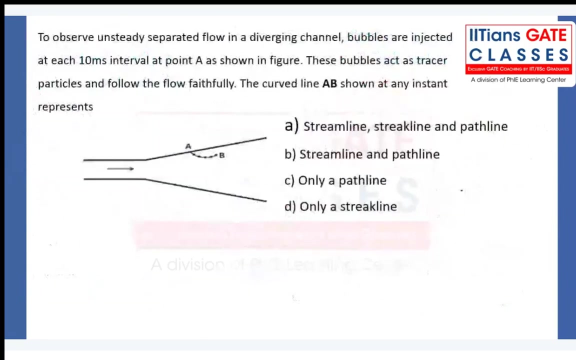 You just think and let me know the answer. That is a very good question. Now, all of you have noted down this particular point. Is it done? No, we have to draw the streamline. Okay, Now try to think of this particular question, which is being asked in aerospace 2014.. 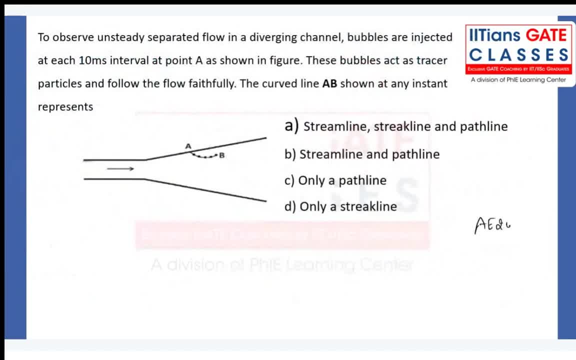 In the 2014 paper, they have asked one question: Is it possible to observe the unexpected flow of air into a diverging channel? Yes, To observe the unsteady, separated flow in a diverging channel, the bubbles are injected At each 10- basically millisecond interval. at a point A, the bubbles act as a pressure. 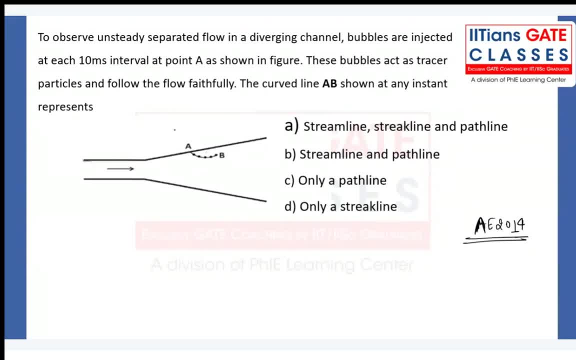 particle and follow the flow faithfully. The curved line AB. whatever the curved line is there, AB will be called as what It is called: the curve path. It is called the curve path. It is called the curve path, curve path from A to B, So individual particle may have travelled like this particle one. 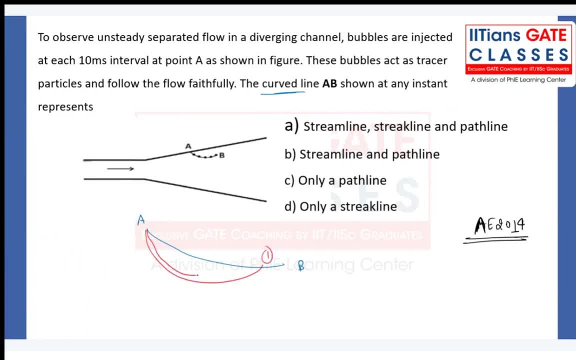 is here. particle two is here. particle three might be here, but the blue colour which I have drawn, that is been connecting all the fluid particles at some time time. t equal to t second: that is my streak line, Because this line containing number of fluid particle, 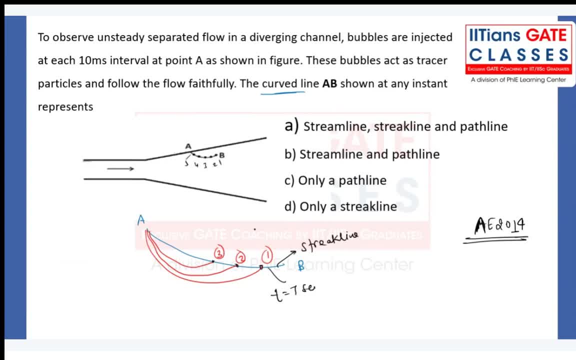 one, two, three, four, five and number of fluid particle means what? when we have the multiple fluid particles, which line is generally resembling which will give you the snapshot of all the, for all the position of the fluid particles? only a streak line. Now some of 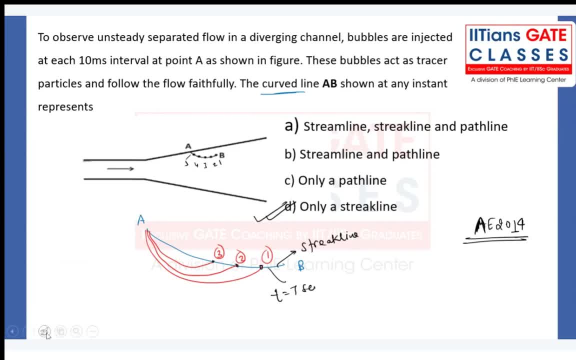 you might be thinking why it cannot have the stream line. tell me this, because when you consider stream line, what do we have? that is also for the multiple fluid particles, right, correct, correct, because the stream line when you draw, you know at any point. 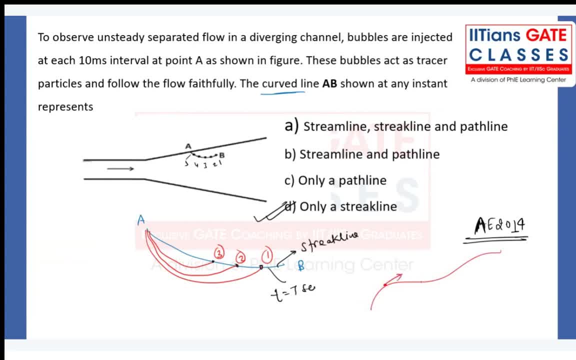 when you draw the tangent, it will give you the direction of velocity vector. it has nothing to do with the identification of particles at a given instant of time. right, it is of no use of that. we cannot tell by using the pattern of the stream line. right the it. 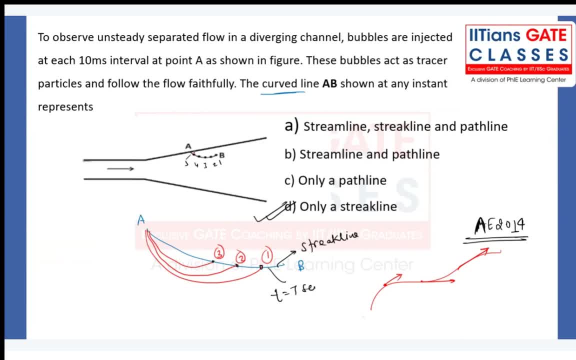 the help of pattern of the stream line. it is only showing only one pattern. right, it is only showing the one pattern and of course that cannot have because it is unsteady flow. so definitely it is not the stream line, so it can have only the streak line. Now tell. 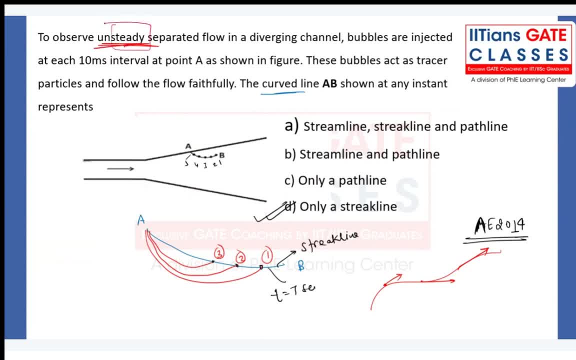 me. if it is a steady flow then we might have a option that is all: the stream line, streak line and the path line will same. but separated flow cannot have the condition of a steady flow. that is highly unsteady flow, separated flow right. 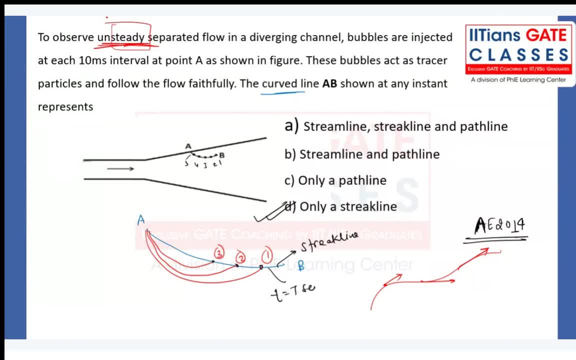 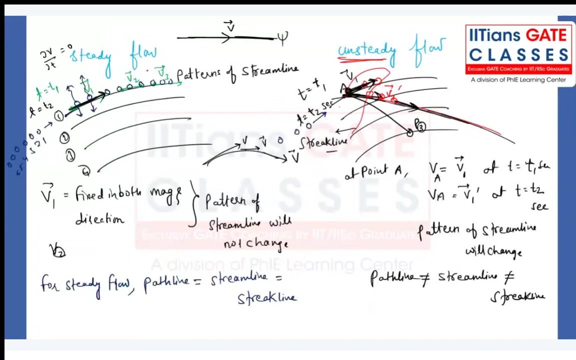 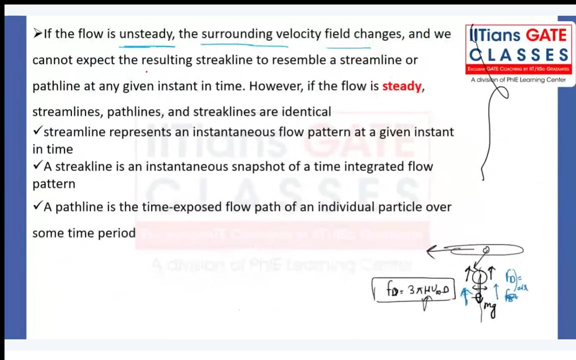 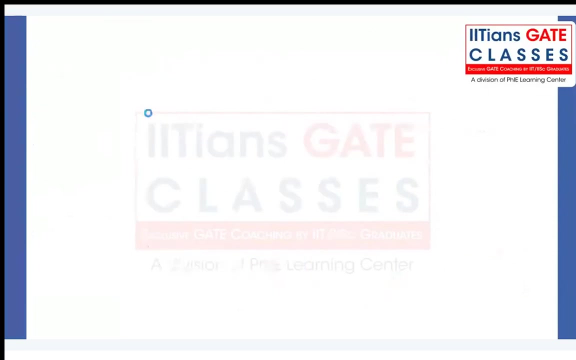 Done, Is it done? Now, tell me the timeline. the next concept: timeline, As the name itself is suggesting that over a given period of time, or basically at a given instant of time, whatever the, you know, the set of adjacent fluid particles, right it? 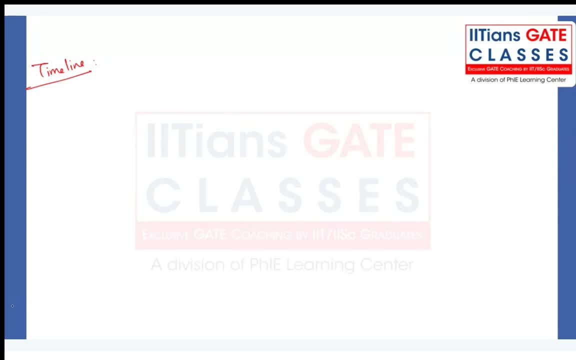 is telling you the set of adjacent fluid particles. Let me tell you. suppose this is a fluid particle or some velocity flow field. Note on the first of all definition. these are the lines. timeline are the lines formed by. it is a line, don't think that it is a history telling just like a path line. you. 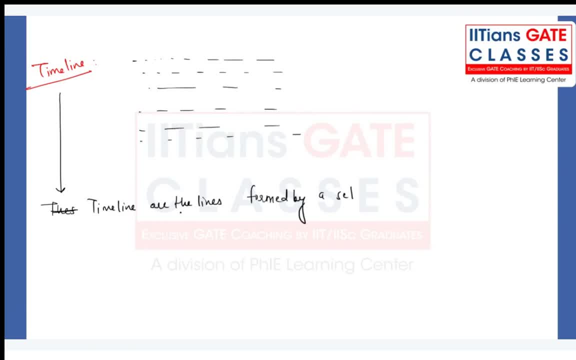 know not, not like that Timeline. basically, are the path line, are the lines formed by a set of fluid particles, formed by set of fluid particles that were marked, that were marked at a previous instant in time, At previous, At the previous instant of time. 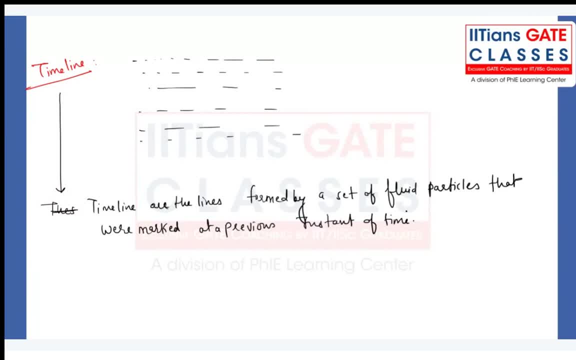 Now suppose we have the fluid particles. assume the fluid particle which is being injected, like this, for example, means I am just analyzing which type of flow field it is there with the help of timeline. For example, the fluid particle one is here, particle two is here, particle three is here. 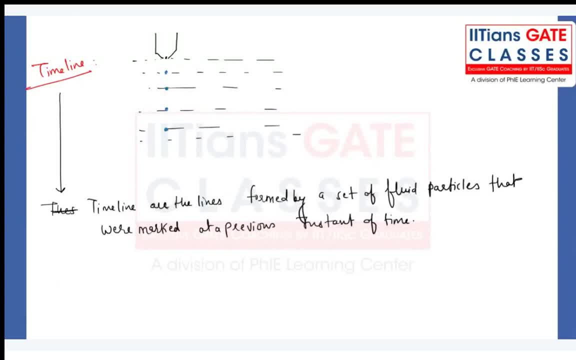 particle four is here And just connect This, all the four particle, by some line. for example- let me just consider this through a line- something like this: just like a thread, assume it like thread- All the fluid particles are basically connected to this thread, right? 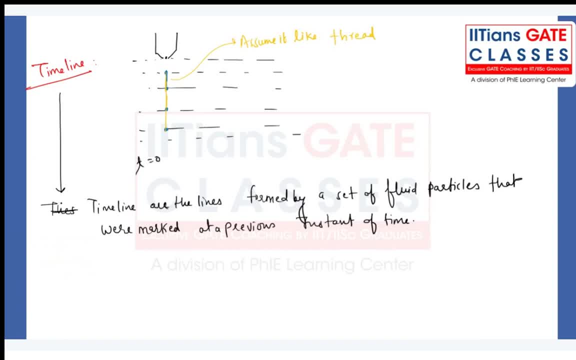 At time t equal to zero, for example. now the flow is happening. These are the fluid particles that were there instantaneously at some given point of starting point of time. They will be there, But now, let's say, the flow is happening with some free stream velocity. 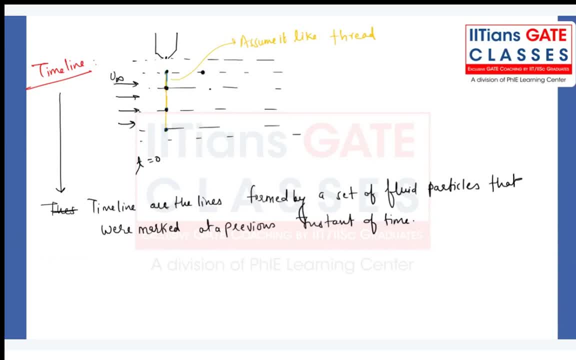 Now the particle which is being marked. now they have been displaced from their position, something like this: When they have been displaced, so what will be my thread? thread will look like this. The thread will look something like this: Okay, Okay. 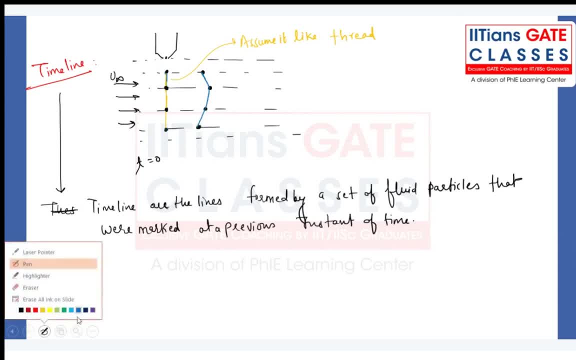 So, like this Further, what will happen at some given instant of time? my particle will be something like this, And if I join through this thread, I will be getting like this. So what we are observing is that it is which kind of flow field? because you can only see. 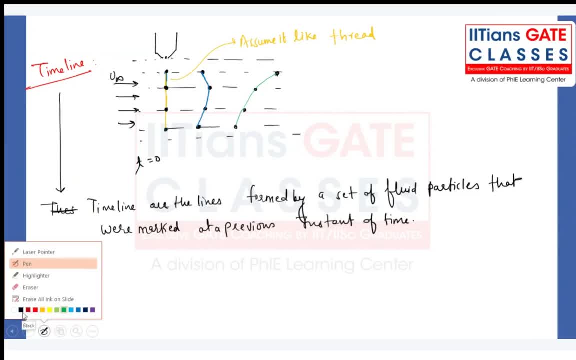 that there is some deformations are happening. Fluid particle initially were straight, but now they are deforming, right, It is something like this: Something is there that is rotating the fluid particle. What is that Rotational flow field? It is a rotational flow field. 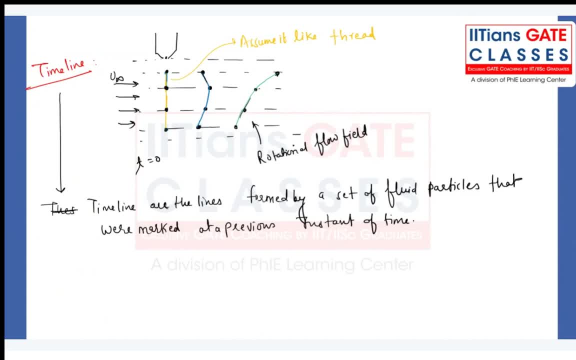 Right. So it is a rotational flow field. That's why the thread is basically bending or taking the curve shape. But, for example, we have the fluid particles and that fluid particles, we have the thread, something like this- That were initially straight and they were straight even after flow is happening. they 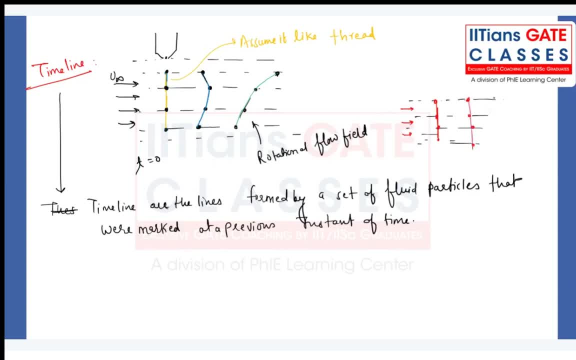 will be straight all the time, all the time. Then what we can say? what we can say, at t equal to 0 hours, 1 hours, 2 hours, then what we can say, this is nothing but non viscous flow field, non viscous flow field. 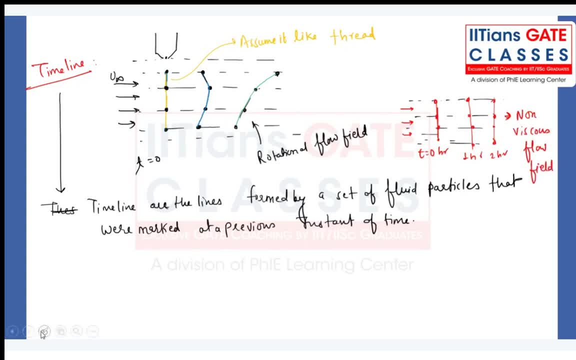 Okay, Okay, Okay. So the first field- you are saying that a rotational or viscous flow field is there, right? Rotational means force vortex and irrotational what we call that to be what? free vortex? Getting my point? Vortex flow is a two types. 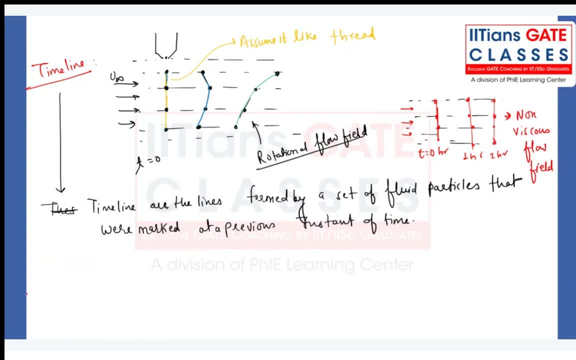 One will be. one will be called as. basically, one will be called as force vortex. second will be called as free vortex. You can say that uniform flow is there about the non viscous flow, because whenever the non viscous flow is there, the velocity profile remains unchanged. 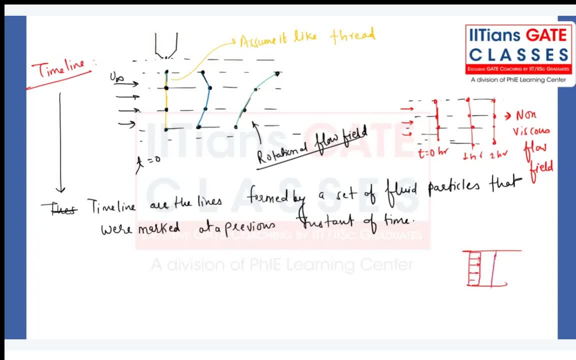 Okay, It will not either move in radial direction or in the axial directions. It will remain same, just like a free stream, velocity conditions. So timelines are the lines, this yellow lines, which are formed by the set of fluid particles that we have marked at a previous instant of time. 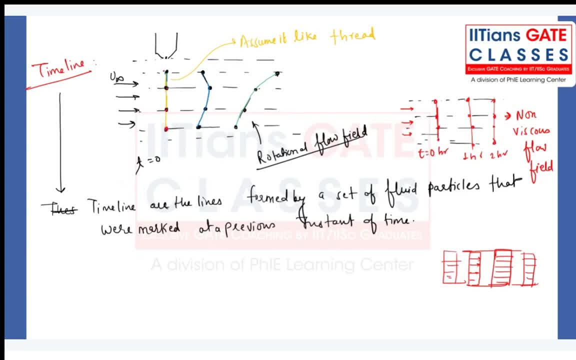 So these particles are there that we have marked at some given point of time And we will see how these particles are changing their positions. See that over the given period of time I will be connecting through this, all the particles through one line right. 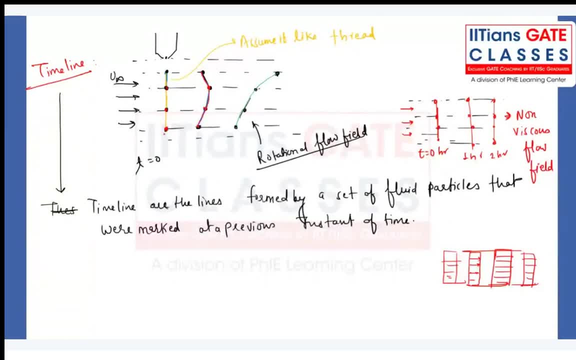 That is my timeline, So that is the fourth line. So there is no connection of this with the streak line or what we call path line. It is a different, because these lines I'm joining not from the starting point, Let's say they have been injected from here. 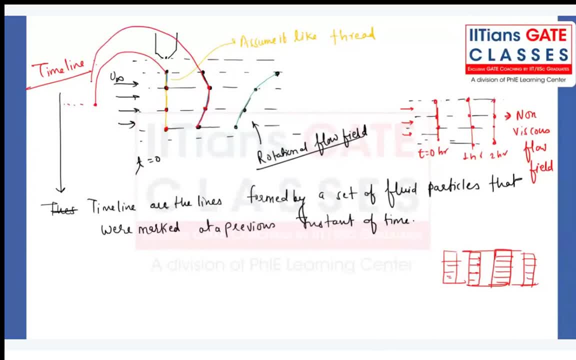 I'm not joining like this. Don't think that it is connecting all the fluid particles. so this is our streak line. No, I'm just joining through instant of time. That's it. I have just marked the points. Okay, These are the particles at time. t equal to one, two, three, four means at given time. 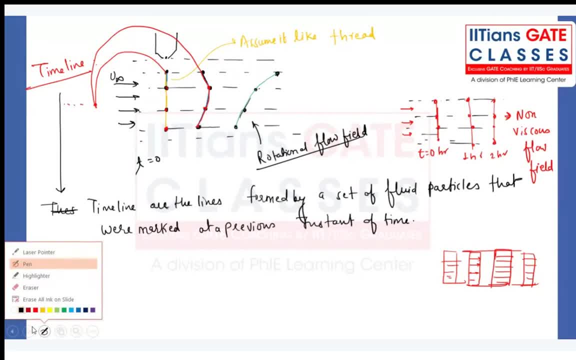 Once again, adjacent fluid particles are at this location. I'll be joining that through a line. So I'm not joining through a starting point from where they have been injected. So I'm not joining through a starting point from where they have been injected. 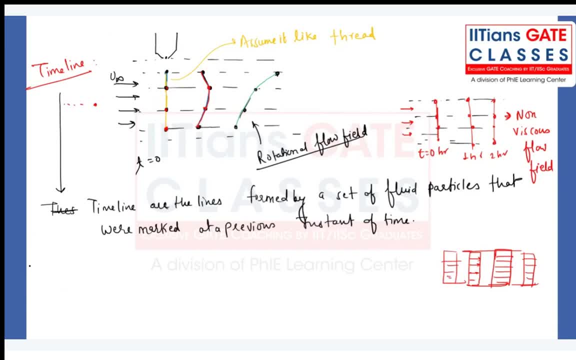 So I'm not joining through a starting point from where they have been injected. Okay, So that is the third line. So I'm going to connect with the starting point. Sit on it. Let's see that. Yes, if you want to do the experiment, somebody will be asking you how you will check whether 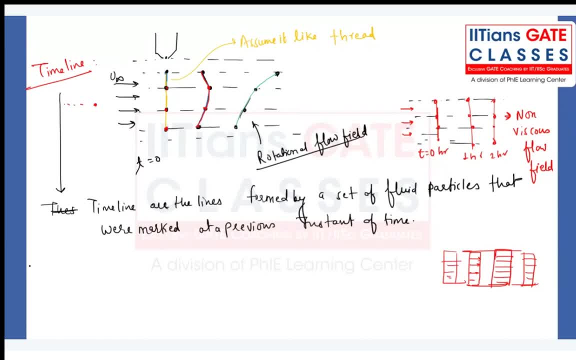 the flow field has been viscous flow or viscous flow or non-viscous flow. So what you will say, sir, boundary layer formation is there, but boundary layer formation is there. you can say by that, but boundary layer is a very thin region. you know very, very 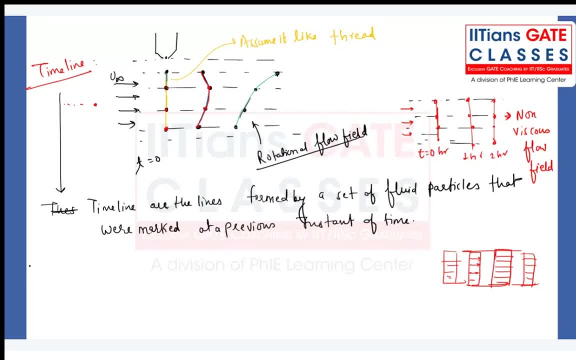 thin region as compared to the fluid domain, whatever the fluid domain is there. So we cannot actually identify through that. So definitely we have to follow some timeline method to identify whether the flow field has a rotational flow field or irrotational flow field. 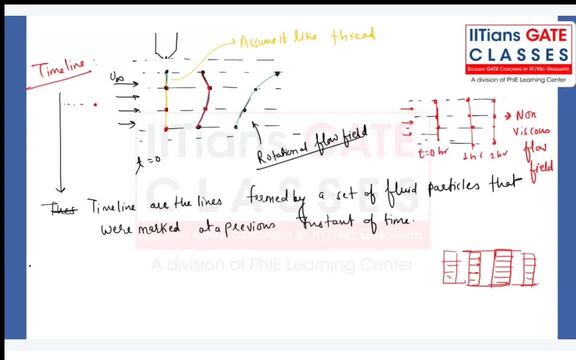 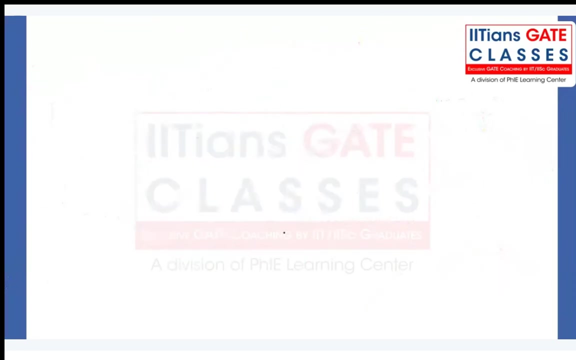 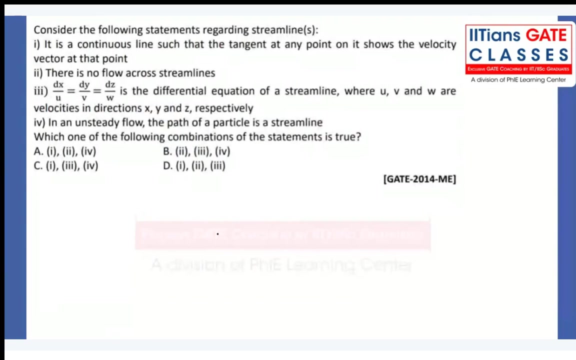 Done. Can I move to the next? All of you have noted down. Can I move to the next one? Now note on the next concept. That is nothing but not trying to answer this question. Consider the following statement regarding the streamline: It is a continuous line such that 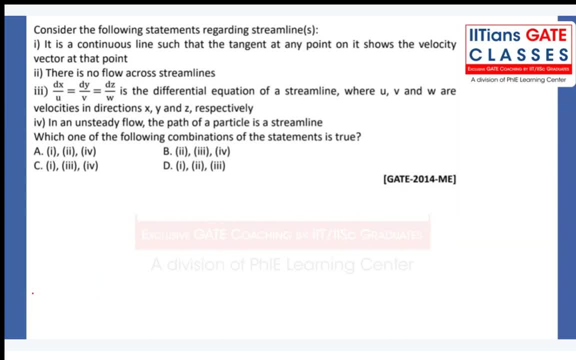 Tangent to It is to make. at any point it shows the velocity vector. at that point there is no flow across the stream line, And this is the equation of a stream line. that is correct. in unsteady flow, the path of the particle is same as a stream line. that is correct. 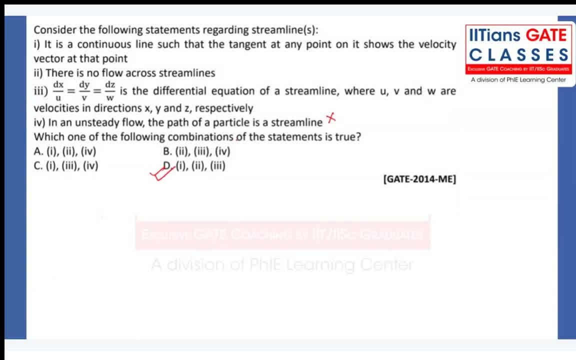 So one, two, three is correct, so D will be correct to make a note of it. There is a no flow across the stream line. suppose two stream lines are there and particle one is here which has been traveling right, So this particle cannot flow across the stream line. 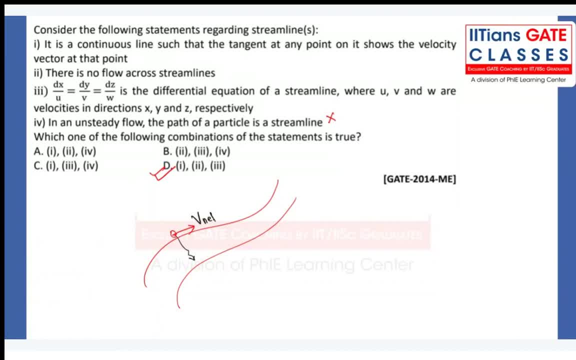 Like this Because the net velocity is in the direction of Something like this: along the tangent directions, all the net velocity right. Some particles are having you, some particles are having we. the net velocity is like this, So they cannot travel perpendicular as there is a no component of velocity. 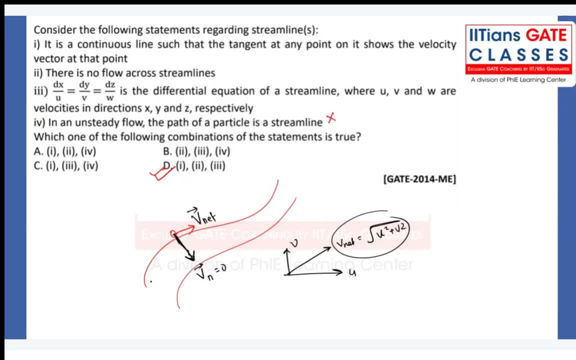 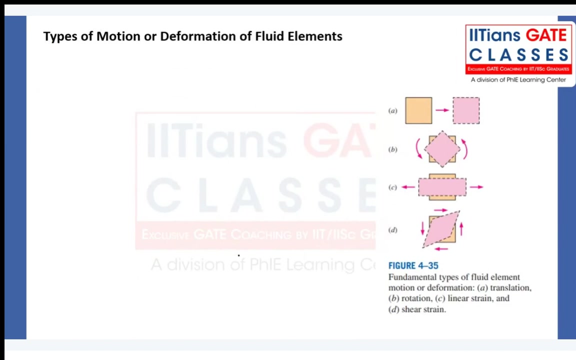 Normal component is zero. Right, Yeah, Now, once it is done, let me know: Okay, So we calculate G today. Just give me the counter thing: Yeah, Okay. My other question is about that. right, Yeah, So all you have to do, right. 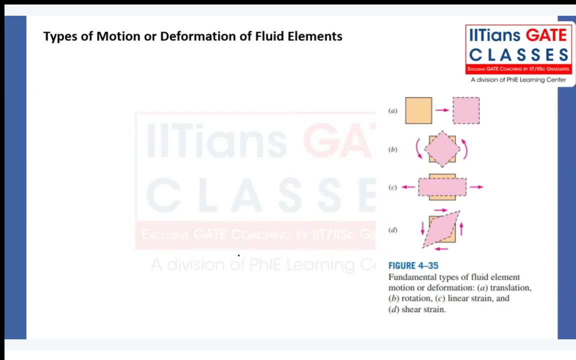 Any sieves. So you have a storm, Just like a solid body. they can also translate. they can also rotate. they can have the shear deformations and they can have the linear deformations. As you can see, this is translation. it is being mentioned in the figure. it is being 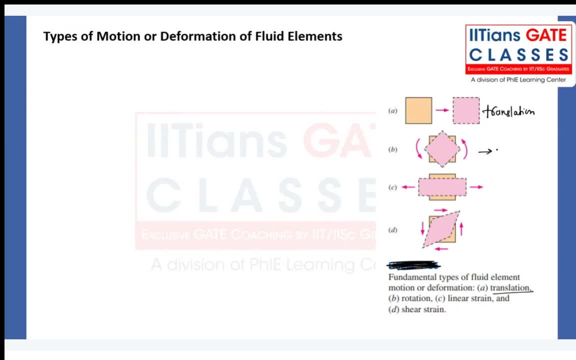 given translation. B is a rotation, C is nothing but linear strain rate and this is nothing but shear strain rate. This is a shear strain and the term we use notation wise rate, because in fluid mechanics rate of deformation is important rather than deformations. 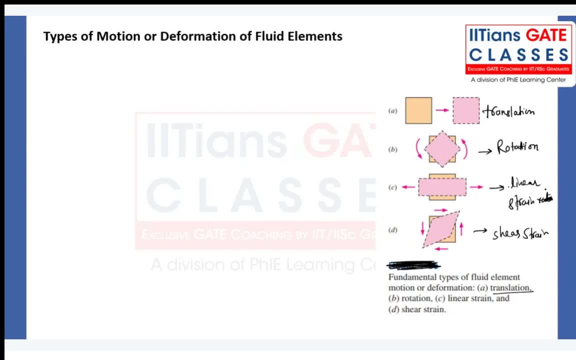 So in the SOM You might have studied the strain rate change in dimension by original dimensions. But you might be thinking, sir, here, what is the particle dimensions? how we can analyze the fluid particles dimensions. So let us see one derivations, and then, in a very similar fashion we can write for other. 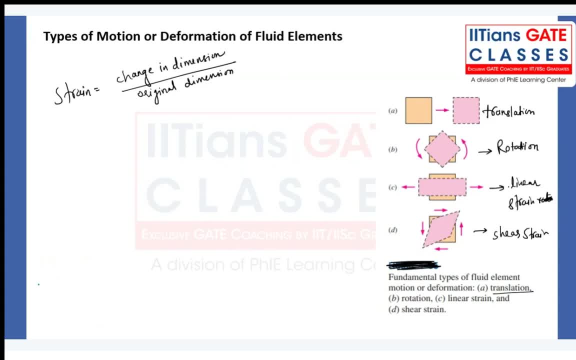 parameters like other motion, that is, rotation, linear strain or shear strain and translations. Let us see for a linear strain or linear deformation of a fluid elements. Done, can I move to the next see here we try understanding. there is nothing to write. 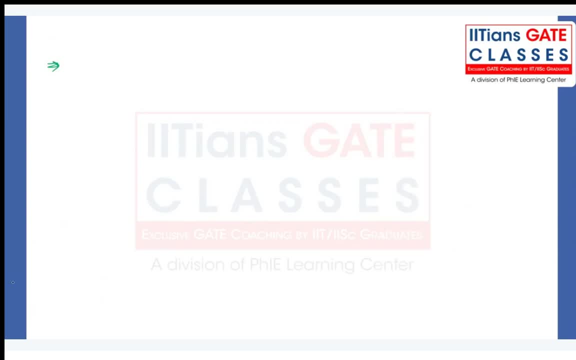 as of now. now, linear deformation rate, Just like what you have done. study about the solid body. let us say we have this solid body. when I just apply the load to this solid body, there will be some deformations will happen. there will be some deformations which will happen: delta L and this deformation. 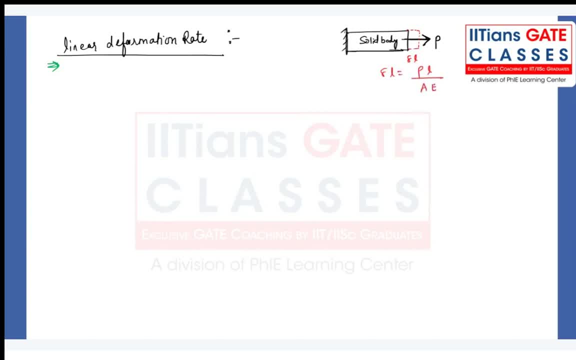 might even we will be calling PL divided by AE. Similarly, in the fluid also there will be some deformations. something like this: Suppose there is a flow field and there is a fluid particles and on any fluid particle layer I am considering the layer. suppose like this: this is my layer of the fluid particle. 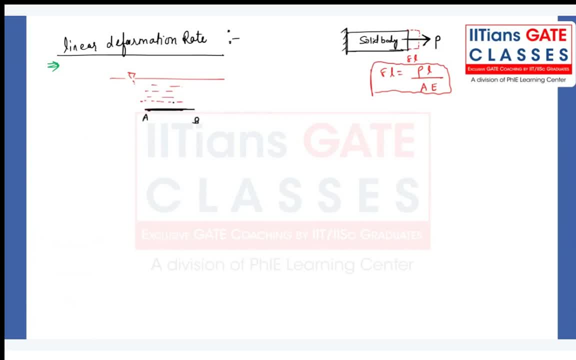 AB, and on that I am applying some kind of shear force to move that fluid AB is a fluid element. Or we can write: fluid element, for example, fluid element. so what we can write, my dear friend, what we can write, the particle- let us say A and B- is there from here to here. 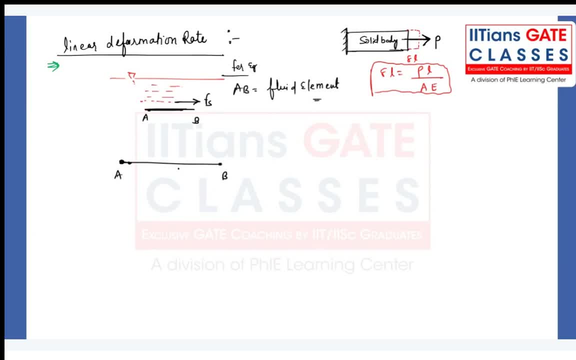 particle A and B which is being connected right means you just assume a thread which is being connecting AB as a fluid particles. now, in a given instant of time, let us say we have the initial gap of dx and the particle A is travelling with u and particle B is travelling. 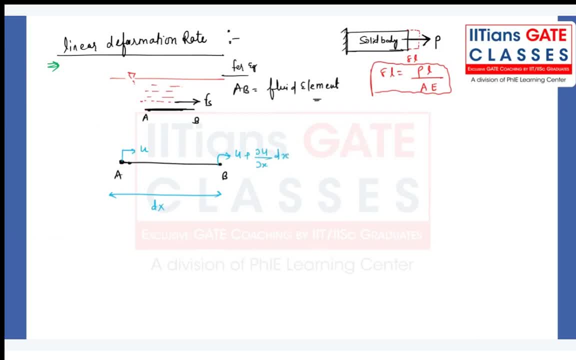 u plus dou u by dou x into dx, for example. right, they are moving with some difference of velocity. then only the deformation will be there. agree with me or not? if they are moving with the same velocity, any deformation will be there. tell me, let us say particle. 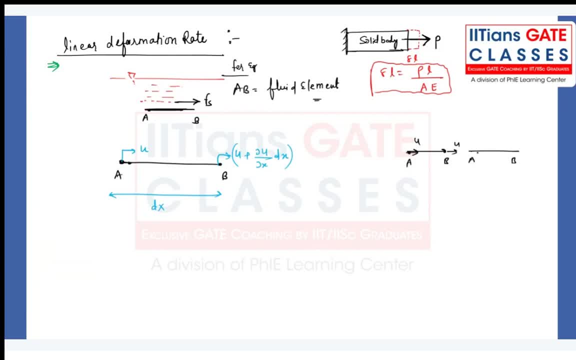 A and B. they are travelling with the same velocity. No deformations will be there, Right, but they will travel with some different velocity. suppose particle A and particle B. particle A is travelling with u and particle B is travelling with 2, u. there will be some. 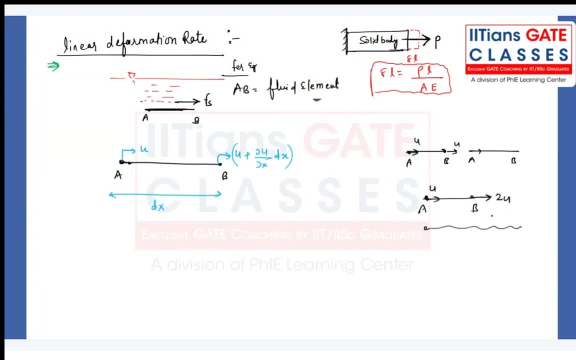 deformations like this in the fluid particles, there will be some deformation with respect to time. right now, let us say after dt time interval, the particle A is has been there here, where here A dash, B dash. 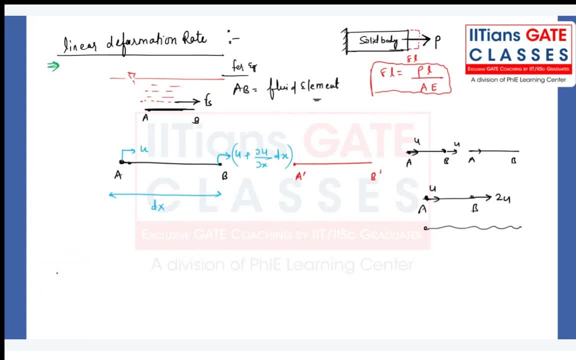 This is my particle which is being stretched. right, you have to assume that it has been stretched. So particle A from here to here, how much of distance it has travelled in a dt amount of time? in dt time the particle A will travel u into dt. and what about particle B? particle. 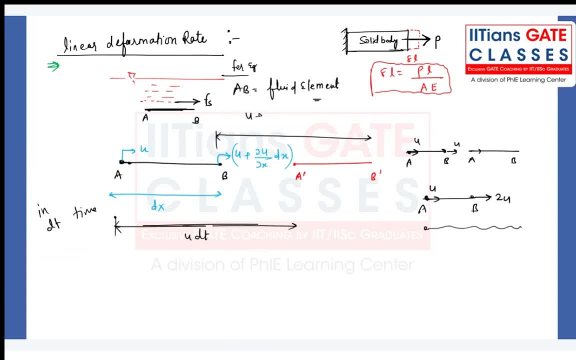 B would have travelled from here to here u plus dou u by dou x into dx, into dt, because we know that. So this is the velocity distance by time, so distance will be velocity into time. so through that segment we are getting this one. 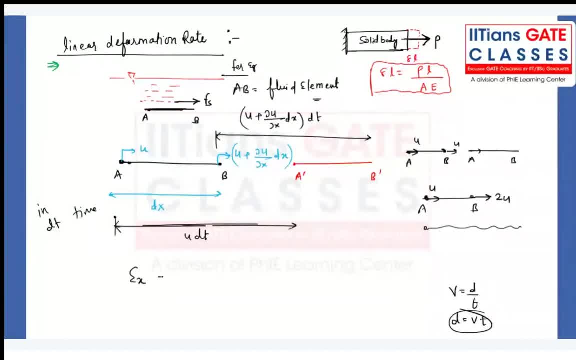 Now, what is the strain rate? right, first of all, note down the strain. what is the linear strain in x direction, as we are focusing our attention in the x directions? so what is the strain in x direction? tell me, guys. 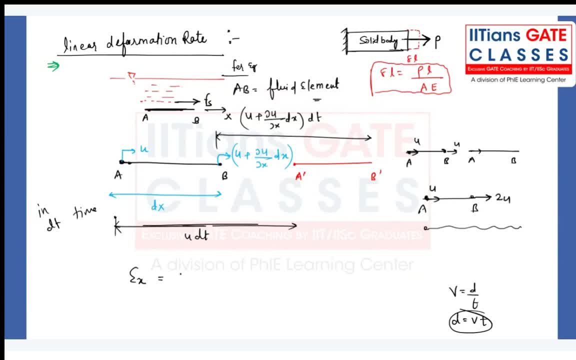 Change in length by original length. Yes, Is it? Yes, can we write like this? in a simple definition you assume AB is like a solid body and now the length has been changed. that is A dash, B dash, you know. so change in length by. 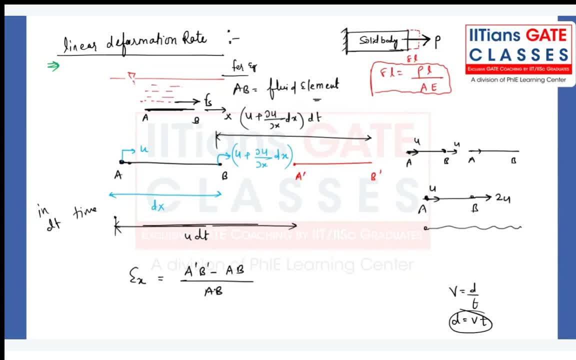 original length. can we write like this? yes, we can write. now tell me AB dash what we can write. can we write AB dash from here to here? A B dash. can we write that is equal to AA dash plus A dash, B dash. check it out. can we write like this: 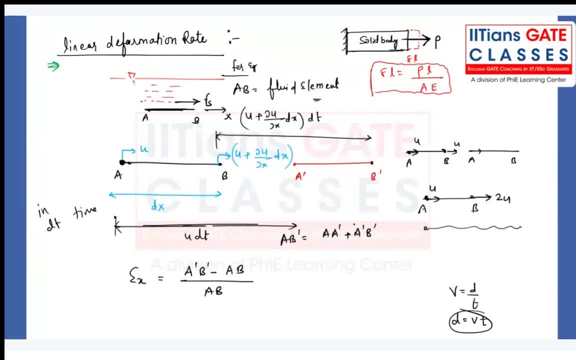 no problem at all. no problem at all. now, whatever the AA dash is there, what we can write, that can also be written as. that can also be written as you understand. that can also be written as AB plus BB dash. see from here to here how we can write the total length. 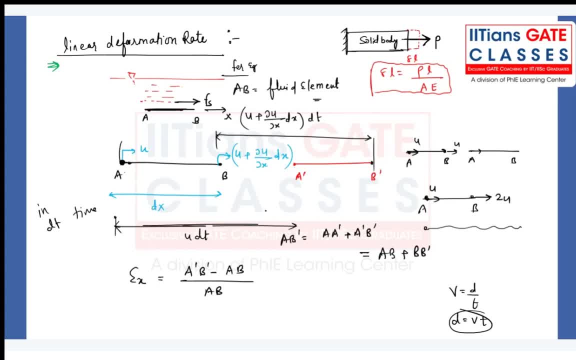 AA dash plus A dash, B dash or AB A dash, B dash plus BB dash. in both the sense we can write like this: now from here I need to calculate A dash, B dash, A dash, B dash minus AB. I can write this to be BB dash minus AA dash- same thing I am writing. 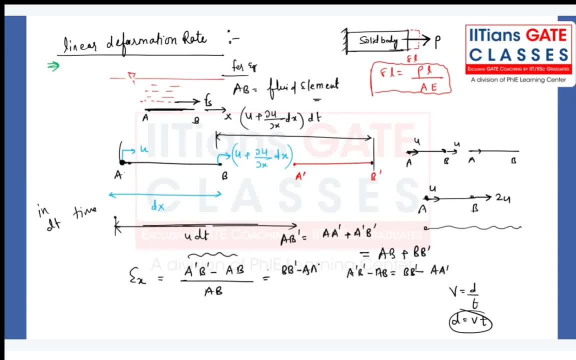 over here: BB dash minus AA dash, divided by AB. so, my dear friend, what we can write further BB dash, what is the BB dash, BB dash, what we can write from here to here, how much of distance it has traveled. u plus dou, u by dou x into dx. 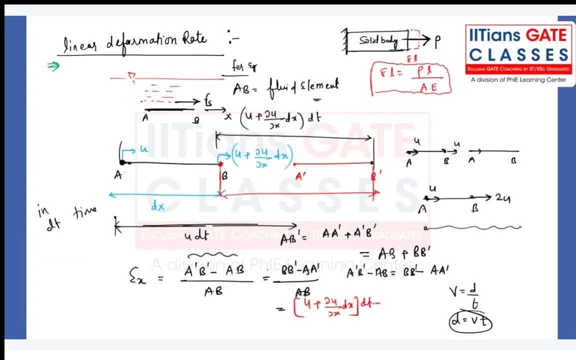 into dt minus AA dash. AA dash is nothing but from here to here, how much of total distance u dt divided by u dt dt I can take out and I can write over here and I can write further dou u by dou x that I can write because u dt will cancel out. 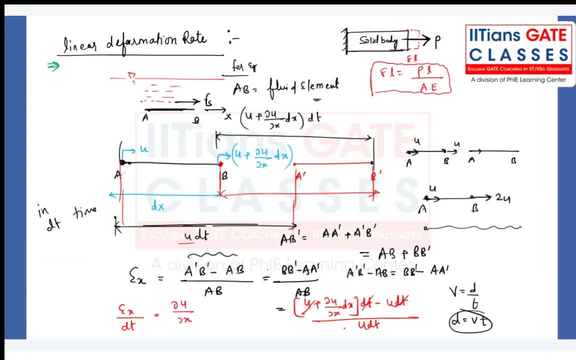 dou u by dou x and d t. d t will also cancel out, right what? we can write: dou u by dou x into dx, into dt, divided by u, dt. this will cancel out we will be getting what? sorry, sorry, here, I will just wait. original length is what. 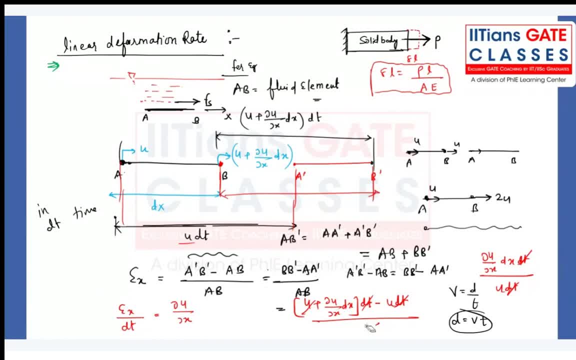 AB. what is the AB we can write? that is not u dt. sorry, that is not u dt, that is dx. getting my point. what is the distance? see, I have written A dash, B dash, minus AA dash, and this can be write: BB dash, AA dash and this is AB. 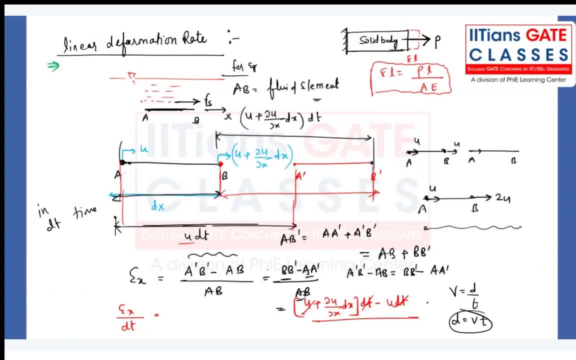 AB is what dx? only right, so I cannot write. this is bx, so this will cancel out. so you will be getting dou u by dou x and one d t is there. that will come to this left side, and this we are calling strain rate. what is that? 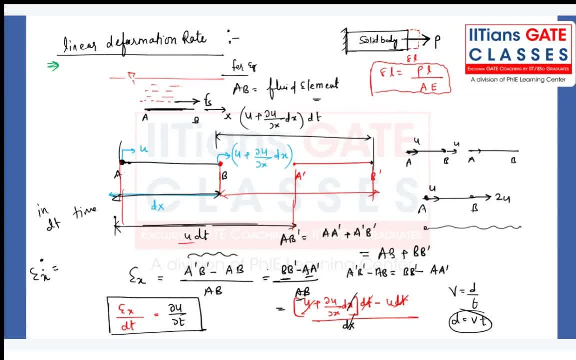 linear strain rate in x direction. linear strain rate in x direction, that is dou u by dou x. make a note of it. if anybody has not understood, let me know in a very similar way. what is the strain rate in the y direction: dou u by dou y. 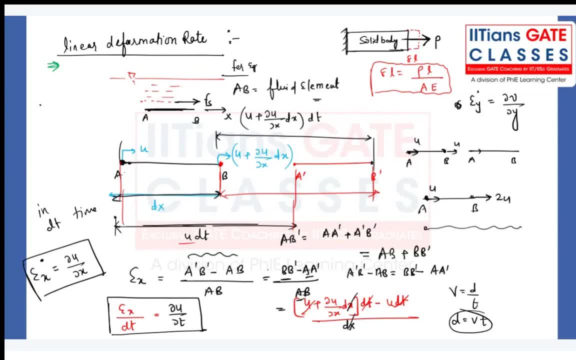 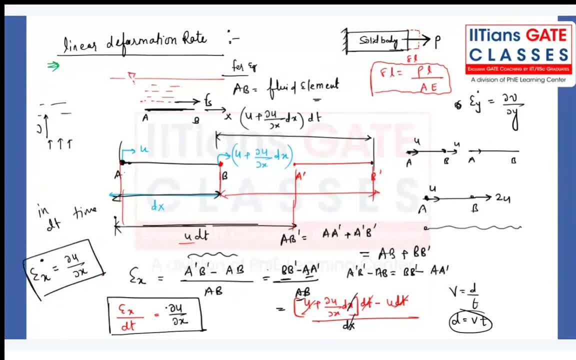 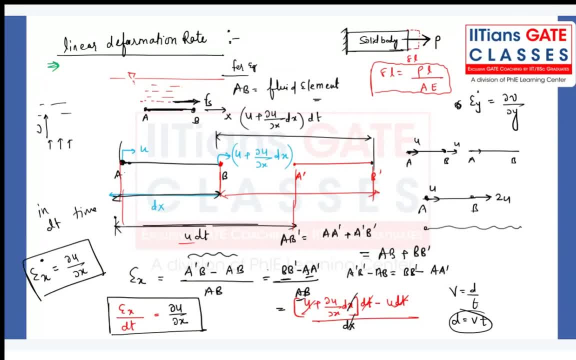 OK, the shear force because particle a, let's suppose here we have some fluid plate which is being booming with some velocity v by the application of force. so this is fs and they will offer fs like here. once it is done, let me know done. can i move to the next one? 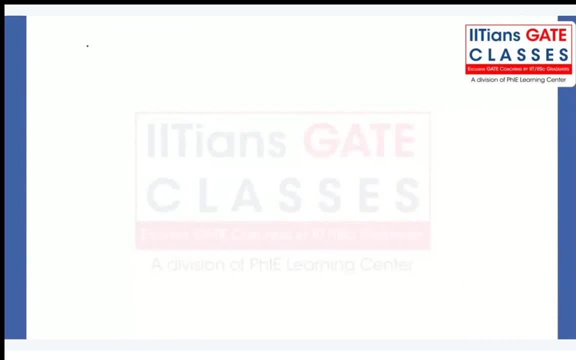 now. so note down the other linear strain rate in y direction. strain in y direction: dou v by dou y. strain in z direction: dou omega by dou z. in x direction: dou v by dou z and dou u by dou x. where uv omega is a component of velocity u. 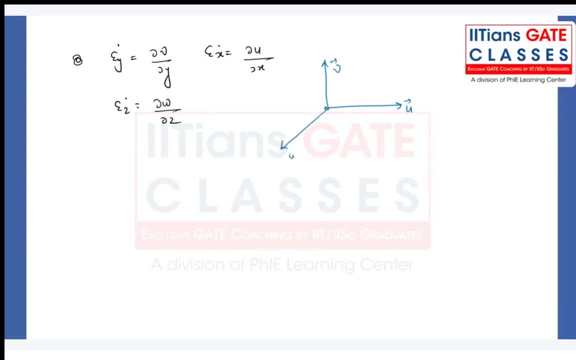 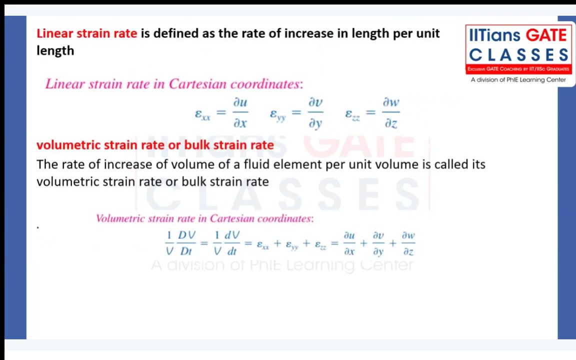 v omega is a component of velocity. u v omega is a component of velocity. u omega in x direction, y direction and z directions and z directions done done. so, as you can see, the linear strain rate is. it is defined as the rate of increase in length per unit time. 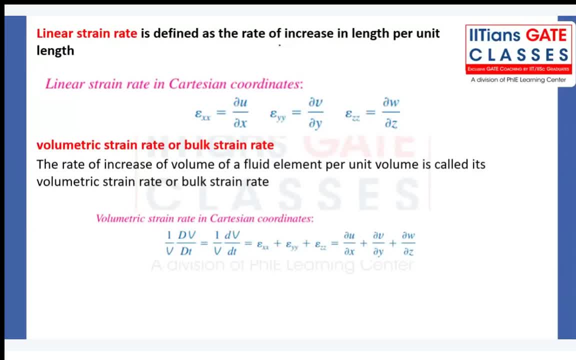 per unit per unit length: the rate of increase in length per unit length. right, that is a linear strain rate in a cartesian, in a particular cartesian system. we can write this way, and if i combine together all the things, then what i will be getting? volumetric strain rate. 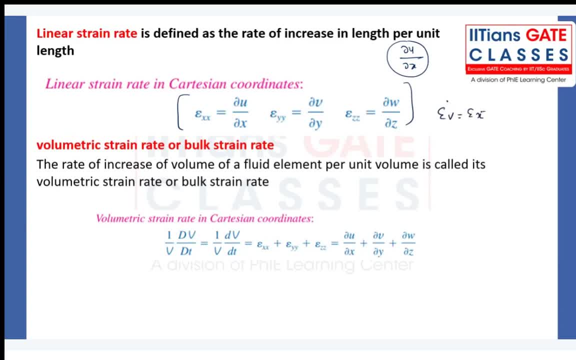 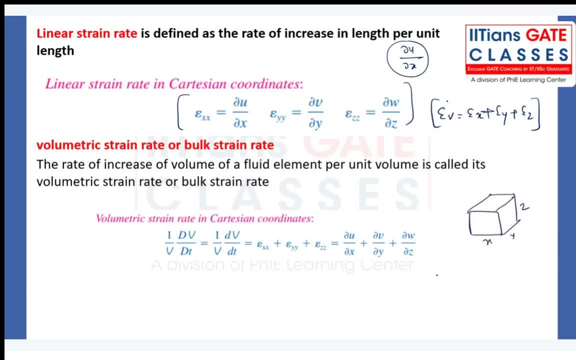 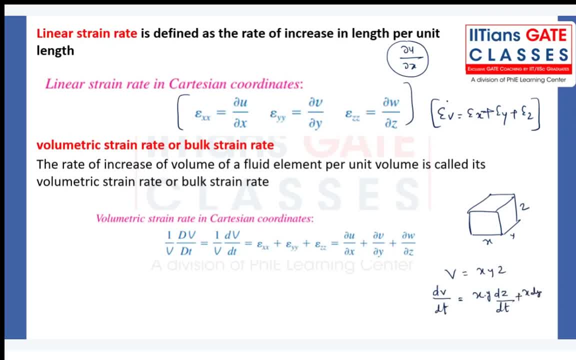 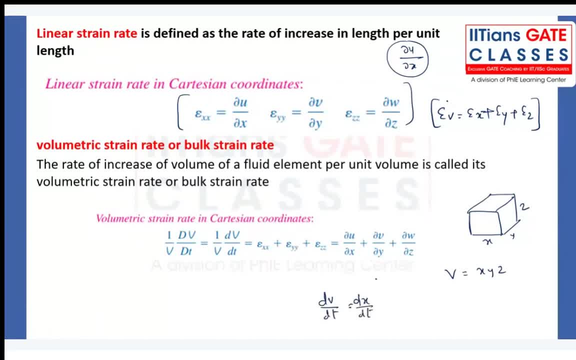 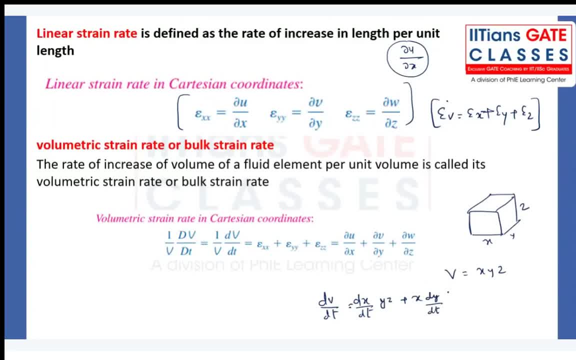 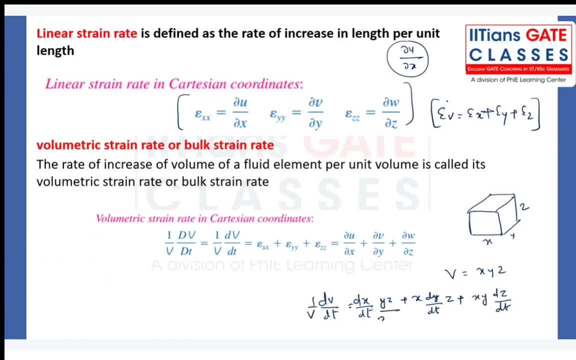 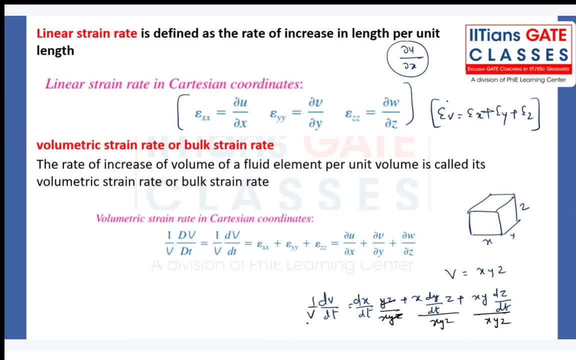 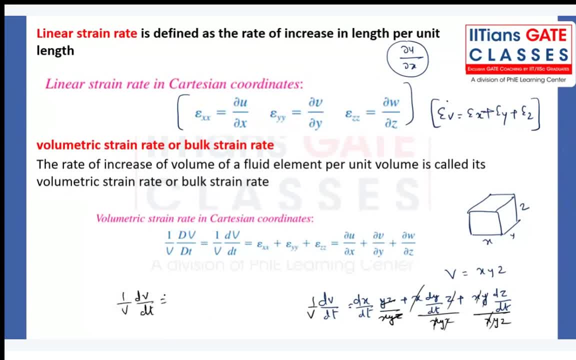 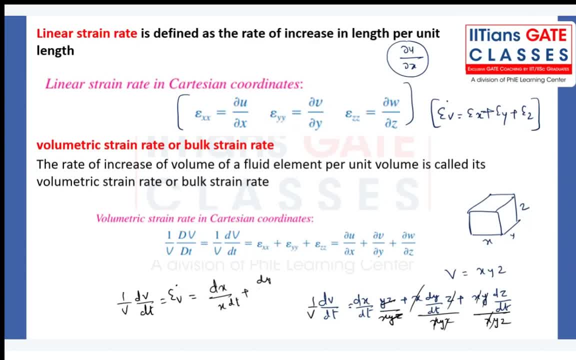 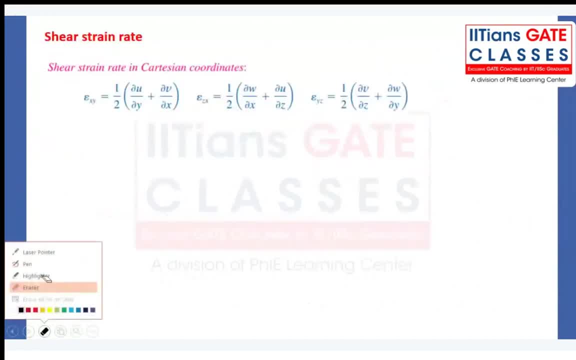 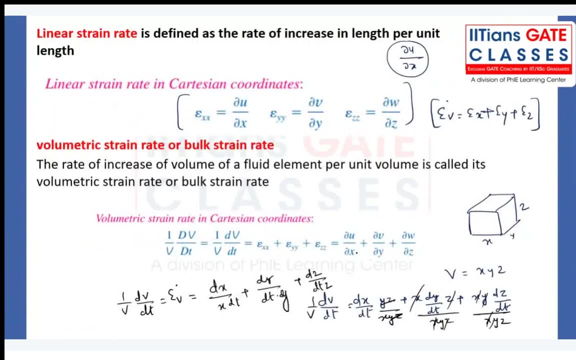 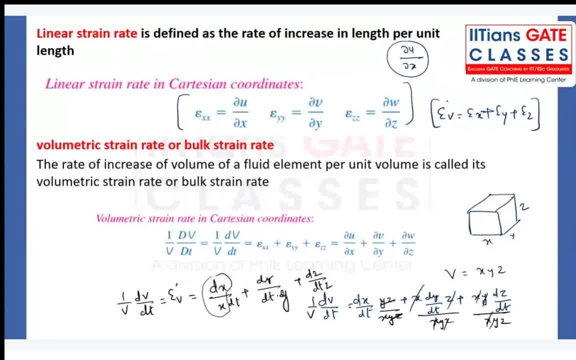 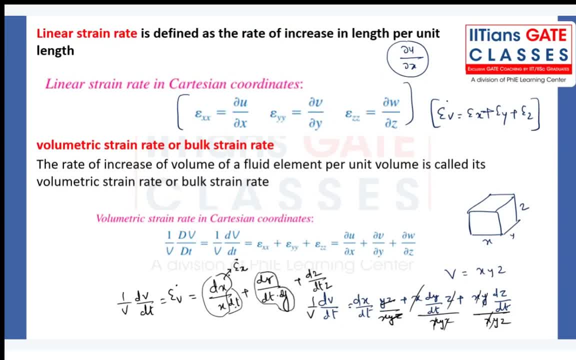 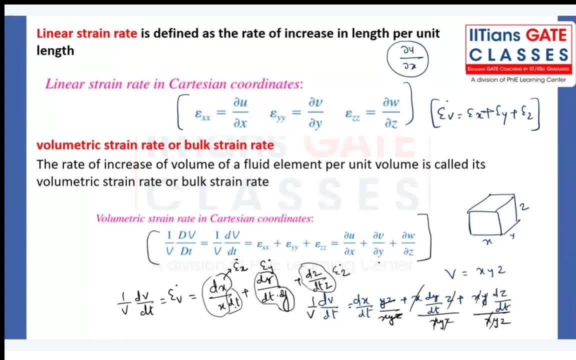 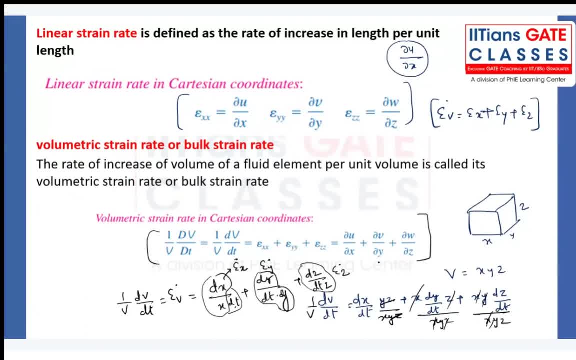 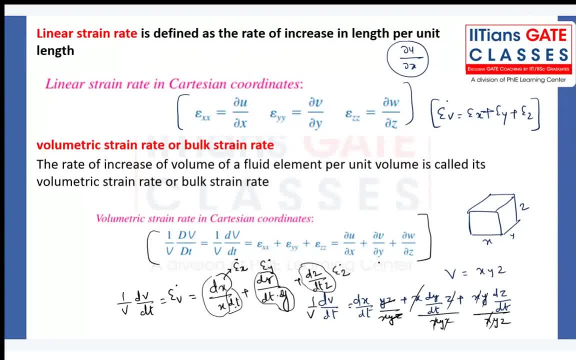 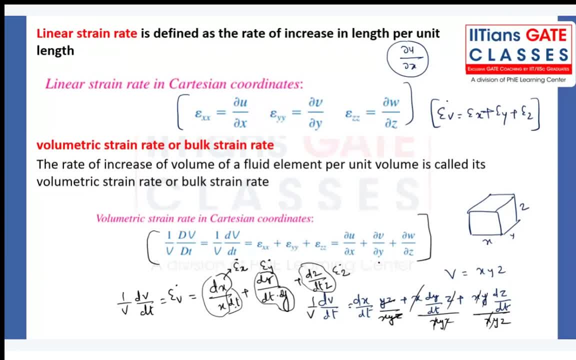 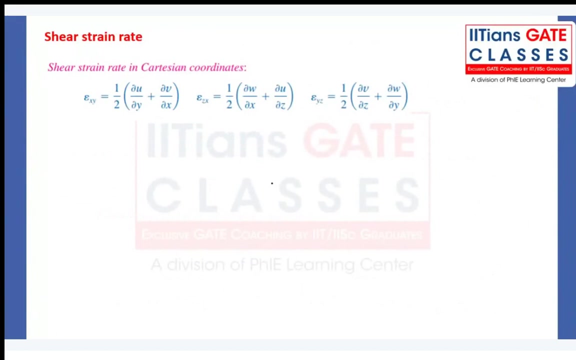 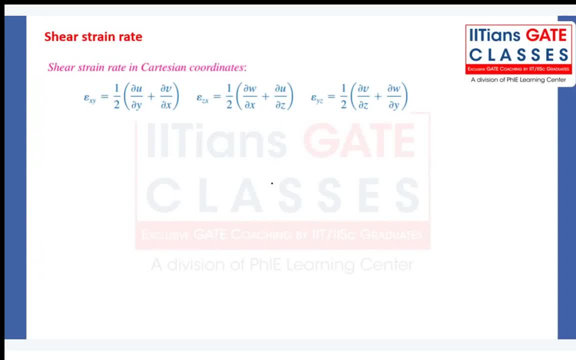 yes, basic elasticity, but per unit time we have to study. suppose any fluid particles are there which is being drive by the plate which is having some velocity. what is going to be happening in that fluid particles, that in the fluid particles, what will happen? the fluid velocity or whatever the particles are? 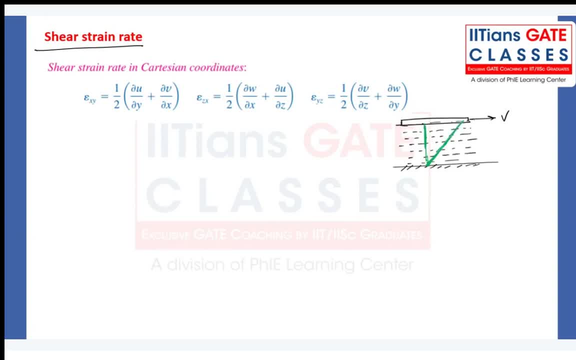 there they will be start deforming. and what is my theta? that is dou v by dou y or whatever the fluid particle is there, we can write that is completely dou u by dou y, and for a linear velocity profile we can write v by h. so what if we are writing over here? this is like: 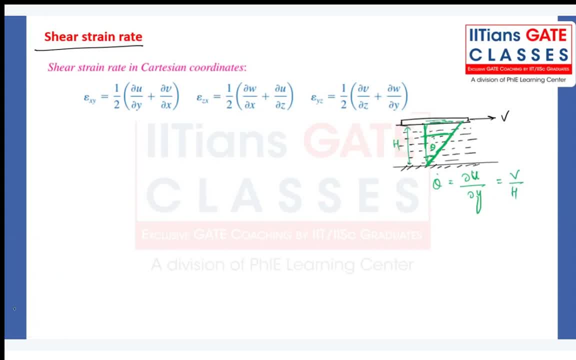 some kind of say deformations which has been happened right for a sale deformation. just note down the definition. what is the meaning of say a deformation rate or say restrain rate which is going to be happening in that fluid particle which has been happened right for a sale deformation? just note. 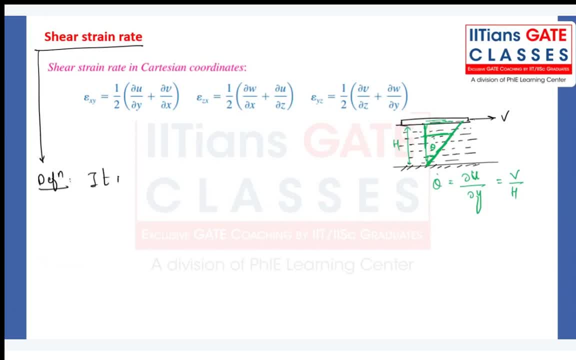 down the definition. what is the meaning of, say, a deformation rate or say restrain rate? it is defined as it is defined as, just like in the solid mechanics, what we have studied about the same strain, in the same manner we have to study over here. it is defined as the 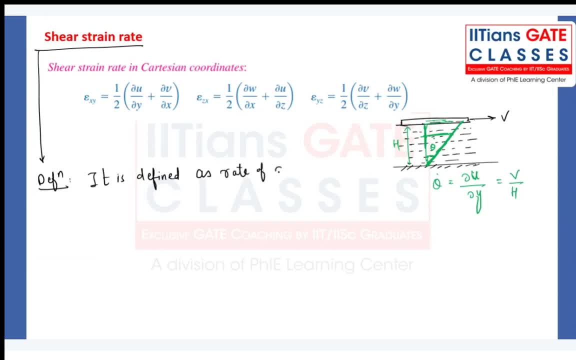 rate of change, of the rate of change of angles between the fluid lines, the rate of change of the fluid lines which we had initially perpendicular. which, fair, we haven't tried at any other stage. initially we haveねぇ, we've had each leaf perpendicular each other. 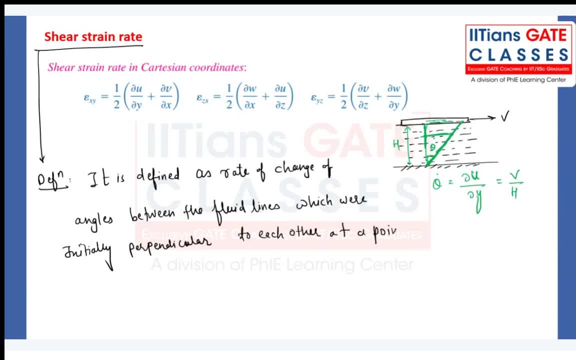 at a point we have you as the rate of change of angles between the fluid lines. that means my defend what you are understanding from this definitions. suppose there is a solid body right. this is a solid body right. it is being fixed at one end. now what I am doing, I am just applying some kind 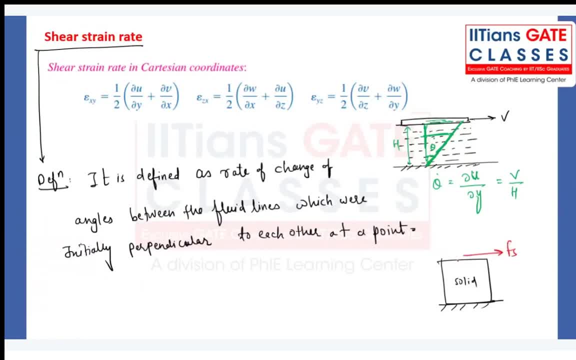 of shear force. what will happen? shear deformation will happen there. how we are defining the rate of shear strain? how we are defining the shear strain? this one, initially, this two line, a, b and c. they were perpendicular to each other. ninety degree was the angle, but now what is my angle? it has been less than that. so what is the definition of the strain rate? 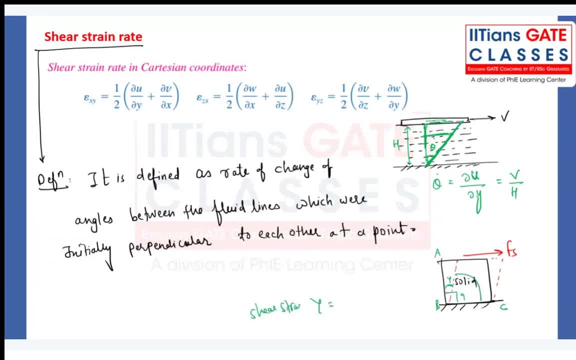 shear strain. tell me, guys, ninety minus this is ninety minus gamma. so what we can write? change of angle between the two perpendicular lines, or two lines which were initially perpendicular. so line a b and b c, initial angle is ninety degree. final angle is what? ninety minus gamma. 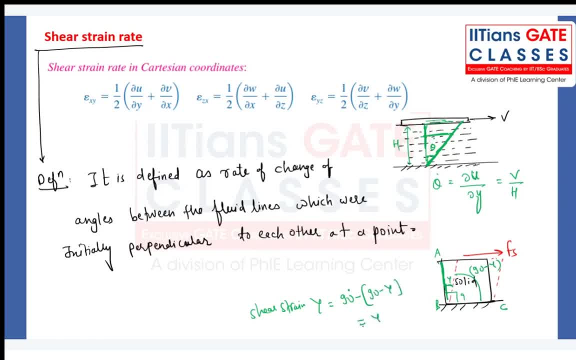 so what we can write gamma- that is my shear strain in a very similar fashion here, also in the fluid, you have to consider two element, a and b, for example. suppose here the two lines are there, let us say a, b and c. so what will be happening, the angle which is being changed. 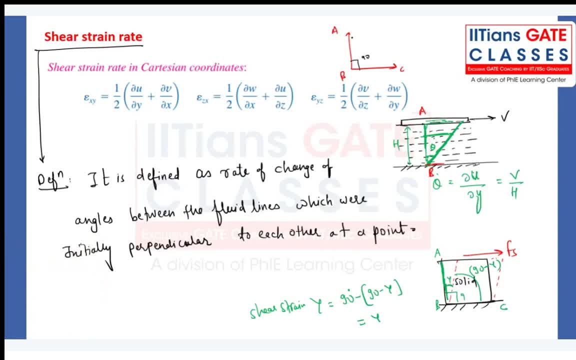 between the two original lines Or the two perpendicular lines, because of the flow. what will happen? the fluid will be start deforming like this. so what we can write this will be b, c, dash. now tell me, guys, what will be the angles. what will be the angles? how much of deformation is there from here? 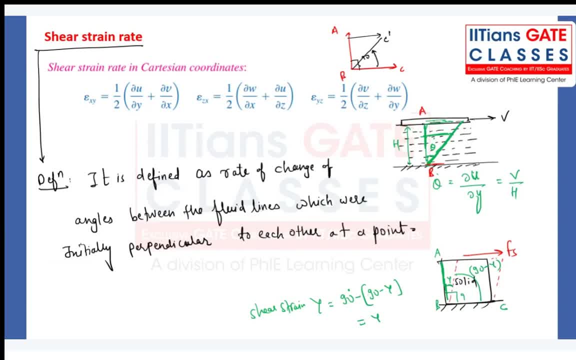 to here, how much of deformation is there between from here to here? or what is the angle from here to here, How much, which angle it has been deformed? what we can write. let's say here we are calling this to be d alpha by dt, d alpha by dt. so what we can write: strain rate in x plane and y plane. 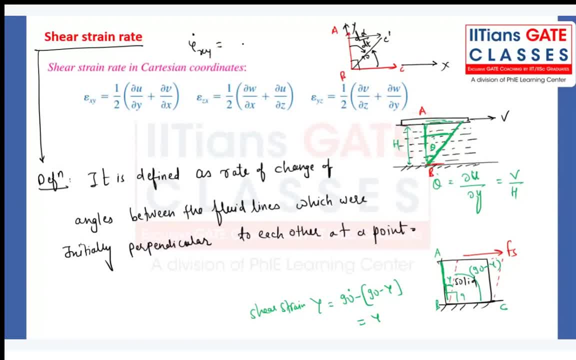 what we can write: gamma x, y, that is equal. to see, guys, i am not here i can directly give the proof, but my intention is to tell you whether you should, whether you are understanding about the topic or not, whether you are feeling about the topic or not. so now here, say strain. 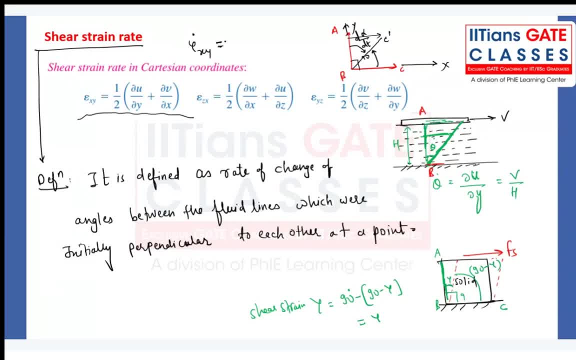 rate in x- y plane will be what change in angle 90 degree now, what is the final angle between these two lines? so what about the final angles between the two, these two lines? yes, if i just assume my fluid particle, which is being traveling like this now say this is taking place in angle a minus our initial value. it has been set to be equal. 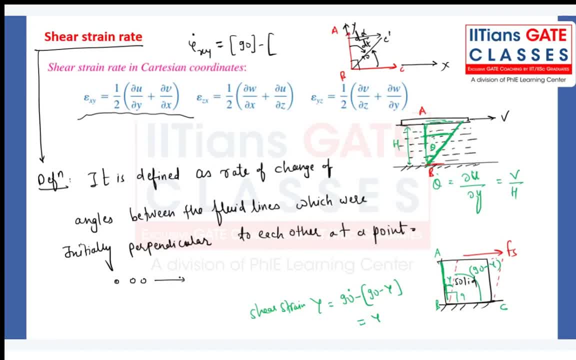 to 0 and so what is the final storms left? whether theny z. this will be our initial damn ajustment. so our expectation is the final 5000: go beyond 1 half of current, so basically go to below point. the next y here plus y here, because we will write z, that will be e minus, z minus. 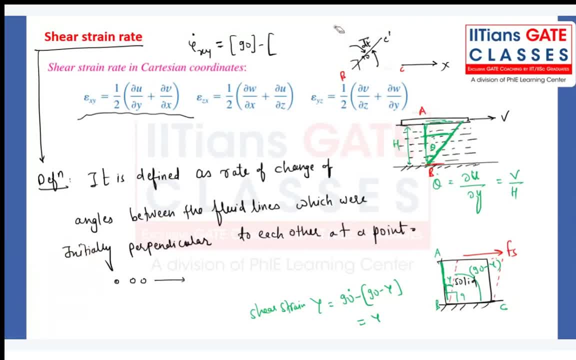 z muốn put equal hp now it is devressive. we are doing the two lines which we have considered. you know that we have to look at very carefully. this is the line a b. this is the b c right when the fluid particle is traveling like 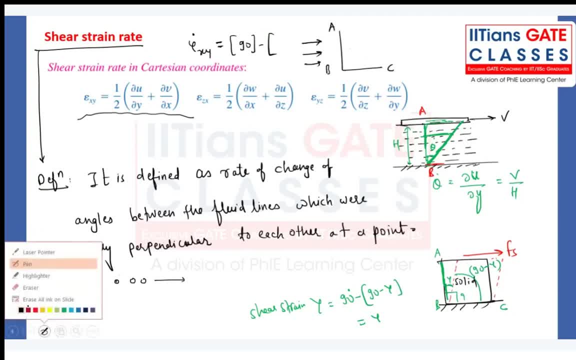 this. a b line will deform. right, get it by point, all of you. a b line will be start deforming like this. get it by point. so let's say: this is my d, alpha by dt, and this line will become what? a b line will become a a dash, b, dash. now tell me what is the final angle between? 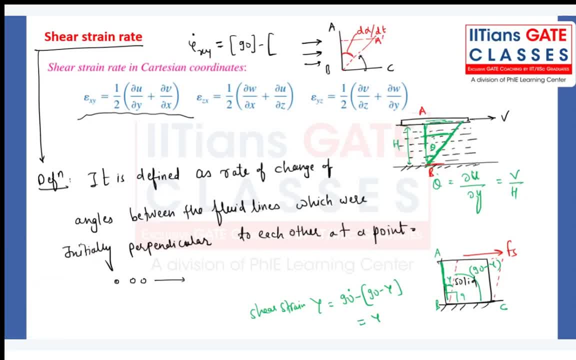 these two lines. the final angle between these two lines will be 90 minus d alpha by dt right. so in this case, what we can write? 90 initial angle. what is the final angle between these two lines? 90 minus alpha dot. so what is the strain rate in x- y plane alpha dot will be: 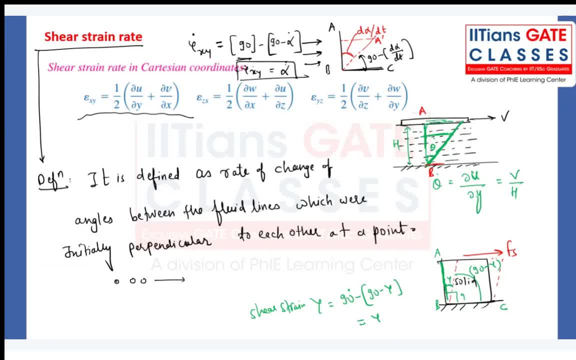 my alpha dot will be my strain rate in x- y plane. so this is one of the very, very important thing. please make a note of it. and how to find alpha dot. how to find the alpha dot? that is the next question. how to find that particular alpha dot. that is a very simple. we have already seen our proof that. 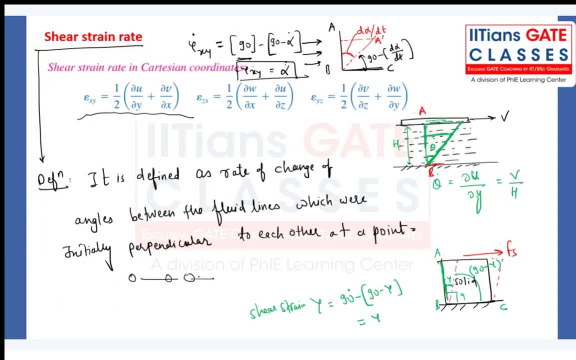 proof of that in the first chapter, particle, which is being traveling, and the lower particle, which will be travel with some lower velocity. let's say it has been traveling what we call from here to here. it is being traveling at a distance d y: it is traveling at a distance. 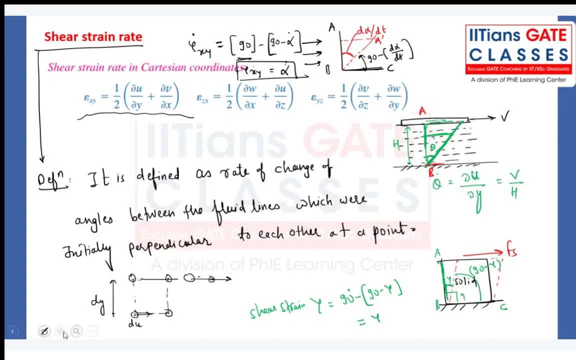 let's say du udt, it has been traveling with the velocity u and this has been traveling with some velocity u plus dou u, by dou y into dy. so this distance will be same udt, but this extra distance which is being traveled by the particle from here to here, or let me just 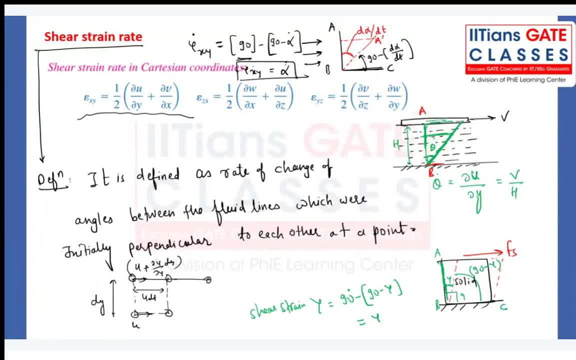 write from here to here, this will be dou u by dou y into dy, into dt. so what is my this? alpha dot, alpha dot, i can directly, or d alpha angle. i can write tan alpha. alpha is very, very small. we can write tan alpha is almost equal to d alpha and that is my this distance. 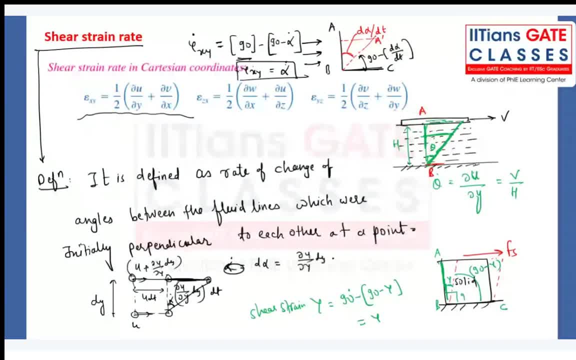 that is dou u by dou y into dy, into dt. divided by uh, what we can write dy. this will cancel out. so d alpha by dt will be my dou u by dou y and that is what we are getting from here also now. so this is what you are getting, the strain rate in x direction, but why it is extra. 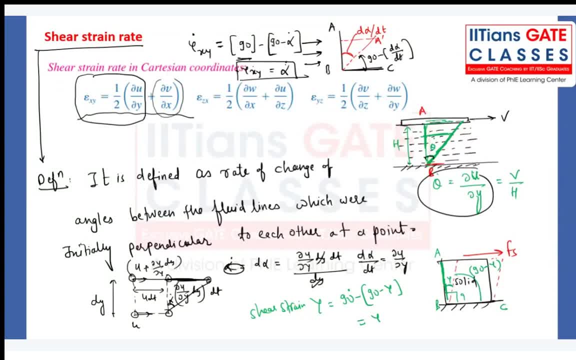 term is there, extra term is there when you have flow in this direction, when you have flow like this also. so both the lines will be start deforming like this: a, a dash and my c will be traveled to- sorry, my c will travel to c dash. so here it will deform by alpha dot, here it will deform. 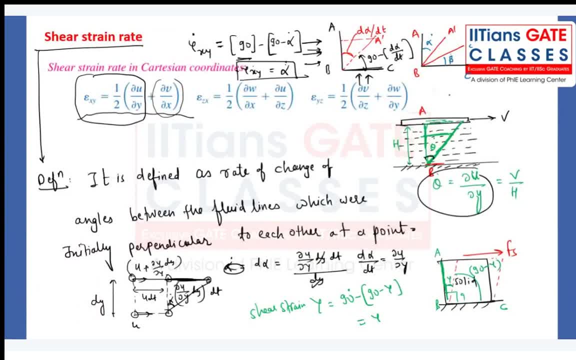 by beta dot, alpha dot. we know that dou u by dou y and beta dot will be dou u by dou x. so together, you know, initial angle will be 90 degree. how we are getting this formula. how we are getting this formula. let me prove that we are getting this formula as epsilon. 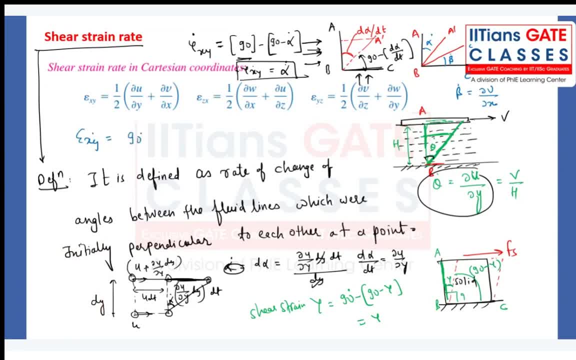 x y dot. initial angle: 90 degree. final angle is: what final angle is this one between these two lines? 90 minus alpha y dot. alpha dot plus beta dot. alpha dot plus beta dot. so finally, what is that alpha dot plus beta dot? similarly for other planes. you please note down the formulas. 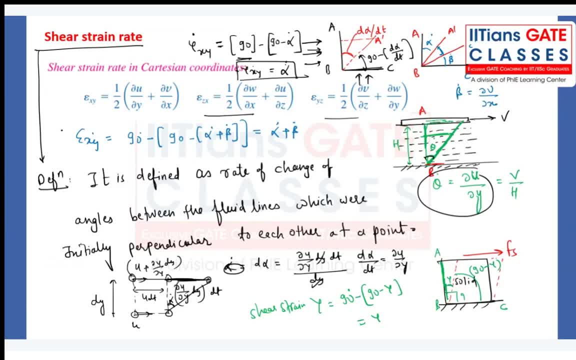 now why half is coming. that is a shear strain rate formula, only for shear strain rate. remember that is a. this thing will be clear when we discuss in the solid mechanics about the strain matrix right as of now. you might be thinking, sir, it should be only alpha dot plus beta dot. that is the 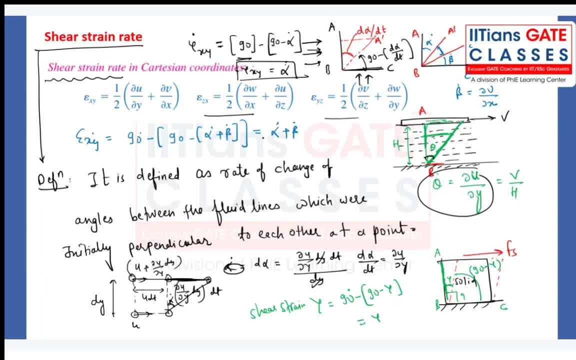 formula for angular deformation rate. of course, both the terms are same same. i will be telling you the differences. just make a note of it. epsilon xy or gamma xy dot, both are same meaning. it's a very easy to remember: x, y is there, u, v will be there, and interchange the y and x. z, x is there. which component will be there? 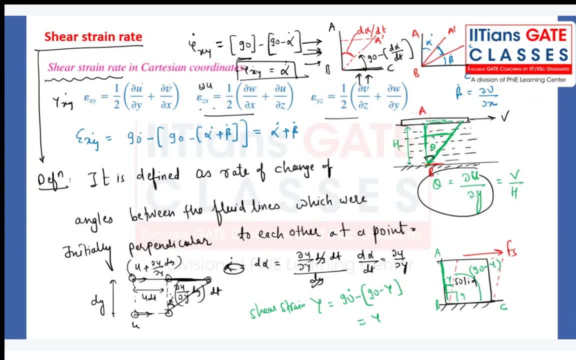 omega and u will be there. interchange omega with the x. interchange u with the what z? that is a short part to remember. now, once it is done, let me know. see for a linear deformation by different. you know you can have the linear deformation also, right, if i show you a very general picture where we can have the both right. see for a. 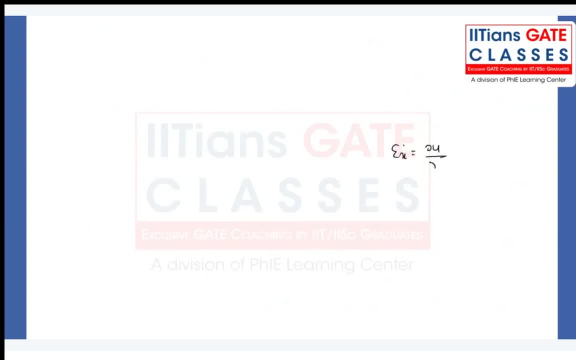 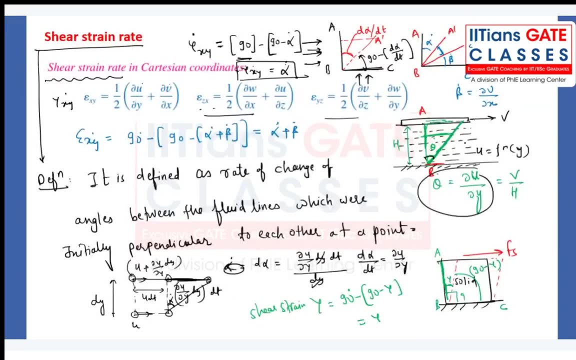 linear strain rate. you should have dou u by dou x, right? but in this picture you know that u is only the function of y. so what is the linear strain rate? especially in this case, dou u by dou x will be zero. getting my point? you can have the both shear deformation and linear strain rate. both you can have when. 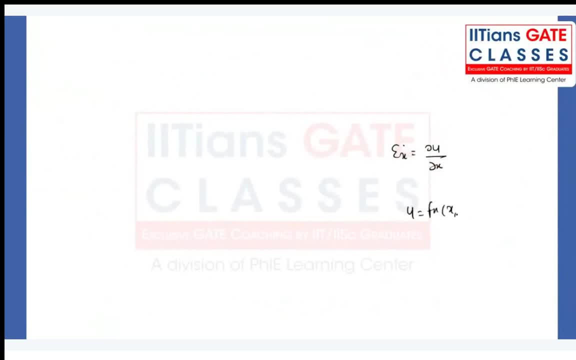 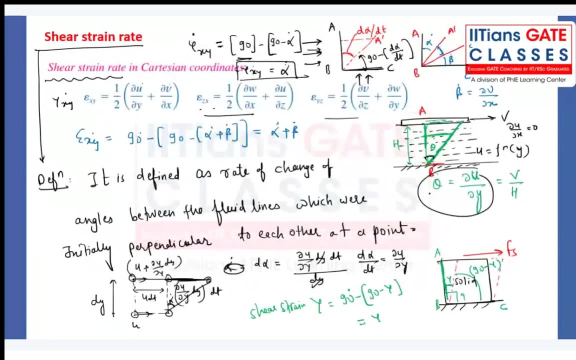 u is a function of both x and y. getting my point correct? correct, but that is the average. what you are mentioning, you know, average of angular strain. that is the definition of the angular velocity, that's the some kind of definition which we give for a rotation. one will be the with the sign convention, like counter clockwise positive. 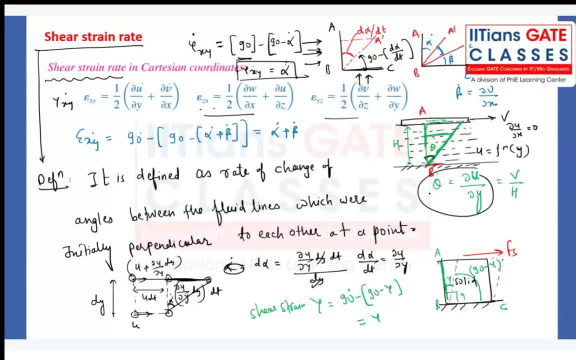 anti-clockwise, clockwise negative, kind of things. once it is done, let me know. okay, so let me know if you have any other questions. if you have any other questions, i will be happy to answer them. i will be happy to answer them if you have any other questions. 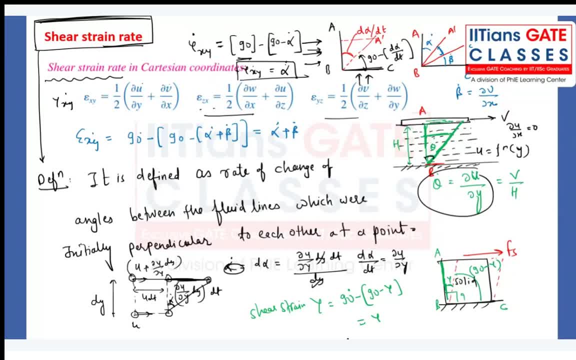 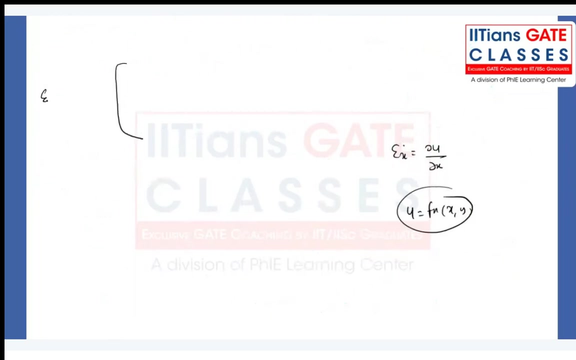 thank you. now, once it is done, let me know the shear strain rate. y half is there, because when you write the, you know matrix, you know strain matrix. you will find epsilon xx, and then you will find my dear friend epsilon xy, epsilon xz, something like this, this epsilon xy- actually we are writing gamma xy. 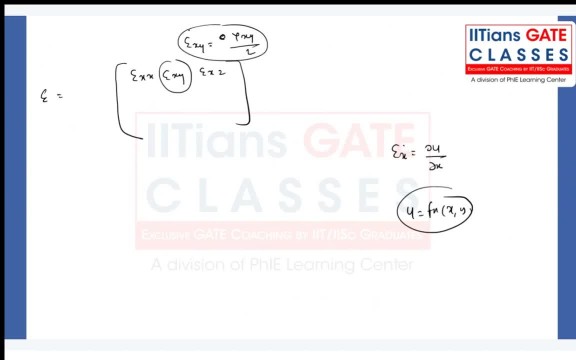 two, something like this. that's why, for this purpose, half is coming: gamma xy. we know that gamma xy alpha dot plus beta dot, but while writing in a matrix form it is coming to. that's why we are writing by two. but that is true when you write, uh, the when the matrix has been given in the question. 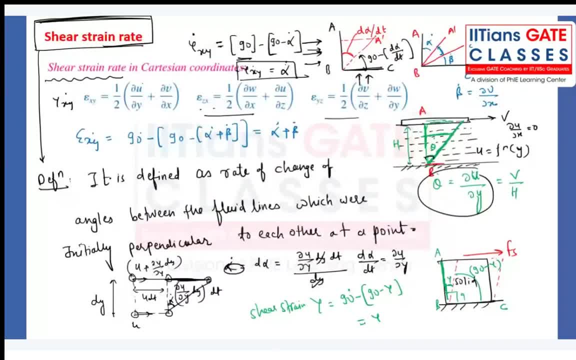 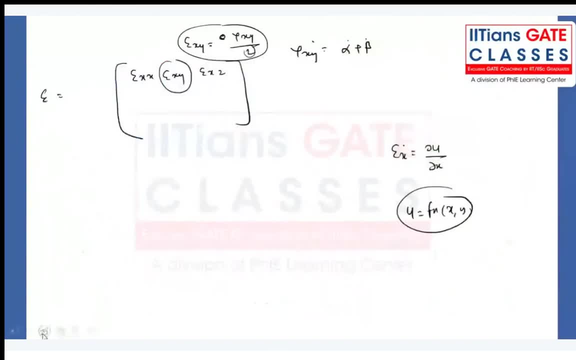 right, but sometimes it is the only formula which is being given in the single and symbol book, that is with the half. but note down the other formulas. what i want to tell you, note down other formulas say, when they mention in the problem, say a deformation rate, only say a deformation rate. 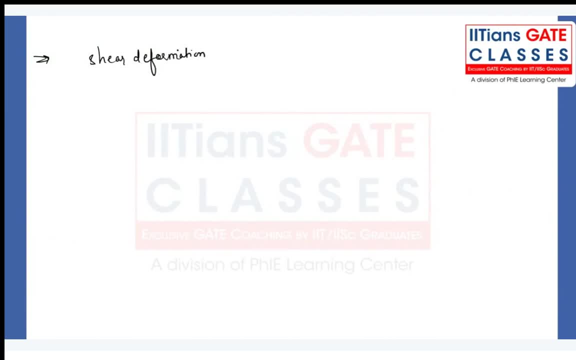 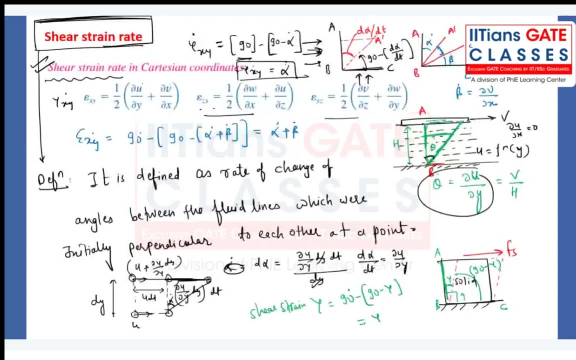 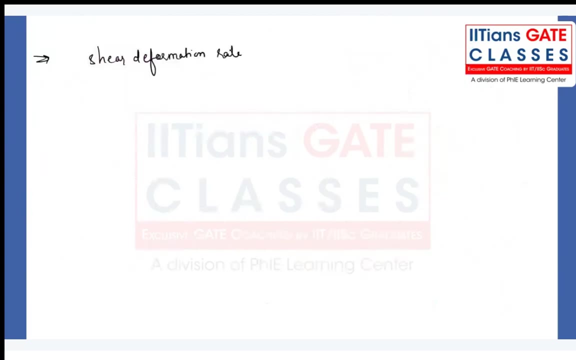 rotation c based on the fluid directions. how the fluid direction is there, in which direction is there? based on that, the rotations would be there. right, say, a deformation rate- we also call it angular deformation rate. this thing we can write. it is the only deformation rate. that's it. that is not the same strain rate. 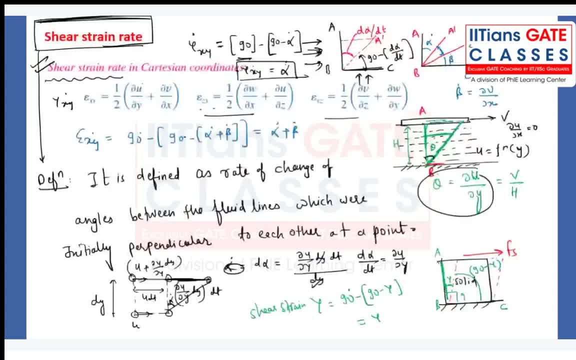 right share strain. this term strain is basically taken from the strength of material. that's why, to respect that subject in uh and they have mentioned very clearly- to certify some condition, tensorial conditions- i will discuss. i am not discussing over here. that's why some half is coming, because 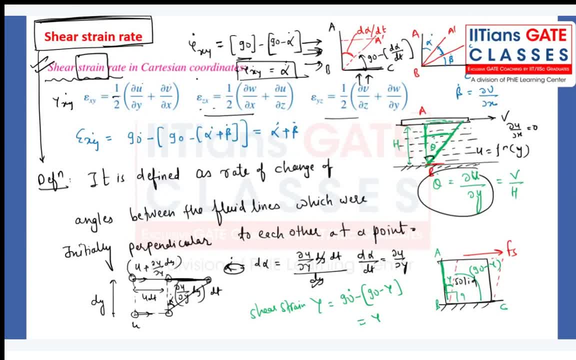 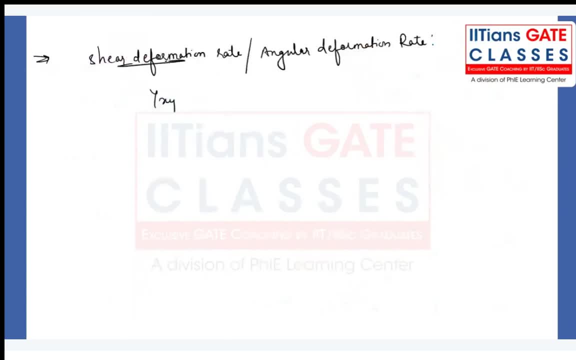 i, i, i said the matrix itself has its own jejgo creator matrix, which i will uh show you as well. come up. i will brief you a little bit on matrix. close, cause we have mentioned only deformations and that's, is it no un beetroot? that is why half is coming over here. i just now shown you, uh, how half is coming in the matrix itself. 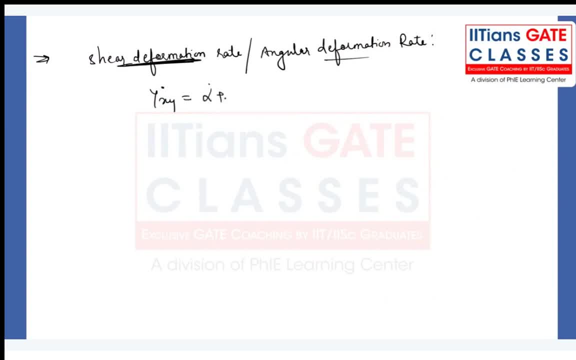 is, half is there. that's why half is coming over here. but when they mention only deformation, that's it. no strand word has been mentioned. then directly note down: osterone, gamma, x, y dot will be alpha dot plus beaten, that is. so you buy do y plus dot by 2 x. 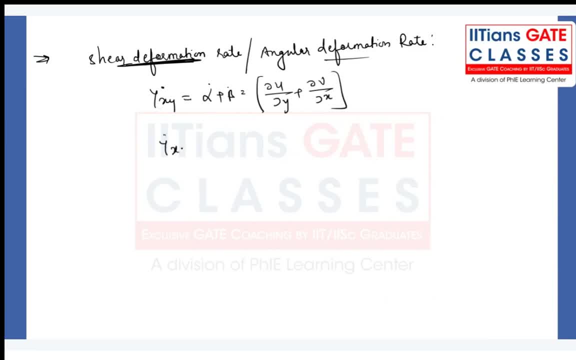 Similarly gamma xz will be. you can write dou u by dou z plus dou omega by dou x. gamma yz will be. sorry, this can be written as see, because sometimes you follow NPTEL assignment, you know you will find, say deformation rate. sometimes you will find say strain rate. 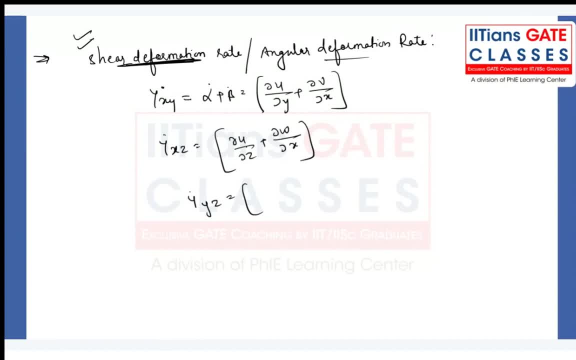 So to avoid that confusion you should please make a note of it: dou u by dou z, plus dou omega by dou y. Once it is done, let me know Done. On the basis of that, we will try to see some of the problem. 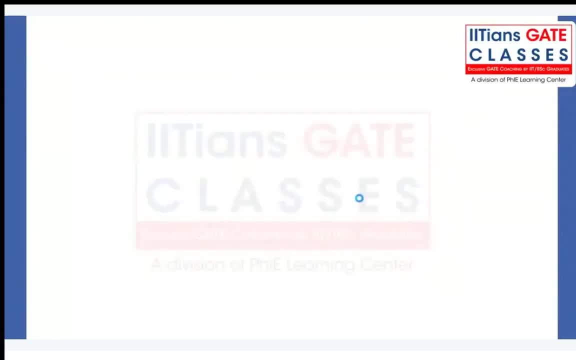 Yes. So when you see in XC paper in 2014, they asked rate of angular deformation at a location of this one, They have given the velocity field x square. y, v is minus y square. If they have not asked anything about, the say, strain rate, then what will be the answer? 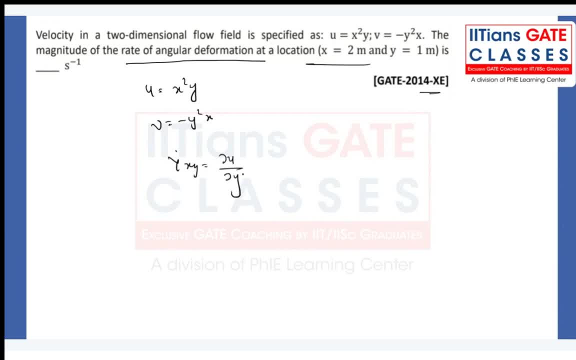 Simply, we need to find dou u by dou y plus dou v by dou x, Dou u by dou y. what will be there? X square, dou v by dou x minus y square, So that is nothing but x square minus y square. that will be 2 square minus 1, that is 3 unit. 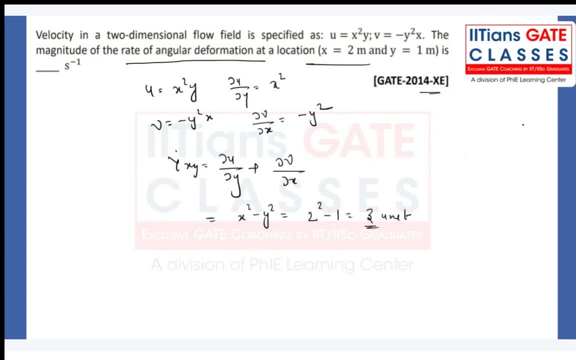 No sales strain rate: half. that is correct because that is given in the single and that is being already verified, So no need to worry about that. No, no, that is being specifically- I shown you the proof right, there is no need to. 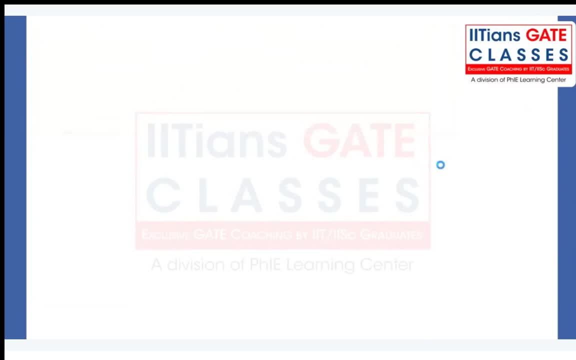 put half because I told you the fluid deformation which is being there, right directly from here to here, flow velocity which is being there, and I shown you the proof: alpha dot, this is beta dot. That is simply the deformation which are happening, right, we are not bothering about, we have. 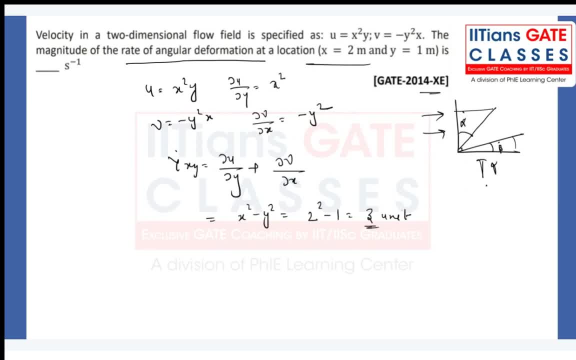 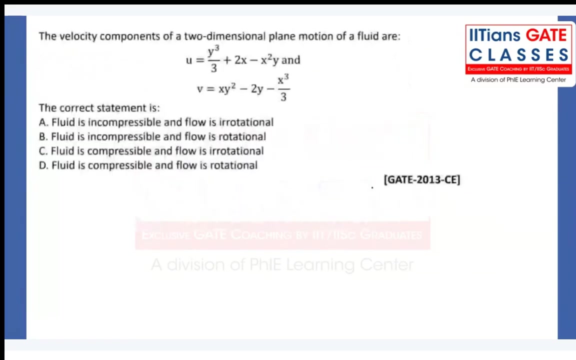 not defined like that- Initial angle minus final angle, initial angle minus final angle- but here in the fluid mechanics it is dot. So that is the signal that is being generated. I am going to put the all Done. Can I move to the next one? 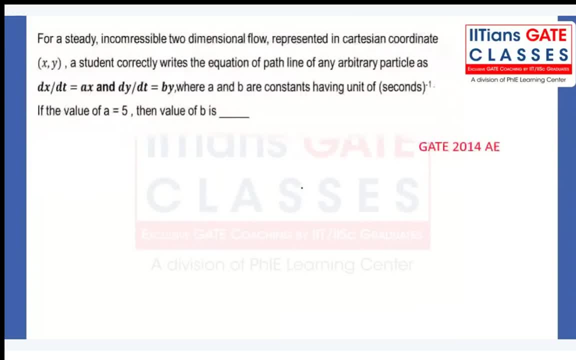 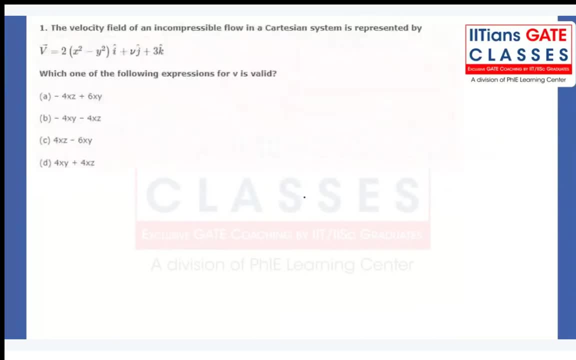 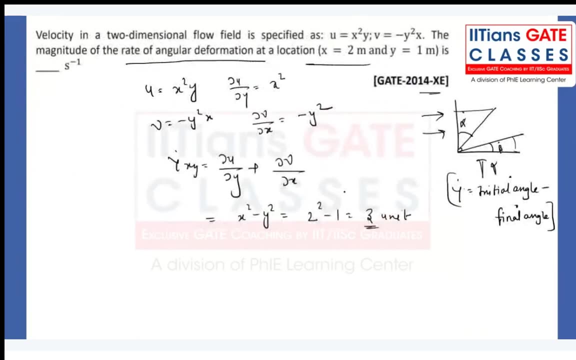 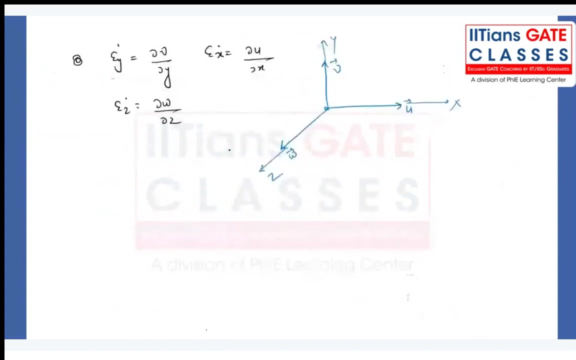 All of you have noted down. Make a note of it. Is it done Now here? just note down one more term. is there rotations? Note down Rotations. We call that to be okay. note down angular velocity. angular velocity, it is just kind. 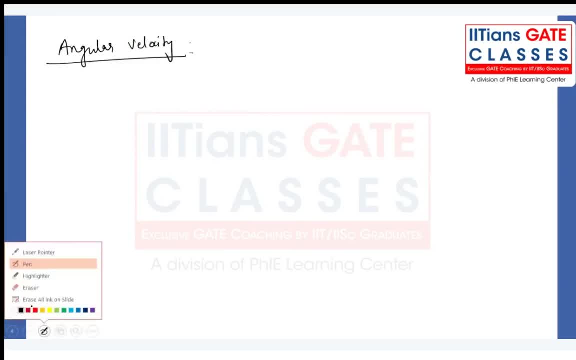 of a very similar expression. Another expression is there, just like what we have studied, but with the minus sign. Now note down, it is defined as it is defined: as average rate of average, average rate of rotation of two initially perpendicular lines. 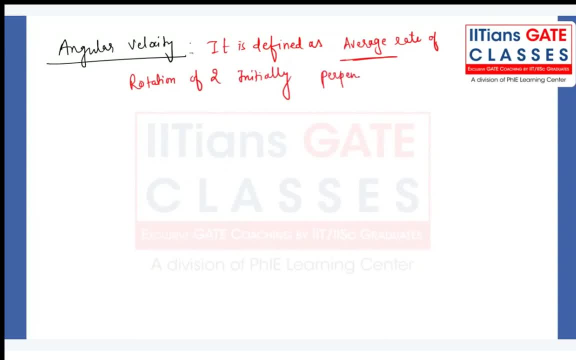 Two initially perpendicular lines that intersects at a point, That intersect at a particular point. That means, two lines are there, A and B, C. they will be start rotating. let us say, for example: Now it has been rotated in this direction. it has been rotated in this direction by: 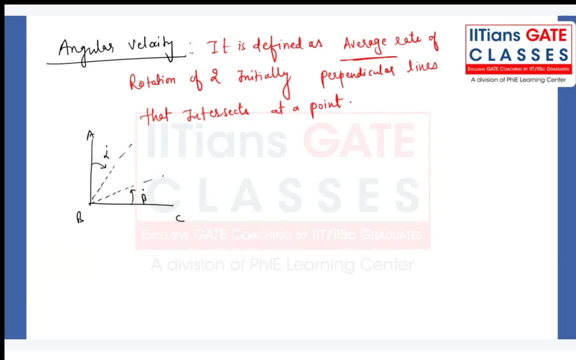 the amount alpha dot by the amount beta dot, right? So what is we are writing over here that clockwise rotation? we are assuming that to be negative. So d, alpha by dt, that is alpha dot. we are writing minus dou u by dou y. 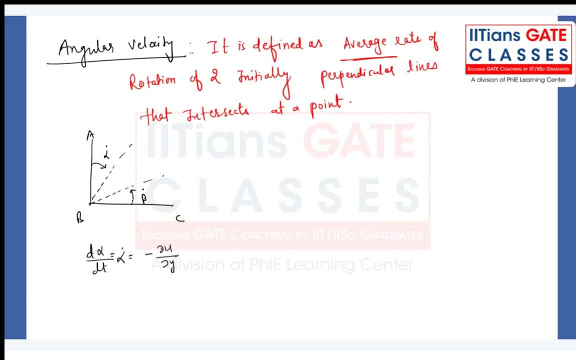 It is not coming just because of the flow directions and all. it is coming via sign convention, right? What is the sign convention? What is the sin convention? What is the sin convention? What is the what they have written? Average rate of rotation. that means omega xy in xy plane. if I want to see in, by which? 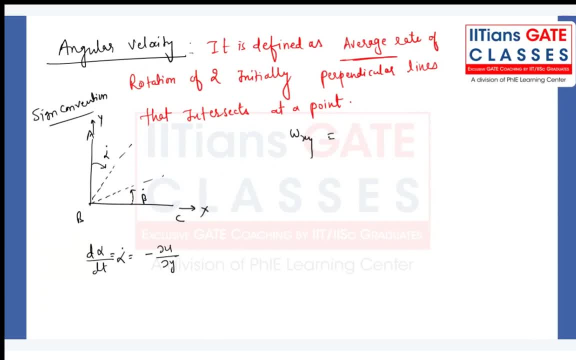 amount they have been rotated. So if I want to find, I will do the half alpha dot plus beta dot divided by 2.. But but here good point is that we have to consider with the sign: What is that sign? 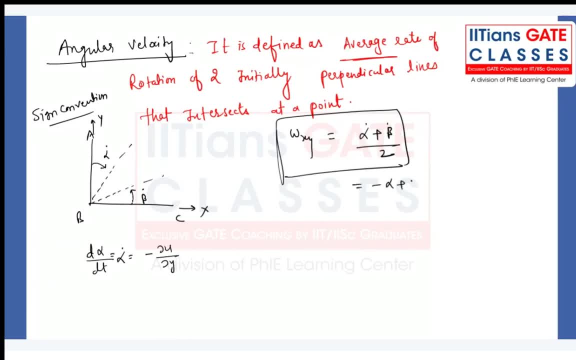 Alpha is what negative sign and beta is what positive sign divided by 2.. So what we can write, What we can write, Beta dot. we know that dou u by dou x minus dou u by dou y and half of that, that is my. 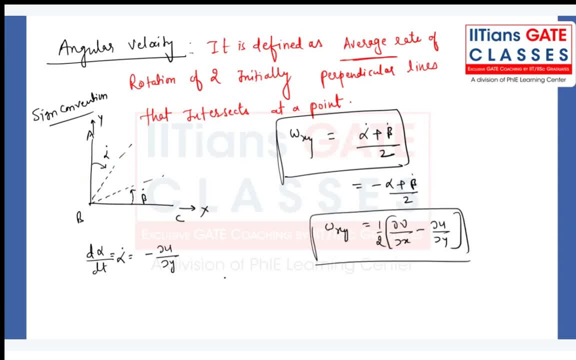 omega xy, Beta, dot. we know that d, beta by dt, yeah, clockwise, negative, anticlockwise. that is positive Like this, so make a note of it. Similarly, my different omega, What we can write, Other things. 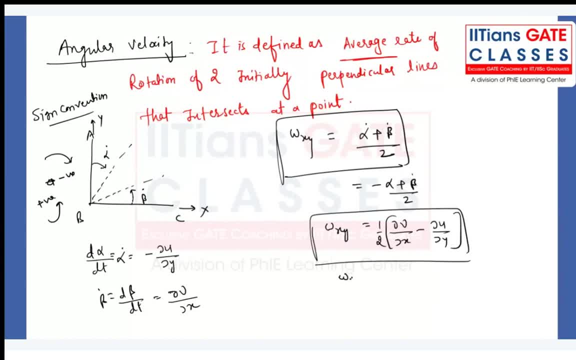 Omega yz, omega yz. you can write half of: see, xy is there. you please write xy and z like this: So xy is there, xy is there now. whatever the x is there. opposite of that we will. 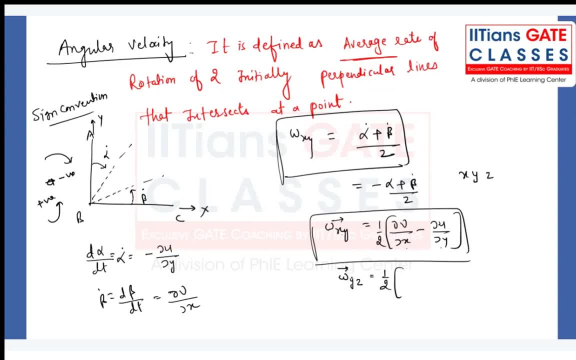 be coming and opposite of y, you will be coming. Similarly, yz, note down the yz like this, with the y which is there- see, there is a yz- means there is no point of discussion about discussing about yz. 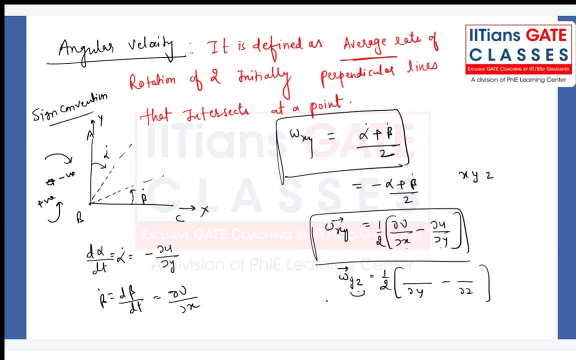 There is no point of discussion about yz. There is no point of discussion about yz. There is no point of discussion about yz. We are discussing about what You. There will be v, there will be omega, but interchange right. 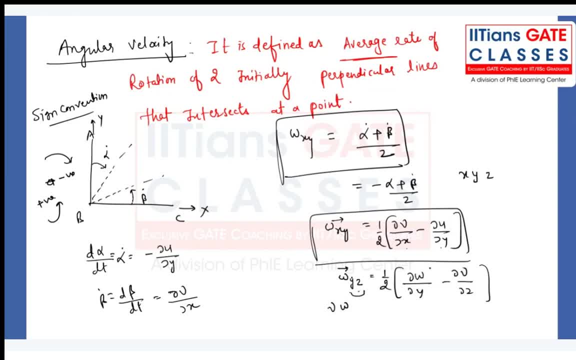 Please remember this, you will never forget z. x will be half of put z, put x in a same sequence, In the same sequence, right, But with the z, which one will be coming, You will be coming. With the x, omega will be coming. 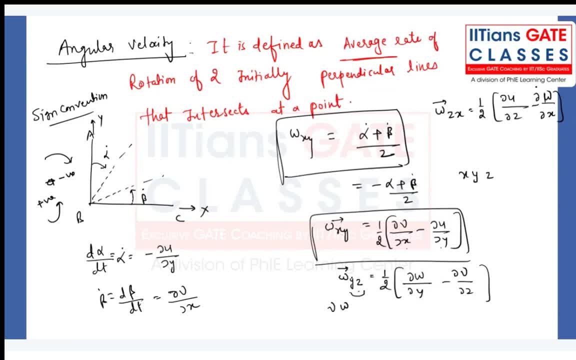 That is the formula, And almost exactly the same formula is there, But there is a plus sign in the subunu. It will be so. you will come with the y, The omega will be coming. That is the formula For a same element. you can have both rotation as well as angular deformations. 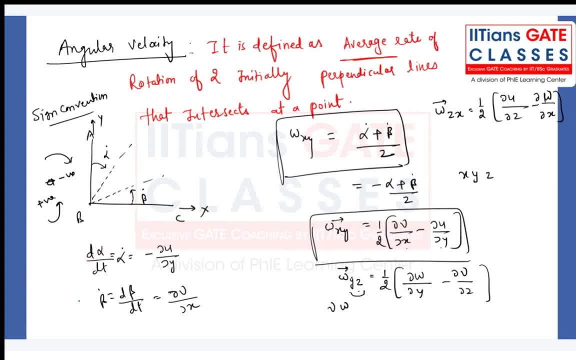 Just like in the boundary layer region, you have both rotation as well as shear deformations rate. Both are happening. Tell me in which case the shear deformation will be zero, but you have the rotation. And tell me one more case where you have angular velocity zero, but you have pure shear deformations. 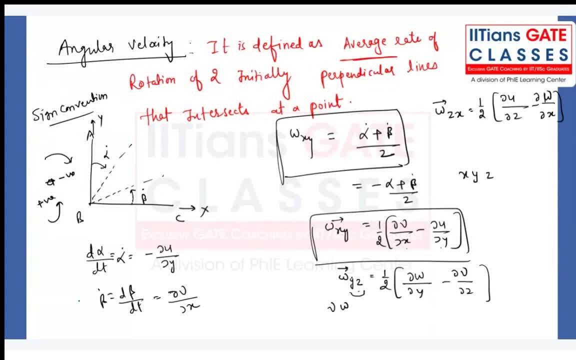 That is, you have no rotation but shear deformations are there? These two cases we have to discuss. Once it is done, let me know This. omega xy. we can also write: See, this is the xy plane, This is the xy plane. 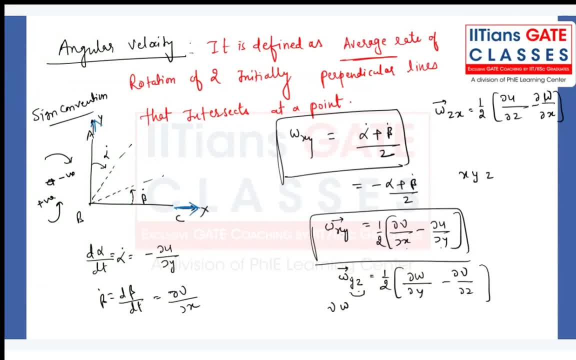 We are rotating about which axis? We are rotating about this perpendicular axis, z axis. Perpendicular axis z axis. So this is my omega z- Sometime they can write like this- And my dear friend, omega xy means, which is the perpendicular plane z. 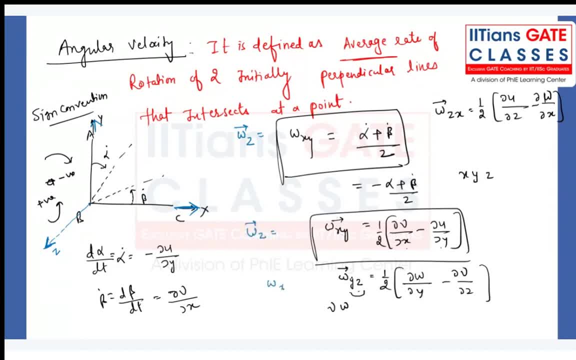 This is the perpendicular plane about what X. So sometime we used to write total angular velocity vector to be omega x, i cap. omega y, j cap. omega z, k cap. Okay, Okay, Make a note of it. Very, very, very, very, very important. 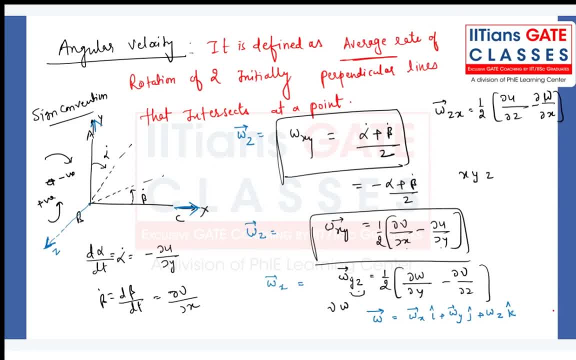 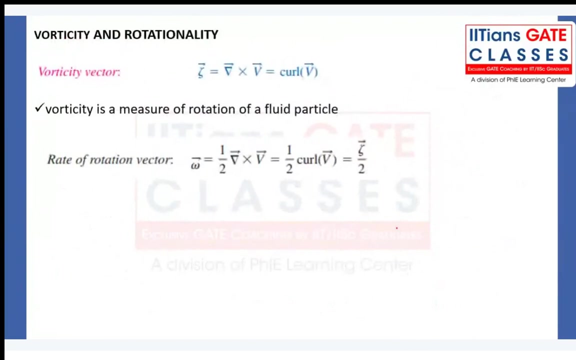 Is it done? All of you have noted down. Can I move to the next one? Okay, Okay, All right. Now try understanding the next particular concept about the vorticity and rotationality. Now, what is vorticity and rotationality? 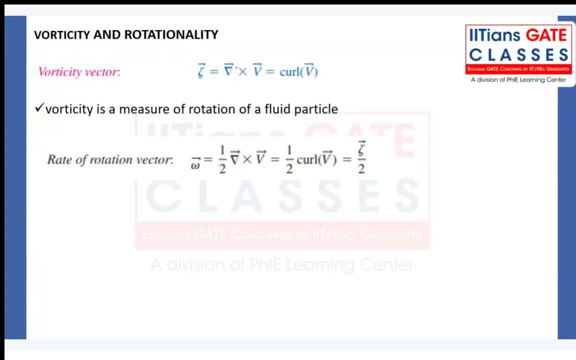 Vorticity. that can be written as delta cross v or curl of v. we say So, vorticity, my dear friend, we can also write. What is it if we can also write two times of angular velocity? Or angular velocity can be written as half of delta cross V, half of curl of V, right? 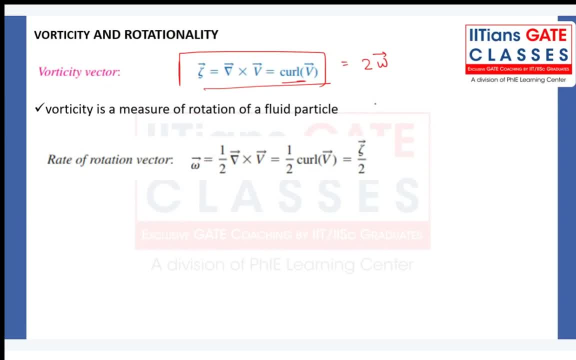 Because when you do half of curl of V, you will be getting the same thing. What is the delta cross? V I cap J, cap K, cap I cap dou by dou X, dou by dou Y, dou by dou Z, U, V, omega. 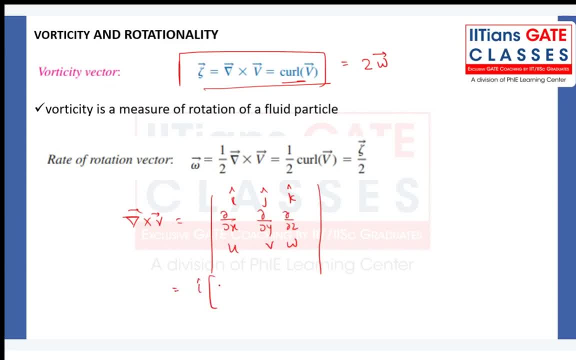 So when you write I cap that is dou V by dou X minus dou U by dou Y. When you write dou omega by dou X minus dou U by dou Z plus K, cap Dou U. sorry, You will be writing dou V by dou X minus dou U by dou Y. 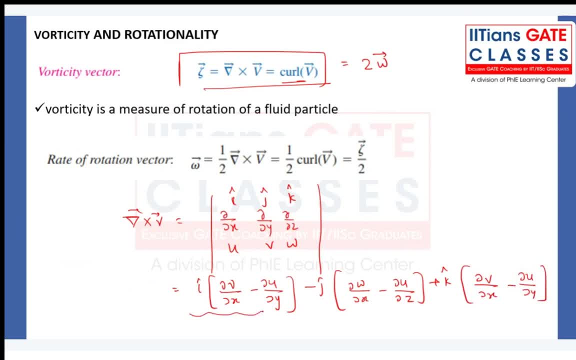 And what you are getting by different. This is nothing but vorticity. sometimes we also represent like this: So vorticity about XY And vorticity about XZ, This is the vorticity in XY. So when you just take the minus sign here, you will be writing like this: 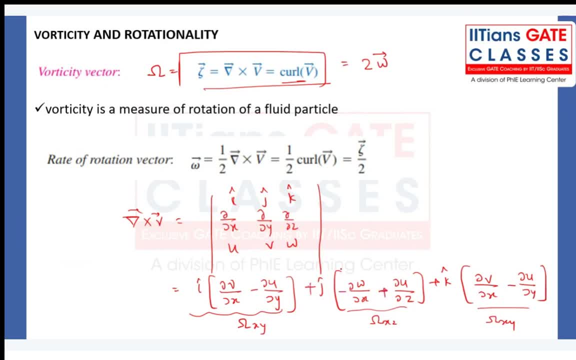 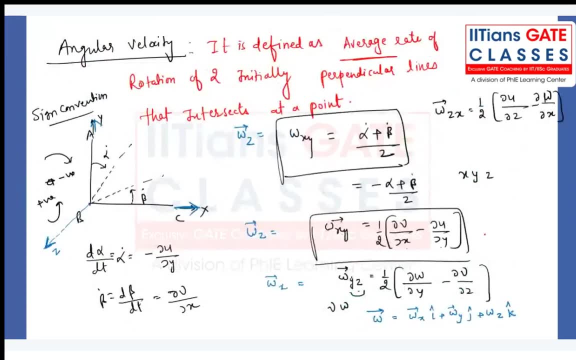 Same expression, See check it out: Dou U. by where is that? See check it out This one: Dou U by dou Z minus dou omega by dou X. When you multiply With the two, you will be getting like this: 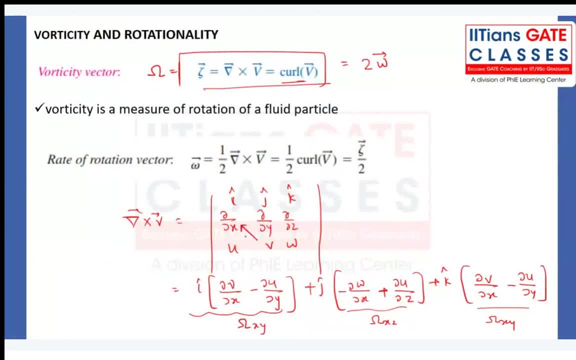 Always in a matrix, we have to multiply like this: First minus second, Plus, minus, plus, Plus, minus, plus. Then you multiply this by dou Y, by dou X minus dou K, And this is solving this equation. So really the next piece we are going to start from here. 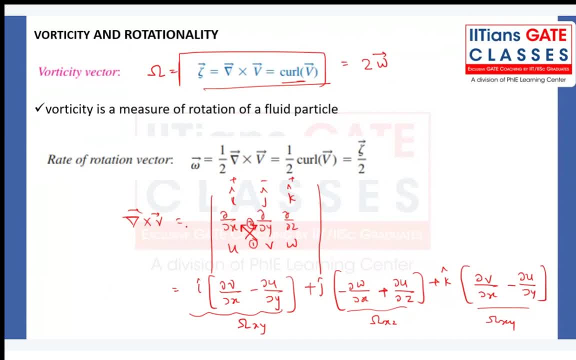 It will just be the下, And this will be our last cube plus, And this is our first equation, And the last one is going to be our last. So now our last one becomes the second, And this is the second. 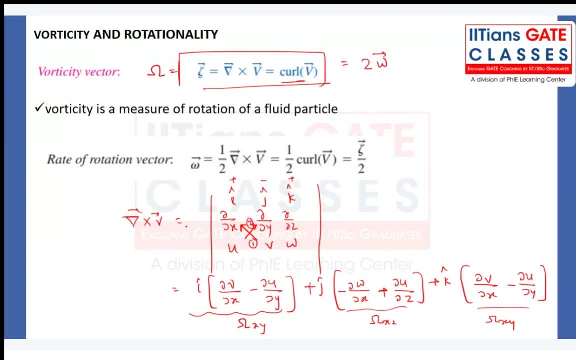 We are going to pick this one up and we are going to pick our last, So we are going to bring the last one. in Time is going to be the last one, So we are going to see the next one And this will be the last two. 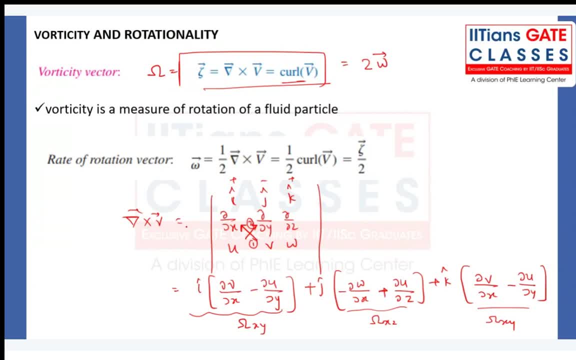 Thank you. What is? it is a measure of rotation of the particles. That means my different what you can write. if Omega is equal to zero- and what is it is also zero- Then it is an irrotational flow field. irrotational flow field which is being not rotating. 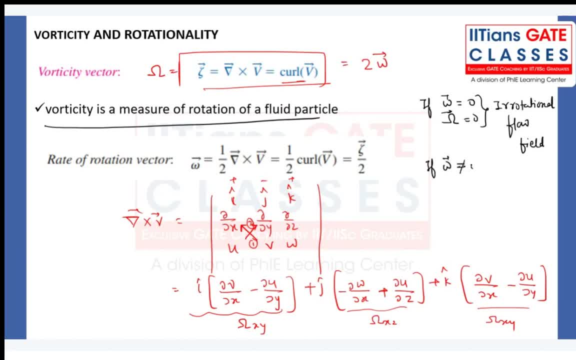 If Omega is not equal to zero, What is? it is also not equal to zero. We say this to be rotational flow field. rotational flow field. Make a note of it. And what is the vector will be X, Y. sorry, What is the about? 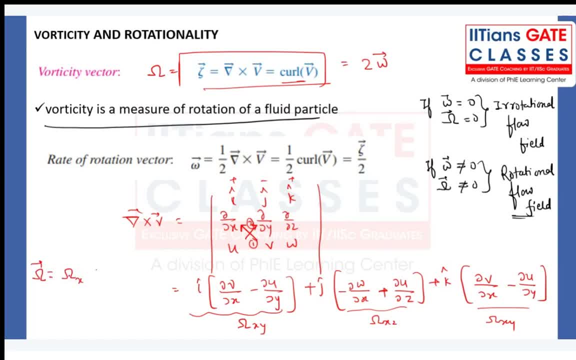 X. I will explain. I will explain. See, when the fluid element is not been able to rotate, that is a irrotational flow field, right, Just like outside the stream, outside the boundary layer, What we have, What you have, my different way. you have the fluid. suppose this is the flat plate and 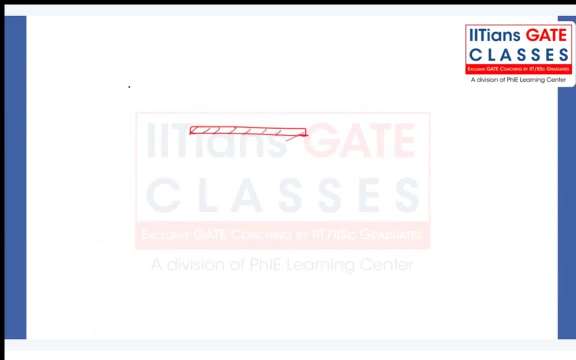 you have the fluid particle which is being traveling. You have a very thin region Where You have the velocity gradient which is being exist. Right Here we have 0.99 times of U, infinity free stream velocity. So what will happen? 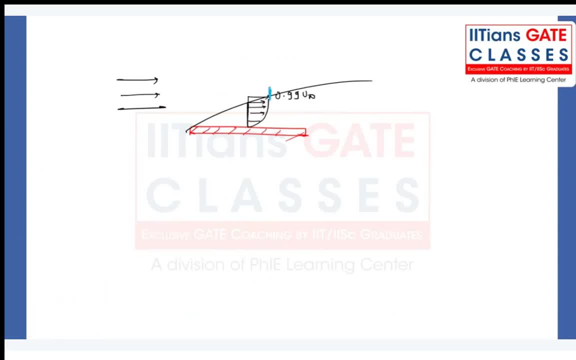 Here you have the slope: almost zero. dou u by dou y is zero. Dou u by dou y is zero. We cannot be there because that cannot be penetrated right. This is a one dimensional flow, So we automatically zero. So dou u by dou x will also be zero. 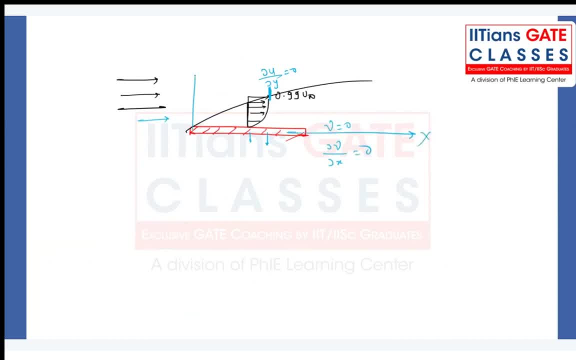 So in this X Y plane, Right Outside the boundary layer, You calculate what is it? Your omega in X Y plane or omega about that access? You just calculate What are the formula we have. We have the form of dou u by dou x, minus dou u by dou y. 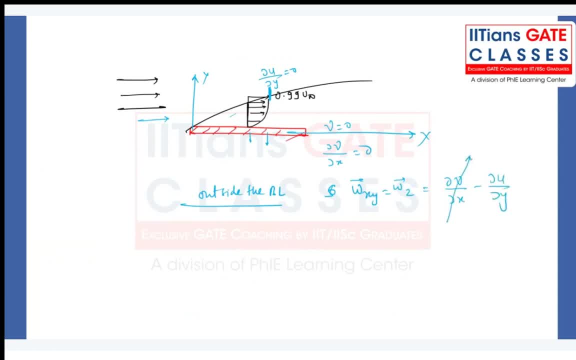 This is automatically zero. This is also zero. This is zero. So fluid particle will not be able to rotate. It will be flowing like this: only Here fluid particle will able to rotate. Getting my point? because we have the dou u by dou y. 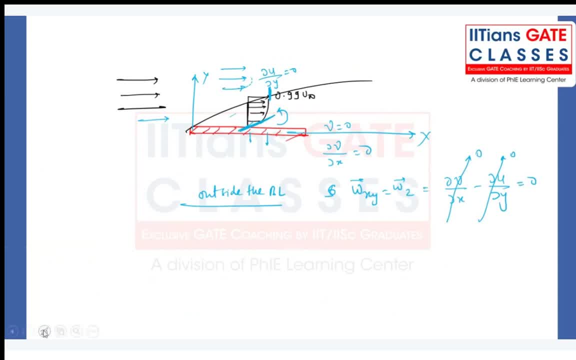 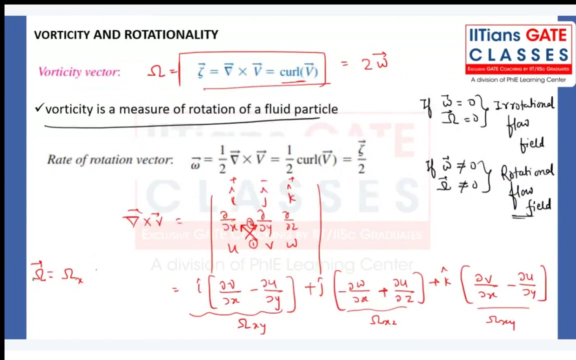 is that clear? so here we have irrotational flow field, here we have rotational flow field. once it is done, let me know: is it done? done which one? which one? i need to repeat? sorry, here there is a, no, y, z. something is missing. x, y is there. 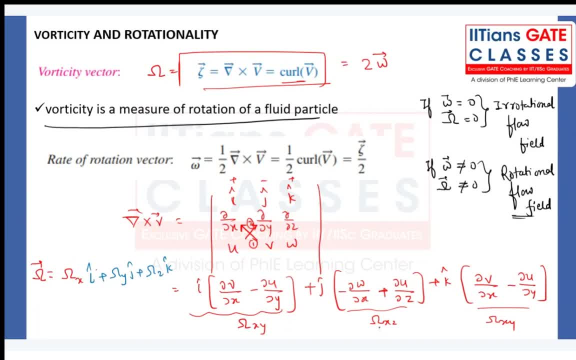 there should be some y. z should also be there, right, dou omega. this is dou omega. make a correction. this is dou omega, right, so this is nothing. but you have what? what you not. x, y, this is you have. this is v. so this is nothing. but sorry, sorry, i have written completely wrong. 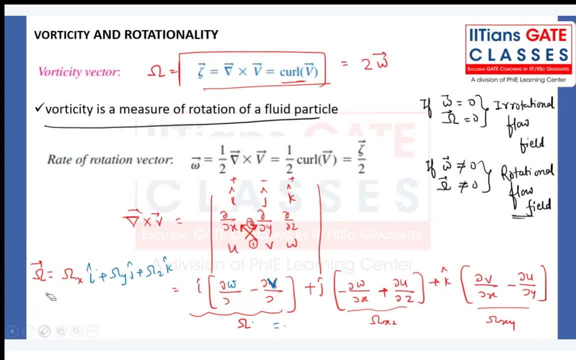 this has to be corrected because i cap is there right? so this is dou omega y, dou omega y, and this has to be z y, z or omega x. cap make correction. remaining things are correct. it is same as rotation. there is a no past history, it is just like a. 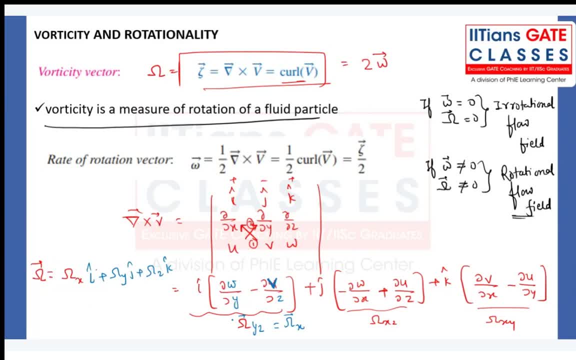 see, see, i told you, just like you know, when we discussed the some equations: whenever in the equation, whenever the terms are coming frequently, you know, frequently terms are coming while writing the equation 2 omega right, always it is coming together. this 2 m term is coming always. 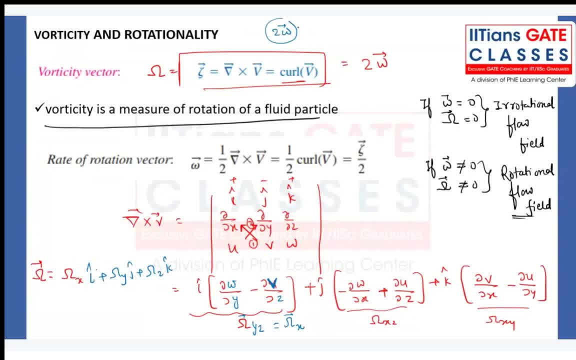 all the time. so instead of telling 2 m separately, they used to introduce one word called vorticity vector. right apart from that, there is a no significance, right, as we discussed about the kinematic viscosity, as well as we have discussed about the dynamic viscosity. there also, what is 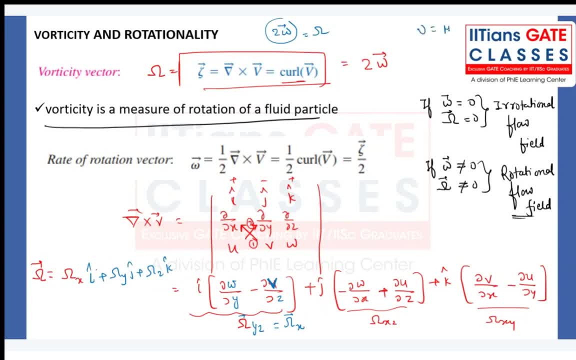 happening. mu is equal to mu by rho right. so upper term is viscous force, bottom term is inertia force. how much of contentment of uh energy is there? that is rho right, that is our inertia term and we call viscous term is nothing but how much it can diffuse to any layer. so with respect to that, 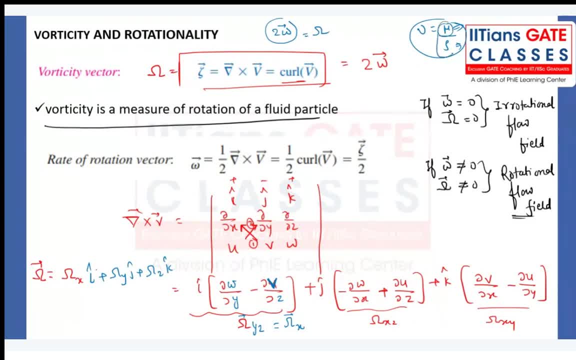 these terms are coming frequently: mu by rho, mu by rho. so they introduce one more term, relative term, kinematic viscosity. so similarly in the equation it was coming to omega to omega all the time. so they replaced by one term called uh, what we call vorticity, right? 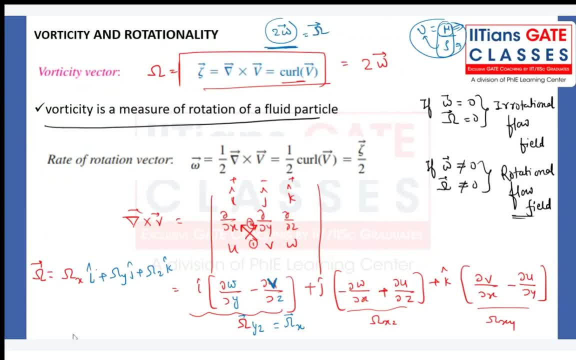 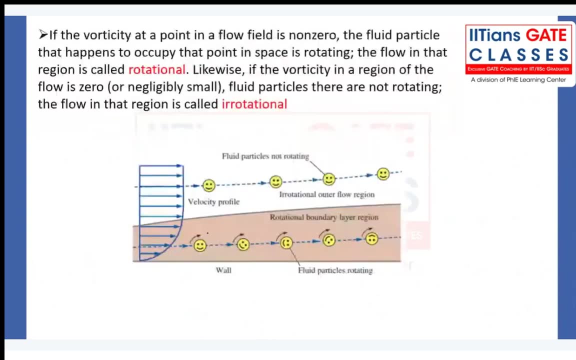 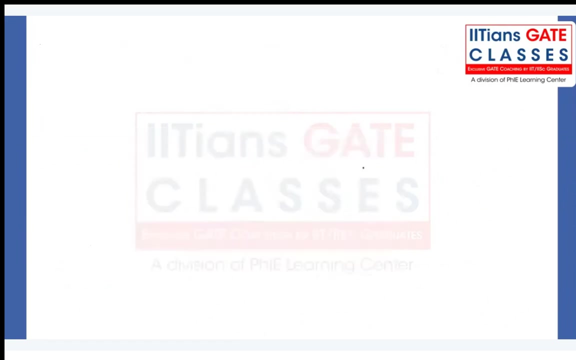 now try to solve the numerical. as you can see inside the boundary layer, what we have inside the boundary layer, the fluid particles has been rotating, so that is a rotating or rotational boundary layer region. outside it is being straight. it is not rotating right now. try to solve this. 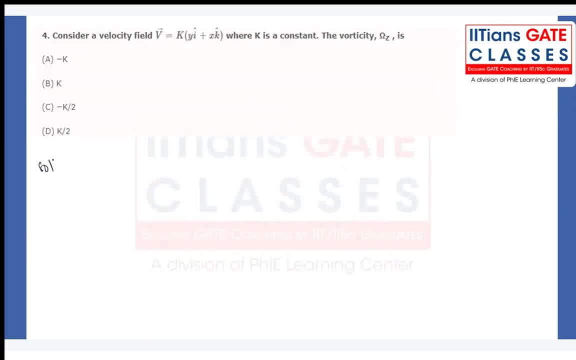 particular question. the velocity field has been given u as ky, v is given as kx. they are asking what is the vorticity z? that means they are asking vorticity about z axis in xy plane. that means x will be there, y will be there. 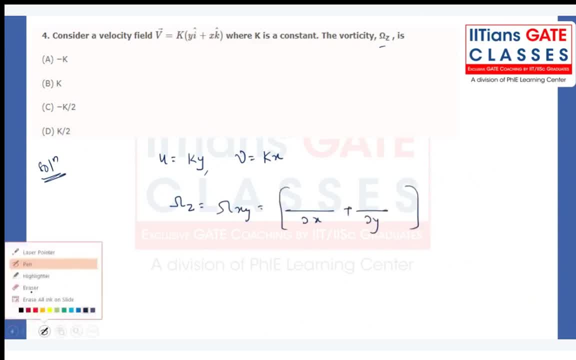 and minus sign will be there, x is there, so u, uh, you will not be there. v will be there and something like this. so what we can write: dou u by dou x is k. dou u by dou y is once again k, so that is coming as zero. 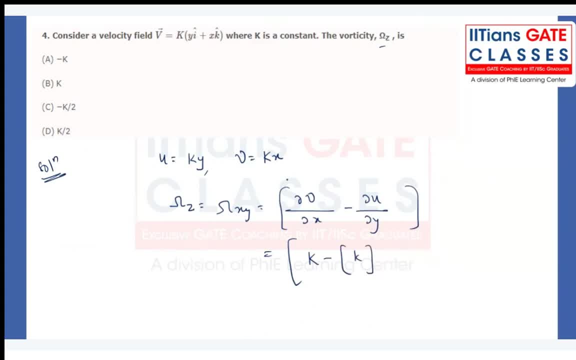 now, what is that here? sorry, sorry, this is not v. omega is given, right, u i cap plus v, j cap plus omega, k cap, omega. they have given as kx. so there is a notice that here v is given. all that is equal to v dot. i didn't know. so that's right. so there is coming a zero here for vale and then this is coming as zero. no, what is that here for the? this is SprSS. negative is r? this is negative. so that's why this is omega right here. sorry, sorry, this is not v. uh, I scopf. so that's why they have given us kx. so that's okay. when we know u, that is coming as negative, not v. 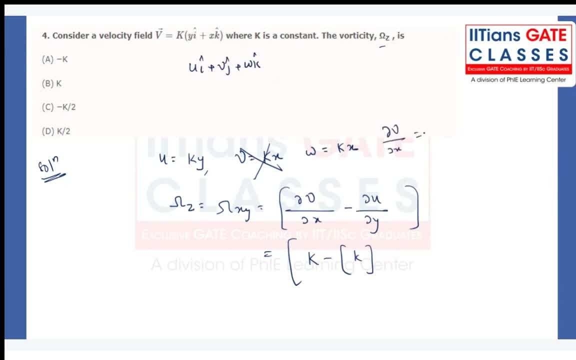 know dou v by dou x, that is 0. this is 0 big 0. so minus k, that is a is correct, so make a note of it. once it is done, we can leave for the day and i will upload the slide. many problems are there. you please try to go through that. you now? thank you.